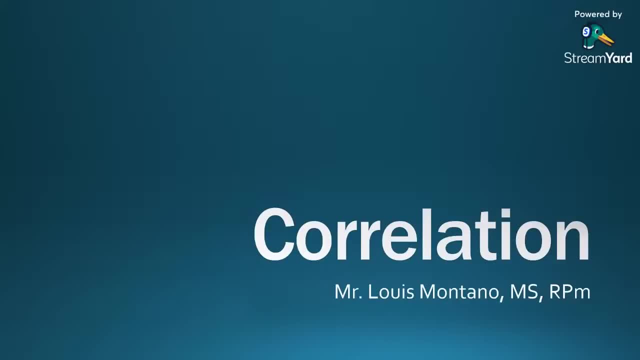 We will start in a minute. Can you hear me? Sorry my sounds, It's been a while since I did. I'll turn off my cam in a minute, Pero can you hear me? Dinig niyo ba ako. before we officially begin. 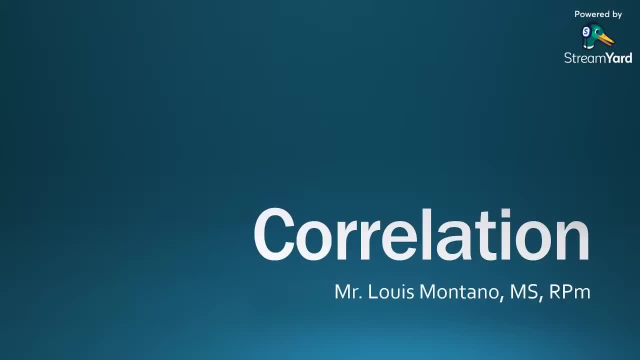 Yes, po. Okay, that's good. Alright, sige, hintayin lang natin yung iba. Okay, it's 8 o'clock, so let me turn on my camera. Hello, hello everybody. Magandang gabi po. Welcome to our live stream. 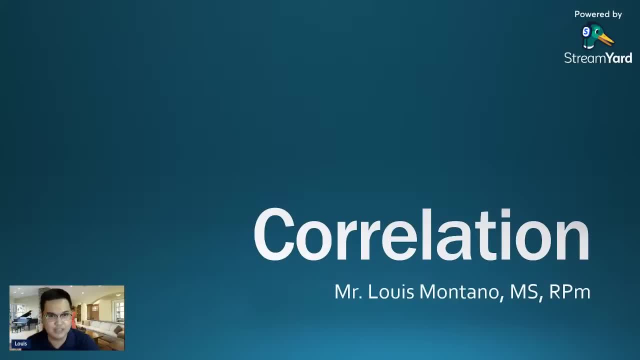 Welcome to our online lecture about correlation and regression analysis. Thank you very much for attending this lecture. I really appreciate it. sa lahat ng mga nag-share, I really appreciate the help of our PM2IT people, particularly our geostudents, And thank you to everybody who helped in disseminating na meron tayong online lecture tonight. 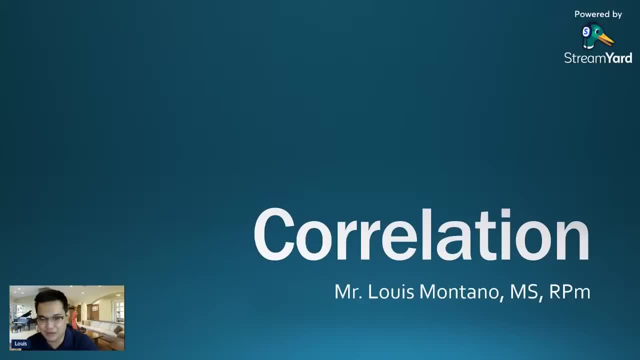 Ayan, So good evening everybody. Pinifigure out ko pa kung paano akong makikita dito sa StreamYard yung, ano, no, Ah, okay. okay, Nakita ko na Ito pala yung. Ah. okay, There you go. 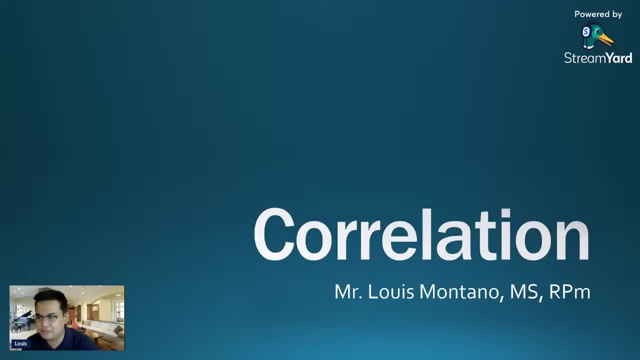 It's been some time since I did live stream on StreamYard, Kaya medyo naninibago pa ako. Okay, Zoom, diba O sino ba sa inyo yung mga naging students ko. no, Naging students ba ko pa kayo sa review. 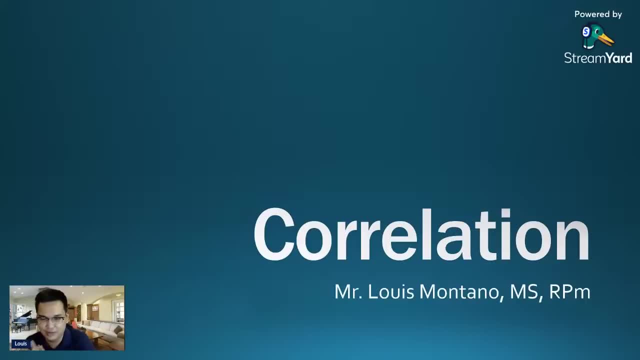 Okay, Saan kayo Sa home base ba kayo, Or nag-meet ba tayo face-to-face. Anong branch ba ang nare-representa ninyo? Okay, Ayan, Gusto ko makita kung mga taga saan ba kayo no. 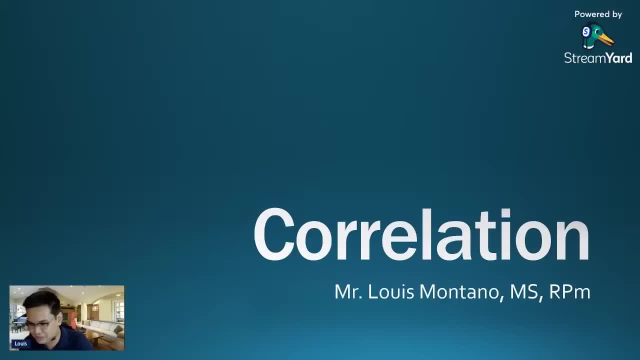 Home base. Ayan, Ah ayan Face-to-face. Kung face-to-face saan sa Manila, Okay Ayan Ayan Nandiyan ka pala Luning-ning sa mga followers ko. no, So hello, hello, no. 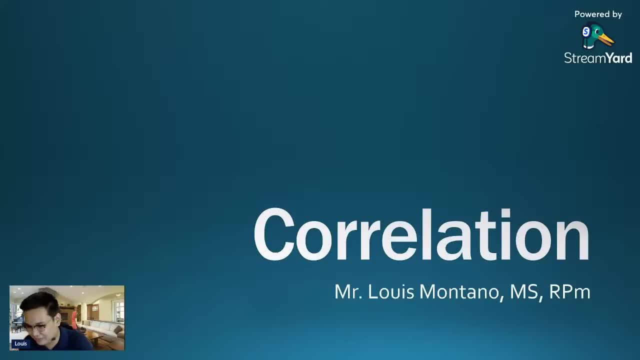 Ayan Cebu branch. Oh, hello, No, Mayong gabi Face-to-face Saan yung face-to-face No, Hello, you no, Nandiyan ka pala, Okay, Ayan, Ayan. 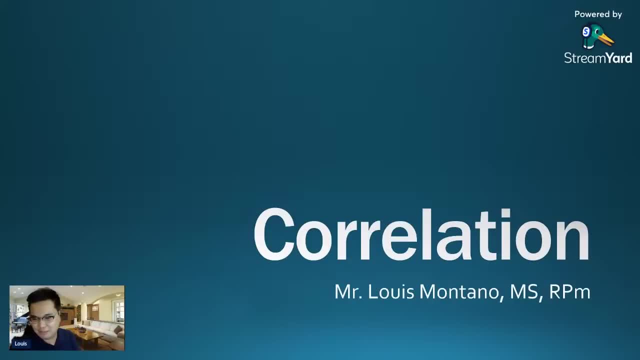 Ayan Nandiyan si Grecian former students ko. Salamat sa pagpunta. Oh, corona da It's been some time. no Kailan ba ako pumunta d'yon, Ano pa yun. 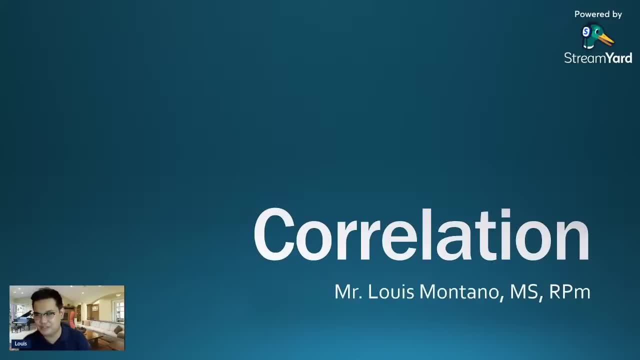 February: RGO Baguio. Wala akong Baguio this year, no, Pero um I'm happy. no, I think magkikita-kita tayo this Saturday online Ayan. Okay. So you no, Yung, pangano mo ba in real life, Anna Forger. 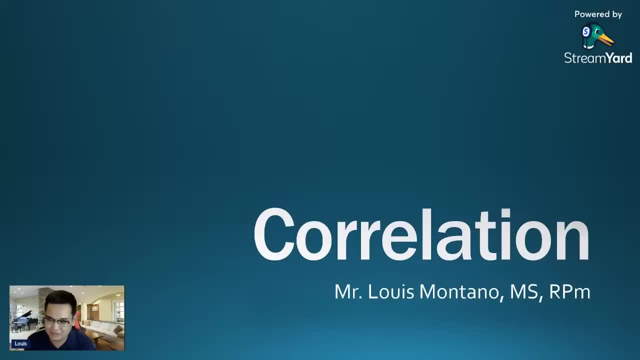 Okay, Double, yeah, Wala kayo double this year. no, Pero I believe magkikita-kita tayo online. no Sa Saturday. Um, I'll let you know ahead of time. no, Sinabi na. eh. eh. eh, hindi ko alam. no, Alam nyo na ba. no, May dev cycle ako sa Saturday. no Sa ano sa booster. 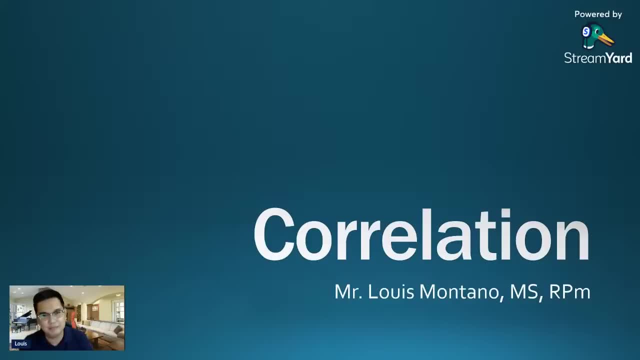 How do you call it? Is it booster? I forgot ano yung term ni Mam May: Competency review. no, Competency review. Yeah, So ayun Amuntin lupa represents. Ayan, Okay, Alright, Sige. 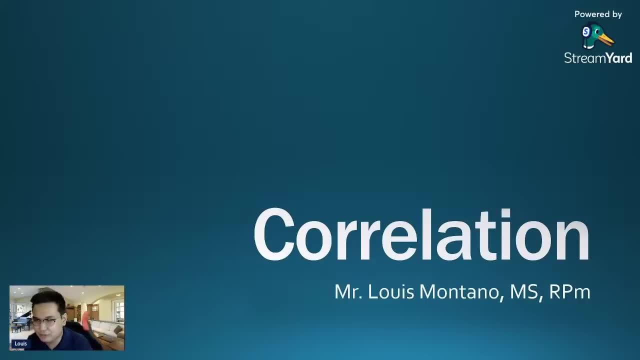 No, Siyempre no Para sa inyo to no Okay And marami-rami, Oh, 100,. no, I didn't expect it na ganito. karami ang pupunta. no, So sa mga kararating lang. good evening everybody. 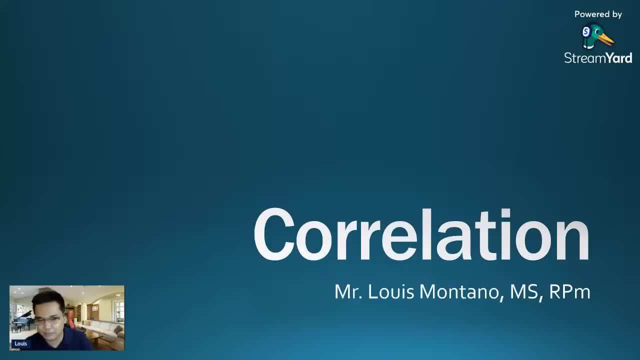 And welcome to- okay, welcome to- our lecture tonight. Um, let's start tayo with some sort of kamustahan, because I know that it's been some time na rin since we ended with our face-to-face review And now we are moving back to online. no, And it's so happy to be in touch with ano. no, 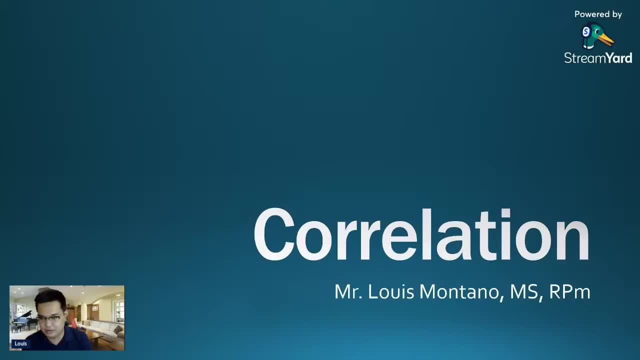 With you once again. no, Kung online man or face-to-face. yung last na last time na nakita tayo. Okay, It's nice to see you again. It's nice that you're doing well At malapit ang board exam. no, 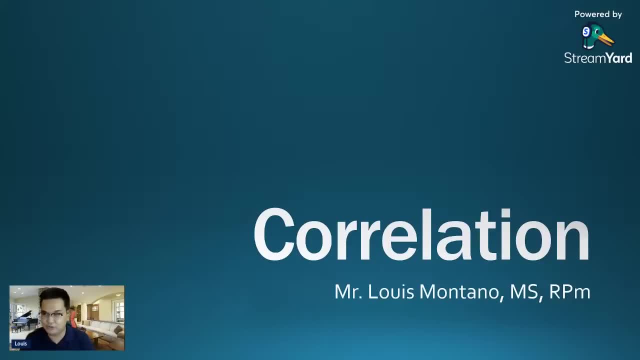 Kung bibilangin nyo ang araw or hindi. it depends on your personality, whether or not you are neurotic, Okay, So nasa inyo na yan, Okay, Anyways. Um sige, no, Let's begin, kasi medyo marami akong ito cover tonight. 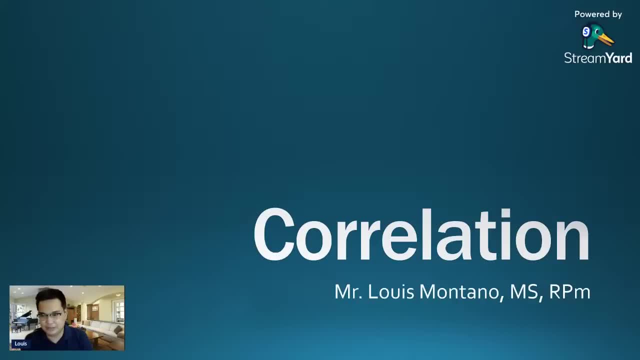 I teach stats in school, by the way, And sa totoo lang, na iba yung gusto ko i-discuss tonight, iba yung nasa isip ko, Pero since it's been some time since I did online through StreamYard, gusto ko munang kapain. 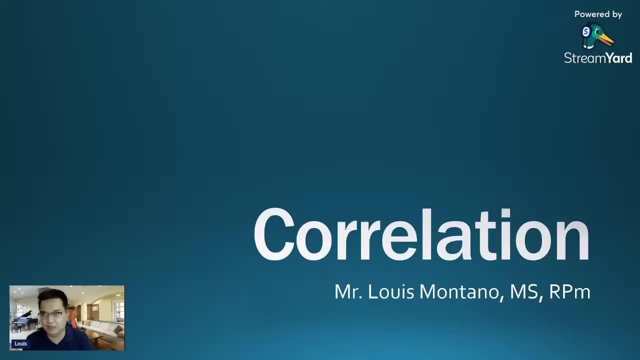 Okay, Kasi baka maputol-putol ako online tapos pumangit yung outcome. Pero originally my plan was to cover Yung mga analysis. kasi Karamihan sa mga students ko sa face-to-face man or home-based- usually say: 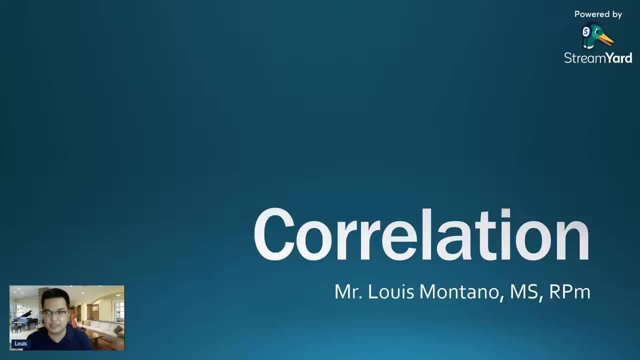 Sir, di namin naranasan yung test-dev, kasi nga online kami ng to-site assessment sadly Okay. Um, pero sabi ko next time ko na lang siya gagawin. Okay, Because I'd like to test the waters first. 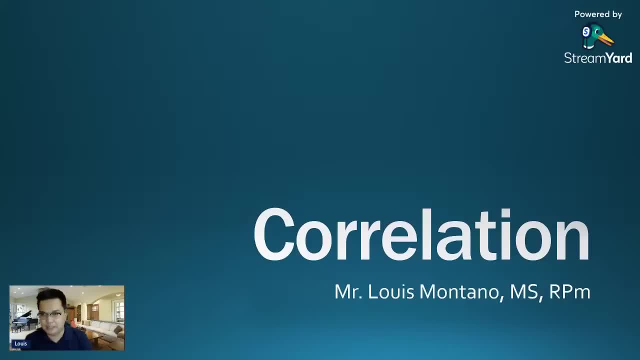 Baka kasi mag-epic fail yung live stream. So why not start with an easier topic: correlation and regression. It may be easy for me, but maybe not for some, no. So I'd like to share what I know about this. 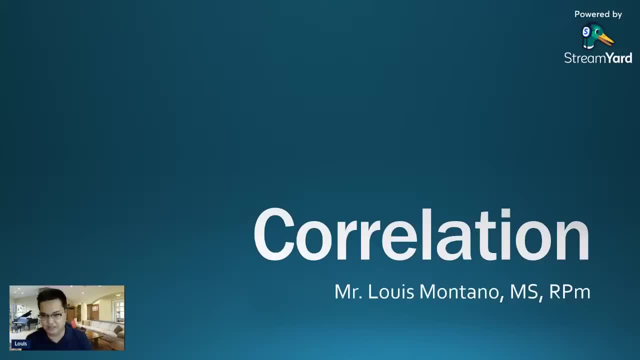 And then later on we will be moving to regression analysis, Yan. So kung nahirapan kayo sa stats, no, I hope you will learn a lot tonight. My approach is simplified. Bakit Kasi hindi ako magaling masyado sa math? 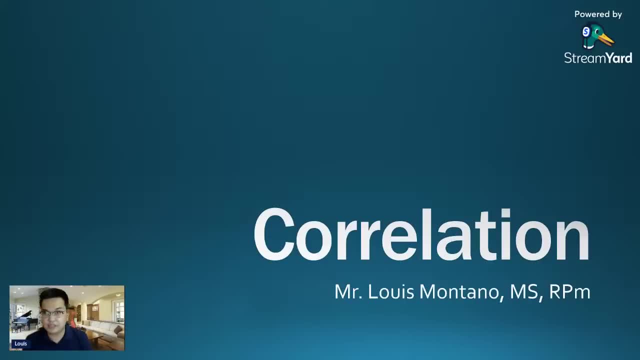 I'm an average student, Pero since we use computers okay in stats, doon ako naging confident Okay Tapos I'm proud that My approach is simplified, At least according to my students, And I hope that will also work for you. 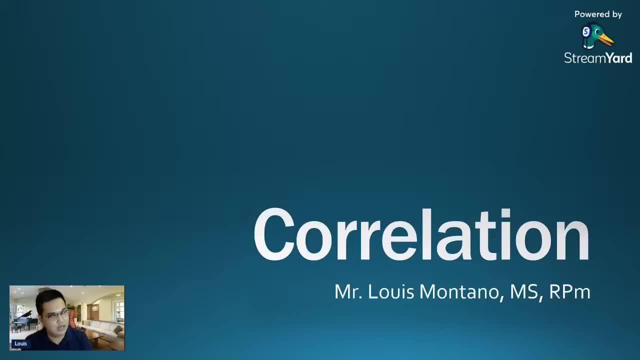 In terms of my experience, I've been teaching stats since 2020.. Okay, Aside from the review class And other than that, I've been a thesis mentor since 2020 rin. So yun yung experience ko. no. 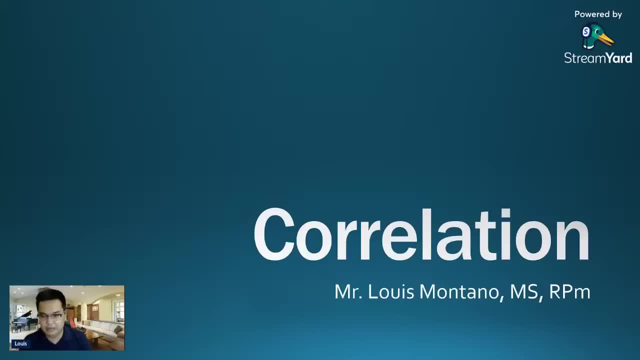 I usually teach And other than that, I also teach, like assessment And the rationale. okay, The rationale why I want to discuss this tonight is Bilang psychometration or if we have listeners here na non-psych students no. 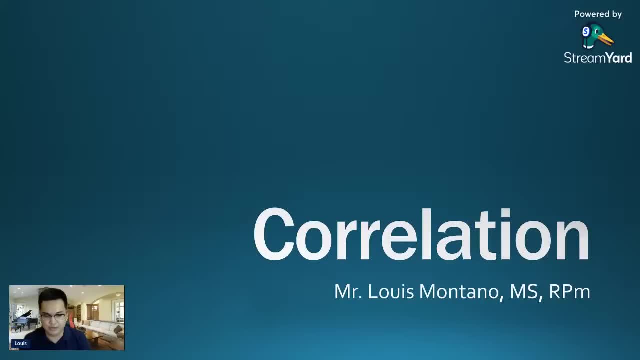 Pero most of you are going to take the boards for psychometration Bilang psychometration correlation should be your friend. It dapat friend mo siya. hindi mo siya kaaway. Tsaka dapat naiintindihan mo siya. 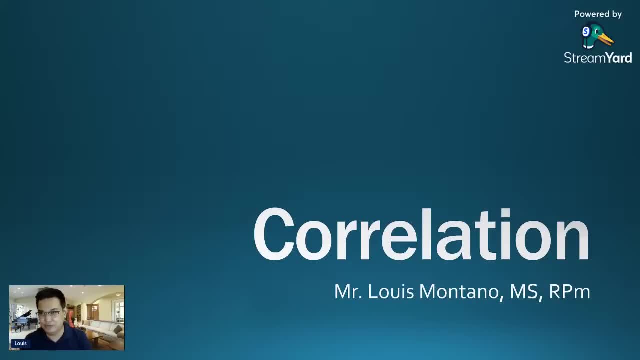 Okay, Kaya yun. yung objective natin tonight is ayun no, To review the concepts of correlation and regression analysis, which is very much related to correlation At pangalawa. okay, The reason why I chose correlation: kasi kapag gets mo siya, it's easier for you to understand all other topics. 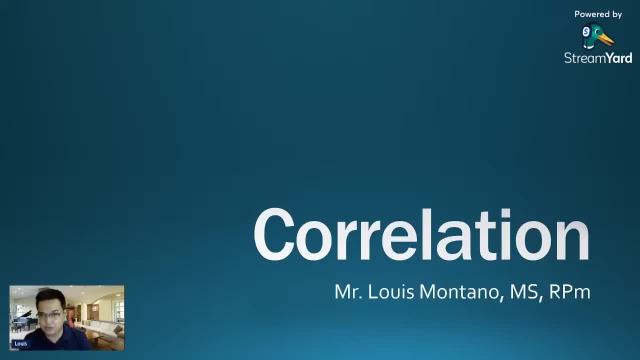 And not really all other topics, but the other topics in what you study. Okay, Like psych assessment, particularly Because in psych assessment, when you analyze reliability, validity, when you create a new test, you rely heavily on correlation analysis. So let's start with correlation analysis. 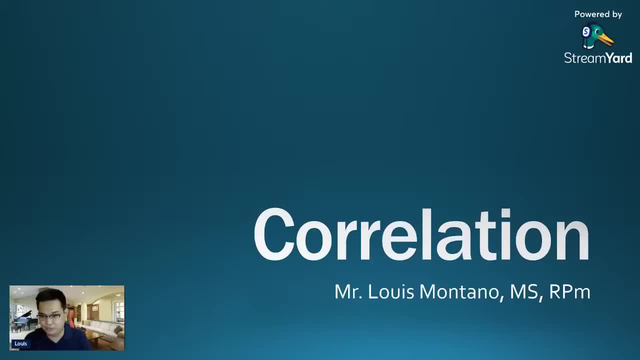 And then, right after this, we move on to regression. So let's first talk about the basic concepts, Okay, But before that, no. Did you do correlation when you were? ano, no, When you were in school, Like maybe thesis or whatever? no, 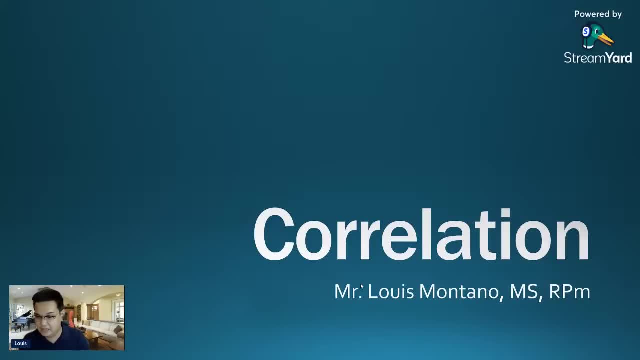 Sino dito yung mga nakaranas mag-correlation analysis? I'd like to know no, Or hindi nyo ba siya nagawa? no, when you were studying? I'd like to know no, Kung kung if you have a question you can ask me. 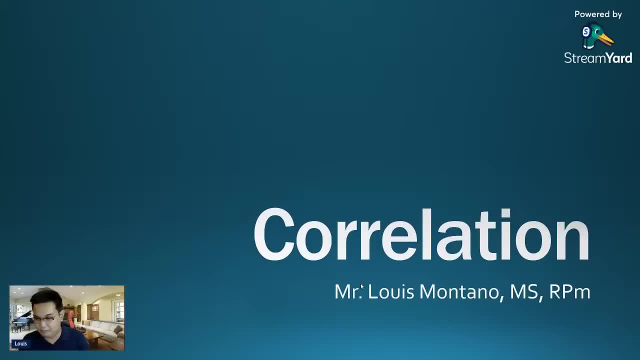 If you have a question, you can ask me. If you have a question, you can ask me If you have a prior experience in doing this or wala pa no? Were you able to run correlation when you were writing your thesis? no, 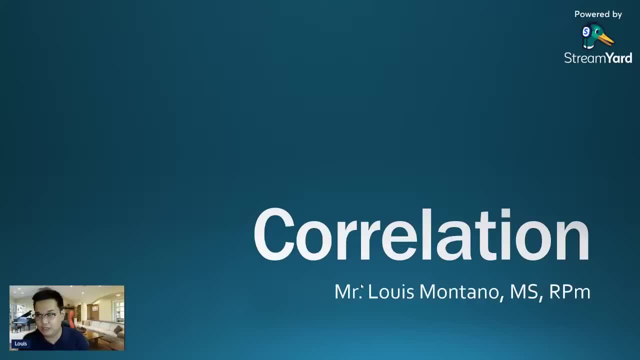 Siyempre, kung kuwanti highly likely no, Pero kung kuwanti, then I doubt no Mababang-mababa yung chance na na-correlation kayo. no. Okay, Thesis po yan very good, no. 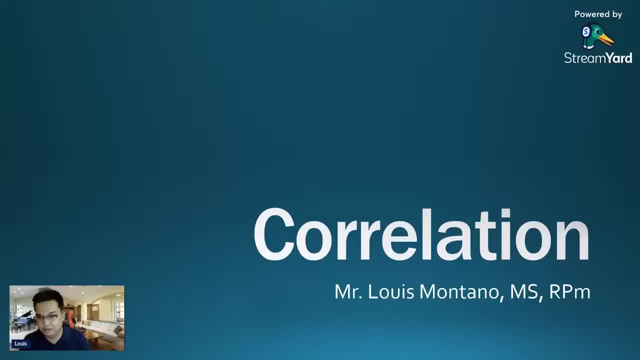 Kung sa thesis kahit pa paano Sa extants, no, that's good. no Thesis or even senior high, pa yan di ba that counts Okay Sa mga medyo siguro nahihiya yung iba to answer no. 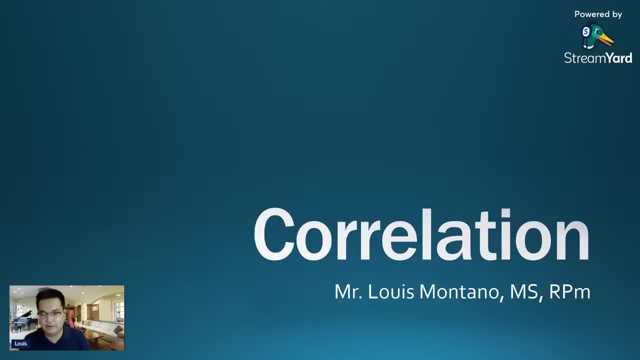 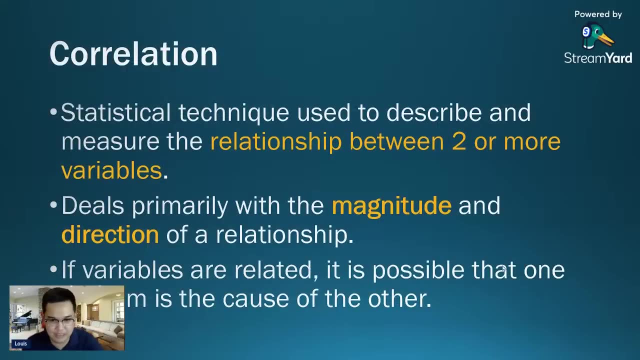 Kasi alam ba't di ko yan naranasan. no, Okay lang yan. no, Kaya nga we're having this session tonight. Okay, Sige, Simulan na natin. no, So what is correlation? Let me transfer yung camera po. 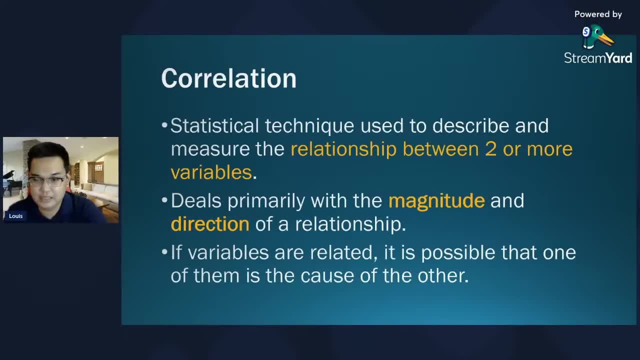 Yan. So when we say correlation, it's a statistical technique used to describe and measure the relationship between two or more variables. So hihighlight ko yung phrase na two or more variables, because what I want to correlation, no, let me just highlight this: correlation: no sino yan, ano yan sino yan. tatawa ka dito no. 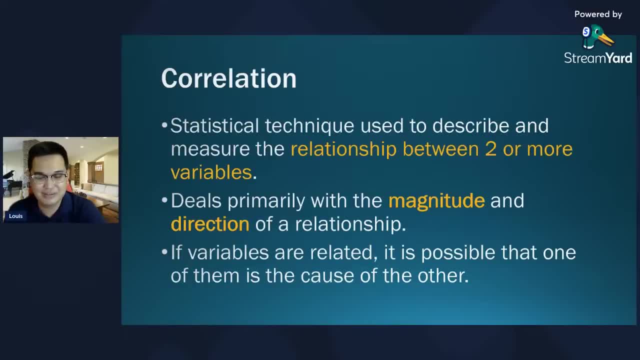 Anyway. so going back: no, so when we do correlation, no, tingnan natin no relationship between two or more variables. no, it means kapag magkakorrelate ka kunyari sa word exam. 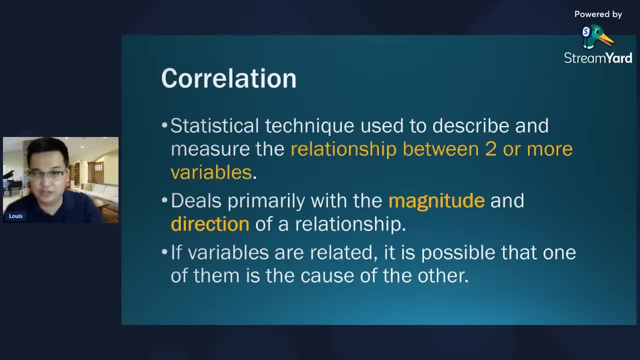 sabihin sa inyo: oh, ito yung sitwasyon, tapos piliin nyo: ano yung statistical treatment Kung isa lang yung variable? definitely hindi yan correlation. Kasi paano magkakaroon ng relationship kung isa lang? 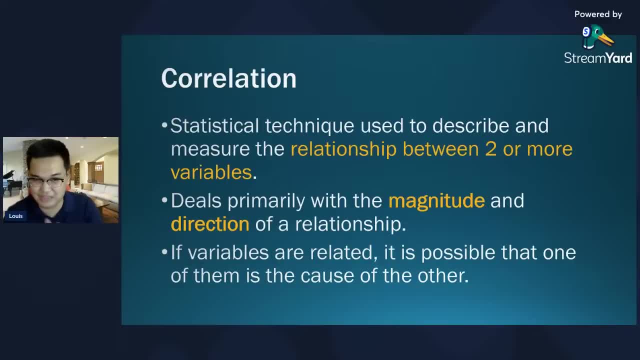 Diba sa relationship dapat dalawa. no, May it be stats or tunay na buhay. no, Sa stats dapat dalawa or more. It's hard, okay, It's hard Ang hirap, isipin ng correlation kung isa lang yung variable. 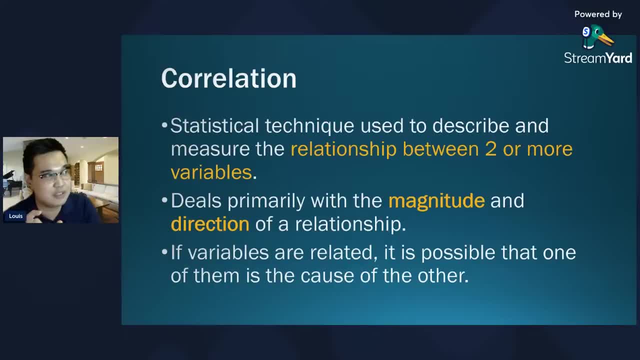 Except na lang. except, if we're talking about test construction, tapos iko-correlate mo yung mga items sa isa't isa. well, isang tabi muna natin yan for now. Okay, Ngayon let's talk about research, not really in the context of test development. 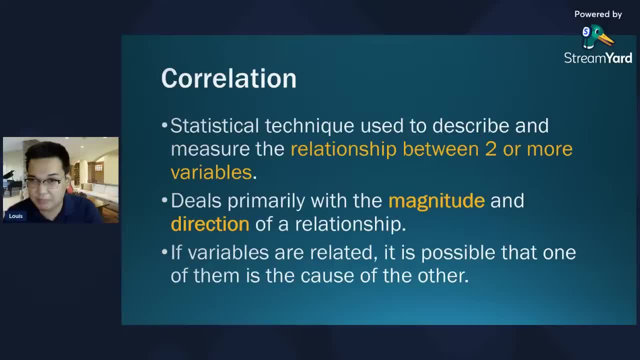 Maybe that's for next time Sa research. kung dalawa yung variable mo malamang sa malamang magkakorrelation ka? Kung isa lang hindi, yan correlation. Maybe other treatments but not correlation analysis. 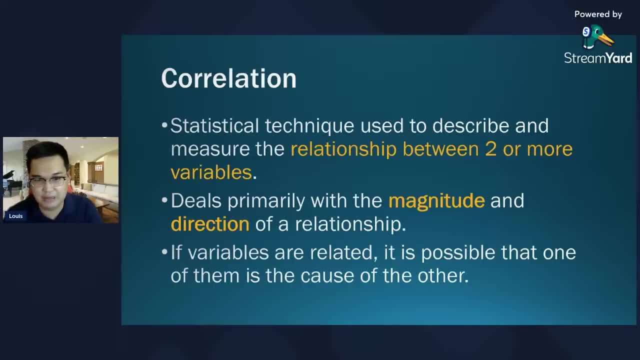 Okay. So, for example, no, Gusto mong malaman. no, Gusto mong malaman. For example, ito yung approachable exam. Gusto mong malaman ng researcher kung may relationship ba yung parenting sa dev psych, yung parenting with aggression, among kids. 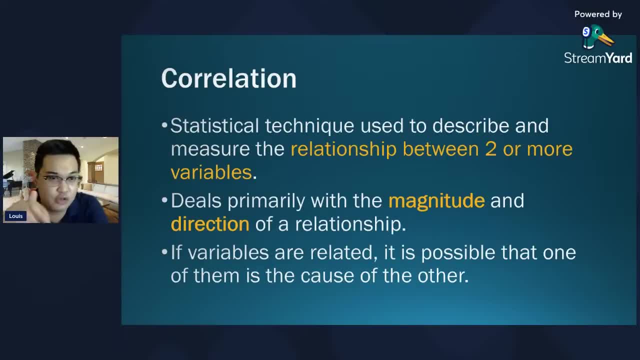 Yun bang mga parents, yun bang mga kinalakihan nila authoritarian parenting, do they become more aggressive? So to answer that dalawa yung variable mo- parenting okay and aggression- And to determine kung may relationship sila you run correlation. 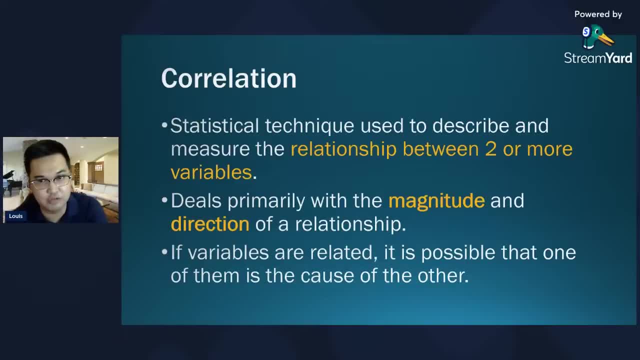 So the word that should come into your mind when we talk about correlation is kinalaman May kinalaman ba. And to answer that, kung may kinalaman ba, you run correlation, You correlate, You look at the relationship. 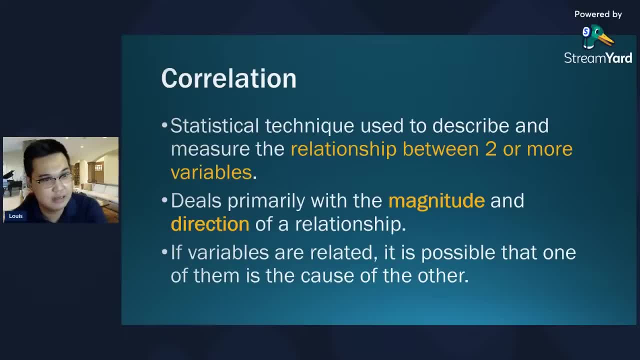 So may kinalaman ba ang happiness sa, for example, job satisfaction. Yun ba mga masayang empleyado, satisfied din ba sila sa trabaho nila. Okay, So kung gusto natin malaman kung may kinalaman, we can run correlation. 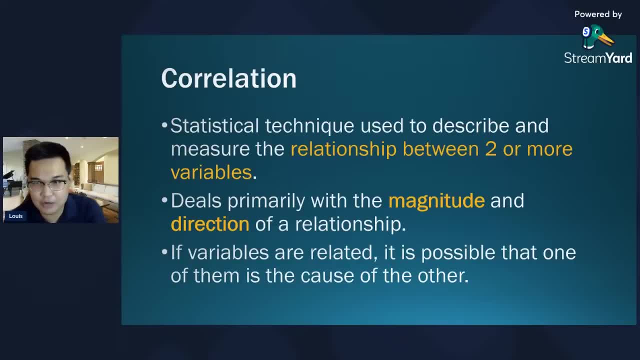 So that's the first thing, Pangalawa, when we talk about correlation. it provides us to data or to information which are highlighted on screen: The magnitude, okay, of the relationship. we also call this strength and the direction of relationship. 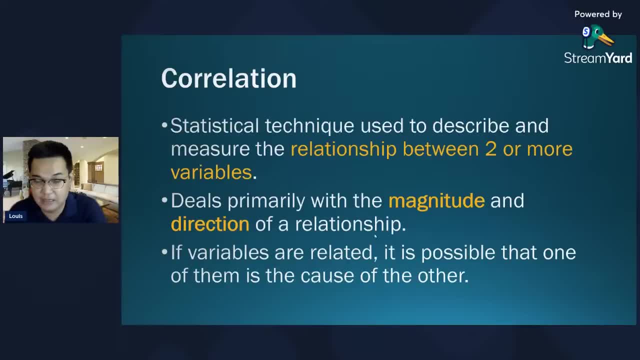 These are two important information provided by the correlation analysis Titingnan natin yan in the next few slides, And one more reason as to why we study correlation, kasi if two variables are related, it is possible that one of them may be the cause of the other. yet we do not claim cause and effect. 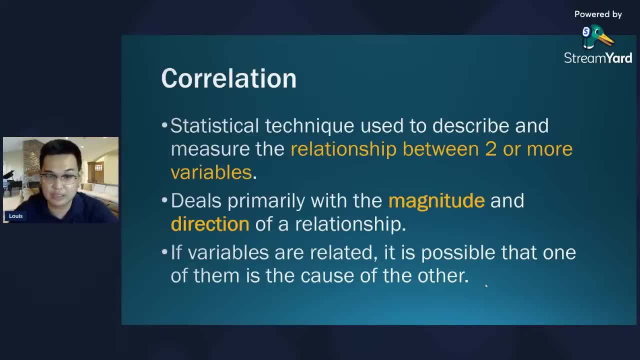 We will go back to this later. kung bakit we do not claim cause and effect. Pero possible that if related sila, then possibly may cause and effect relationship sila, Pero bakit hindi natin kiniklaim yun? 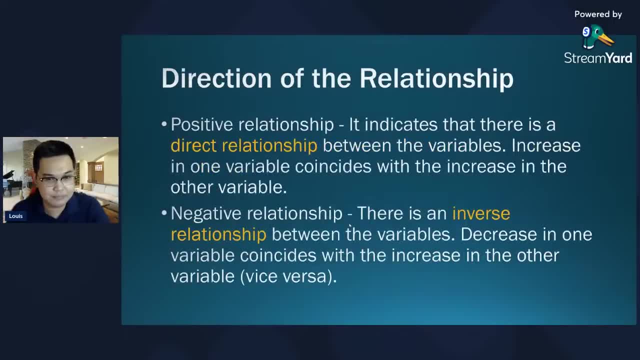 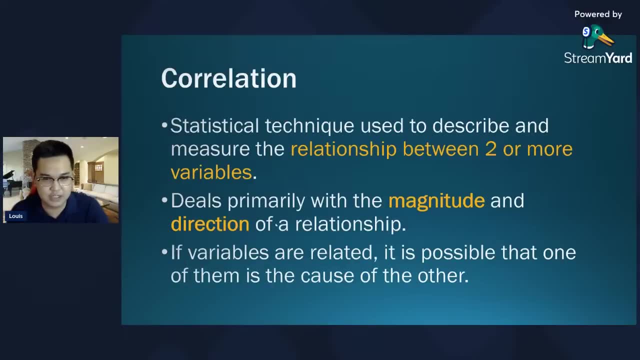 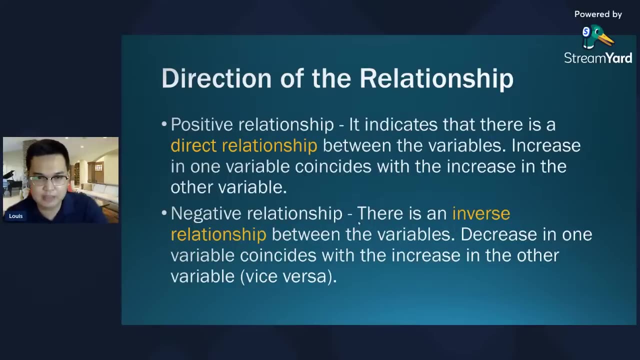 That's for later. For now, let's talk about sabi ko kanina. correlation provides us to information, the strength or the magnitude, and the direction of relationship. Let's start with the direction of relationship. So when we talk about direction, always remember dalawa yan. 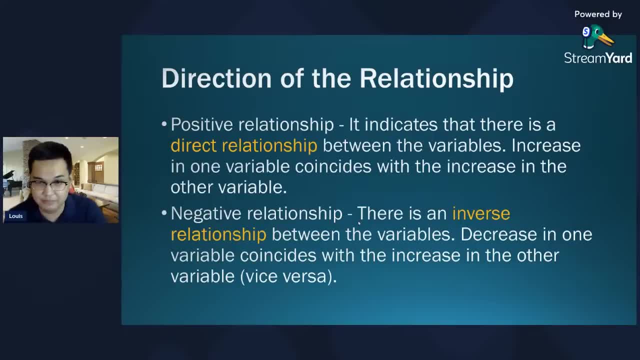 A relationship can be positive or negative. In a positive relationship, okay, As one variable increases, the other increases as well. Kung tumataas yung isa, tataas din yung isa. As X increases, Y increases as well. 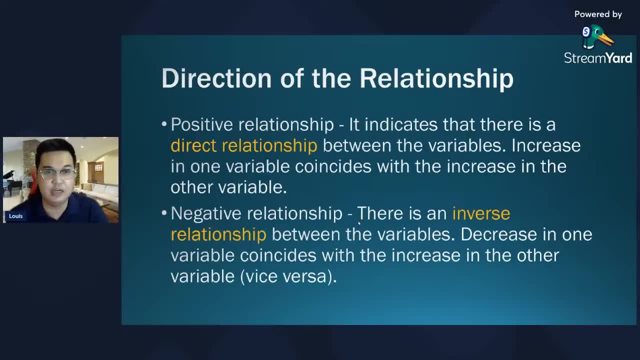 That's the idea behind positive correlation, Also known as direct. Siguro, kung sa board exam gamitin yung term direct or sa research paper sabihing direct, it's a positive correlation. On the other hand, in a negative correlation, baliktad. 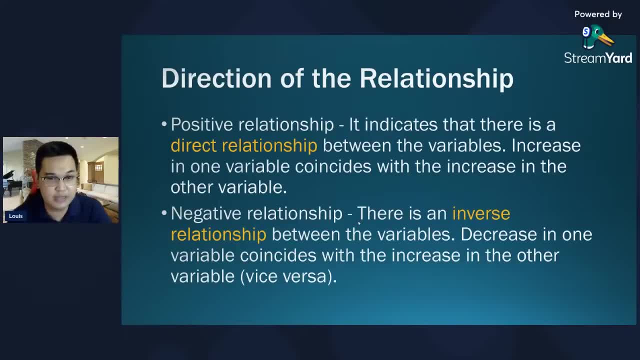 Habang tumataas yung isa, yung isang variable bumababa, So baliktad yung relationship nila. We call it inverse correlation, We don't call it indirect. Okay, we don't call it indirect. 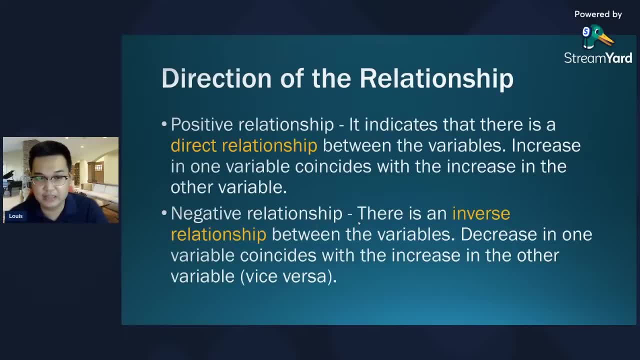 We call it inverse And yung word na negative hindi ibig sabihin pangit, It means inverse. Hindi siya pangit na correlation Just because yung pangalan niya negative, Hindi siya ganun. It means yung relationship nila inverse. 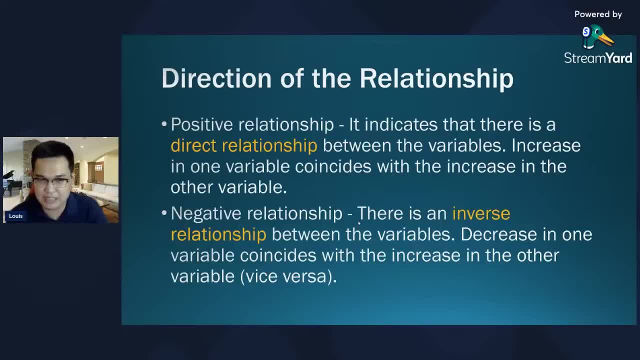 So what does that mean? Sige, balik tayo sa positive. Examples of positive relationship include: Sige gagawin kong board related, kasi karamihan sa inyong review isa board exam. Examples of positive relationship include: the higher the consensuousness, the higher the productivity. 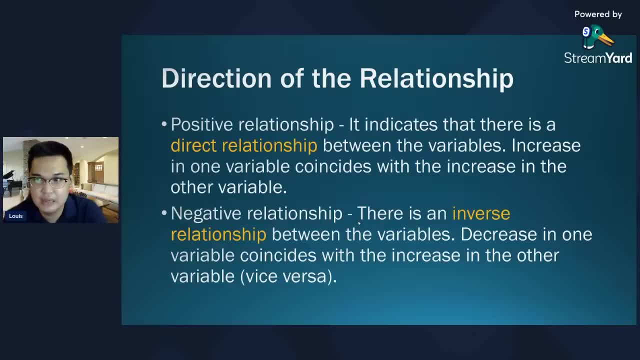 The higher the consensuousness, the higher the compliance with the law, The higher the consensuousness or gawin natin neuroticism. The higher the neuroticism, the higher the chances of developing depression or anxiety. 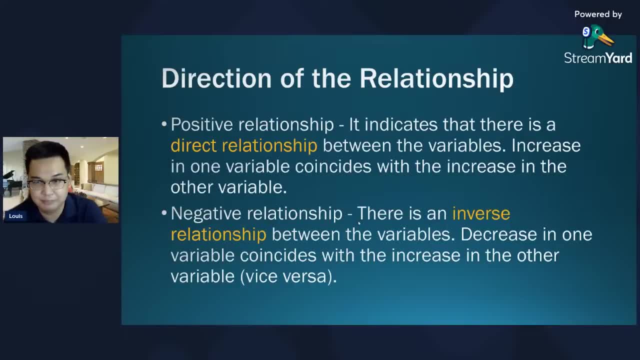 That's a positive relationship. Pag mataas yung neuroticism mo, mataas din yung chance na magkakaroon ka ng depression, magkakaroon ka ng anxiety. Okay, So parehang tumataas. 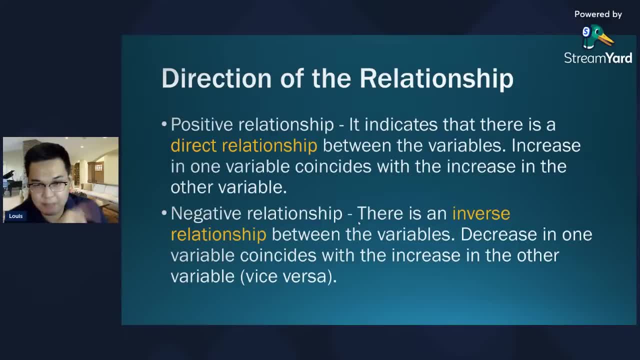 Whereas in a negative correlation or in an inverse correlation, pag mataas yung isa, bababa yung isa. For example, the higher the job satisfaction sa trabaho, the lower the intention to resign. Kasi masaya ka eh, So the more na masaya ka sa trabaho mo, sa IO, sabi ng IO. 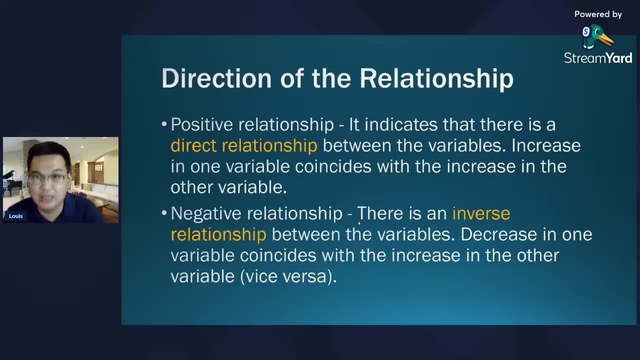 the lower the probability that you will resign. Okay, What else? The higher the neuroticism, the lower the life satisfaction. Mas neurotic ka, mas mababa yung life satisfaction mo. Kasi kapag neurotic ka more prone ka to psychological problems. 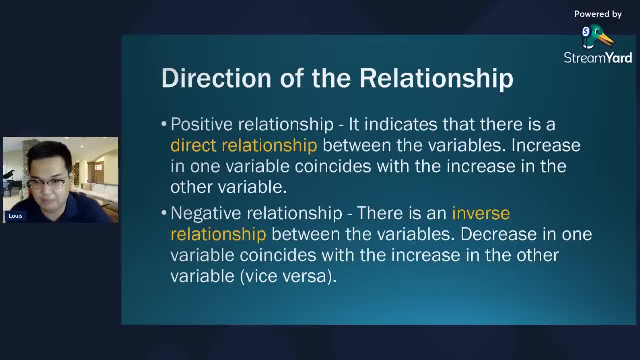 Very good, This is correct. Tama ito, Kapag inverse, as one goes up, the other goes down, Samantalang in a positive relationship, the variables move in the same direction. One last example is kunyari no. 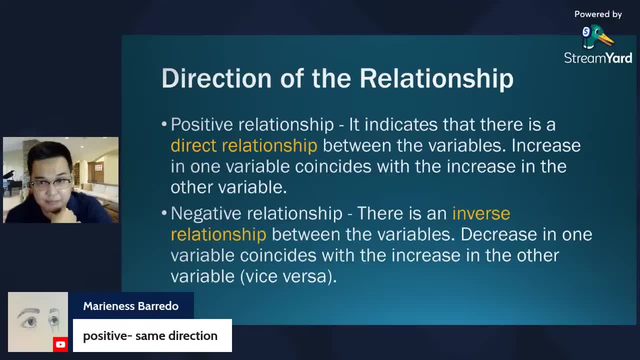 The higher your score in the entrance exam, the higher your grades are going to be in college. So ganun siya, Okay, Do you have questions about direction? By the way, meron pa supposedly pangatlo Yung pangatlo no relationship. 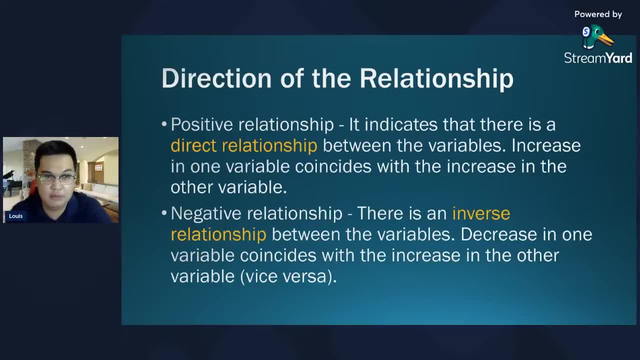 So kapag no relationship walang kinalaman sa isa't-isa, Okay. Hindi siya positive, hindi siya negative, Okay. Kapag no relationship walang kinalaman, For example, the relationship of English proficiency with the intention to say Mother Earth. 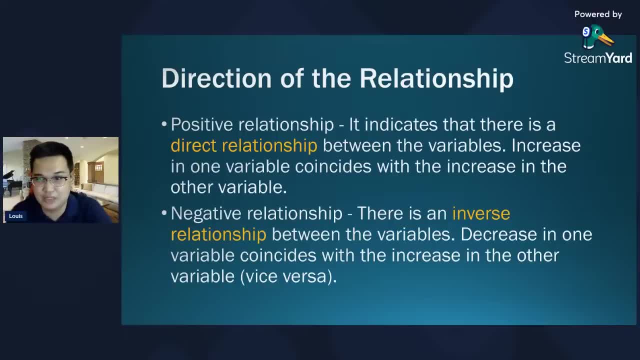 No, Parang ang layo ng variables na yun sa isa't-isa Diba. So in that case there will be no significant correlation. So that's for the direction. Okay Ngayon, ayan no. 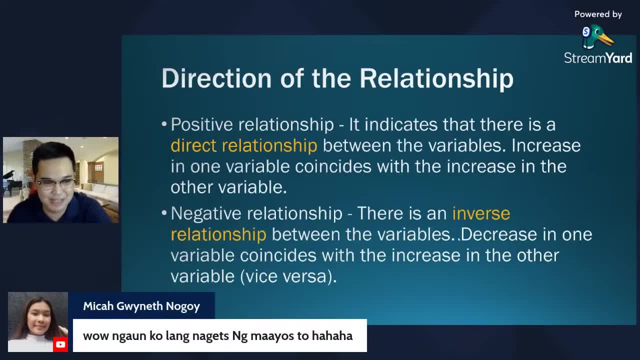 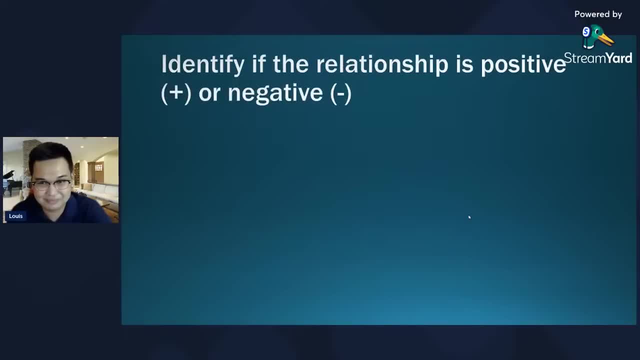 Nag-gets, daw niya. Salamat naman, Sana, mas mag-gets mo rin yung iba pang mga concepts na dadaanan natin. no, So that's for direction. Okay, Sorry, sorry, sorry. 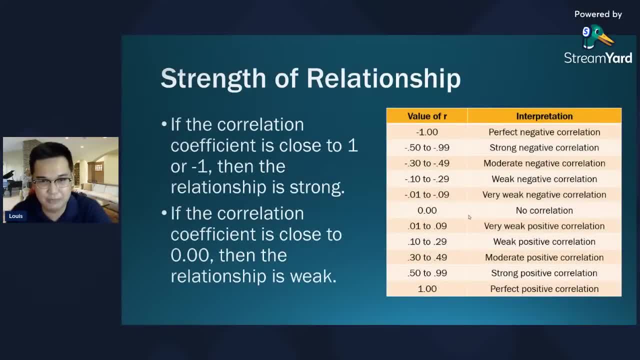 Ngayon naman, kung merong direction the relationship also has, you know, strength, Or we also call it magnitude, Ganon katatag yung relationship And the rule of thumb is if yung correlation coefficient o yung value. 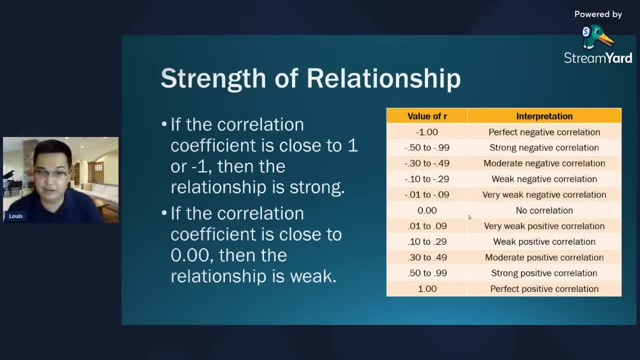 yun kasi yung tawag sa stats ay coefficient. yun yung tawag sa value. Okay, The closer it is to 1,, the stronger the relationship is Mas malapit sa 1,, stronger yung relationship. 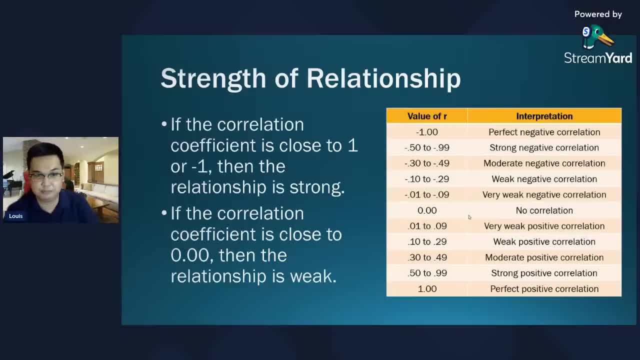 Mas malapit sa 0, mas mahina yung relationship. Okay Say, for example: so ito yung um yung interpretation na sinusunod ko. I listed it down sa right: no Sa mga nagtatanong. 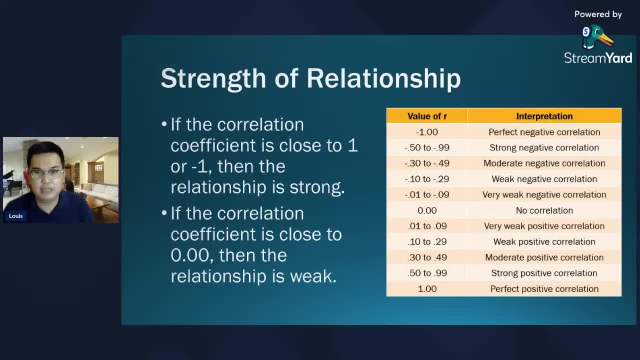 kasi usually may mga nagtatanong: Sir, saan niyo yung po nakuha yan? Kasi sa librong binabasa ko, iba naman po yung sabi: no, Ako sinusunod ko yung standards sa stats tsaka sa research. 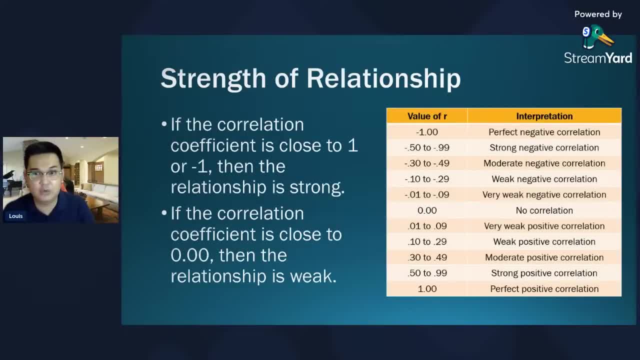 Eto ay based kay Cohen. I'm just not sure if the Cohen I'm talking about is the same Cohen as in the textbook. no, I think ibang Cohen ito, So I have to check on that. Anyway, hindi yung identity niyo, yung mahalaga, no. 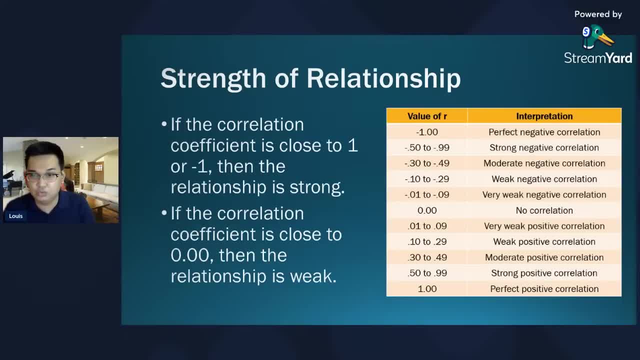 Um Cohen, 1992: interpretation of correlation coefficient. So kaya ito yung sinusunod ko, kasi ito yung standard. eh, Kung may susundin man yung mga libro no, or yung, for example, sa board exam. 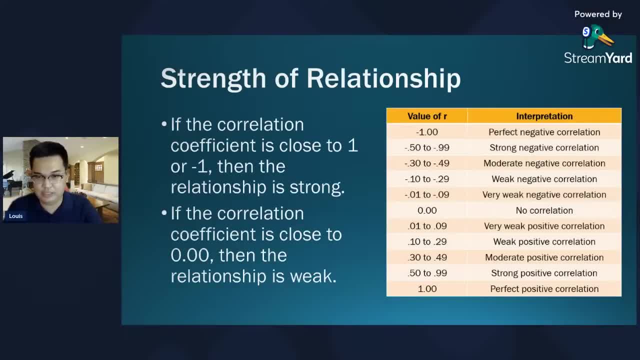 I think they will base it on Cohen 1992.. So ito siya: For example, kapag 0.00 yung value ng R na makukuha natin walang relationship yung variables Kapag um 0.01. 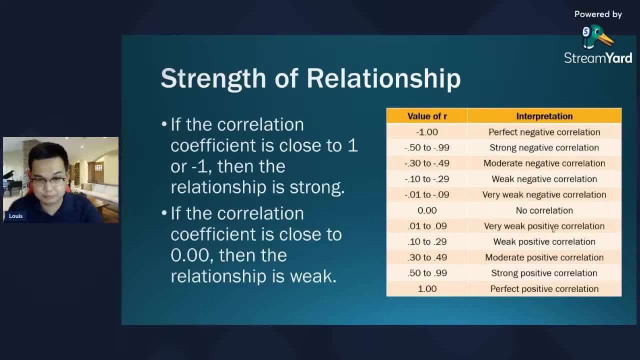 to 0.09, there's a very weak positive correlation. Kapag 0.10 to 0.29, there's a weak correlation 0.30 to 0.49,. moderate positive correlation 0.50 to 0.99 is a strong. 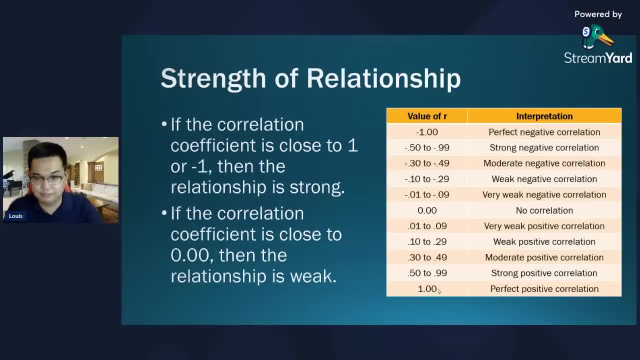 positive correlation And perfect 1 is perfect positive correlation, Hindi siya pwedeng lumagpas. If the correlation is, for example, 1.30, imposible na. yun Meaning hindi yung ano yun. 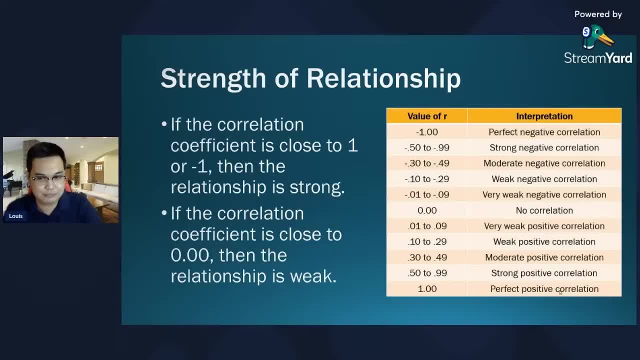 May mali sa computation. So that's really impossible. Ngayon, kung lalagyan natin ng negative symbol, negative sign. kapag walang negative sign, automatic positive relationship yan. Kapag may negative sign, yan yung negative correlation. So 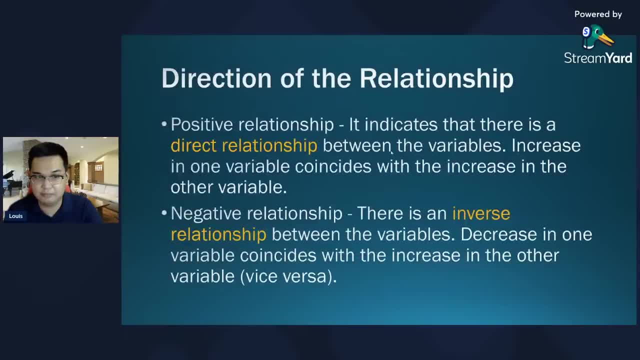 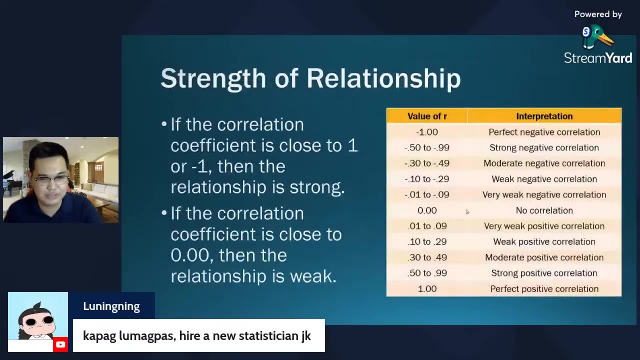 it will go back to your understanding of the direction of relationship. Tama yan luningning Kapag lumagpas, yan yung sagot. Mali nyo, yan talaga yung choice sa board exam: Hire a new statistician. 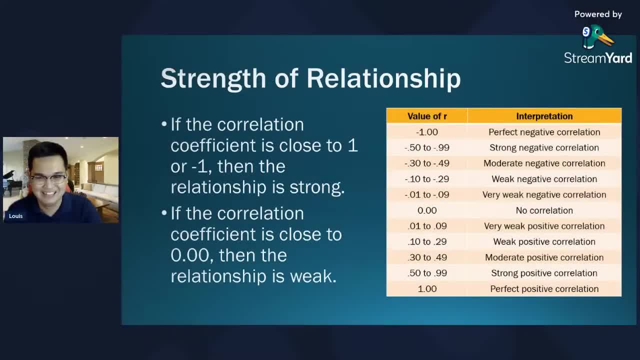 kasi imposibleng lumagpas, Okay, Anyway. so yan Baliktarin, Lagyan nyo lang ng negative symbol. Tapos, ito naman yung interpretation ng negative Pag negative 1, that's perfect. negative. 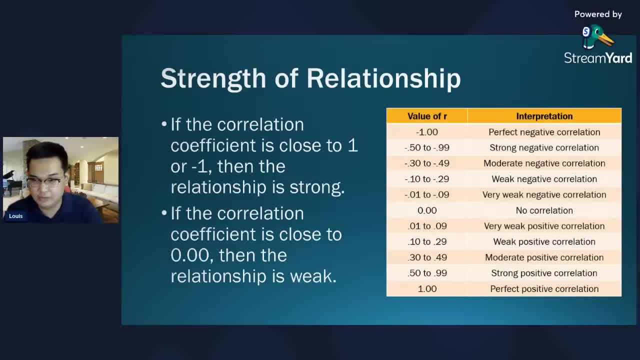 correlation and so on. So if you always look at this, if you base it on this chart, it will allow you to easily understand. Okay, What kind of relationship are we observing? And this correlation coefficient automatically gives you two data: Dalawa na. 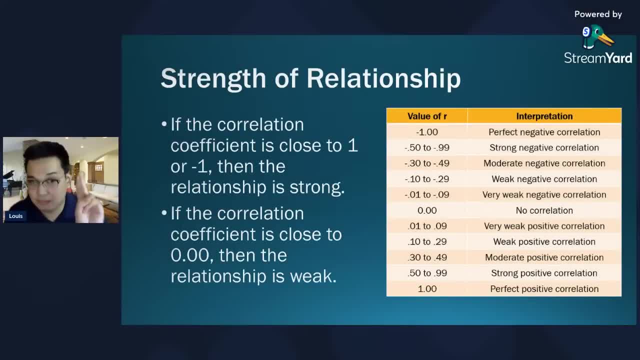 Una, yung number. Yung number tells you the strength Pangalawa, the symbol tells you the direction. So this number, for example negative .50, gives you two information already. That is nang unang una since .50,. 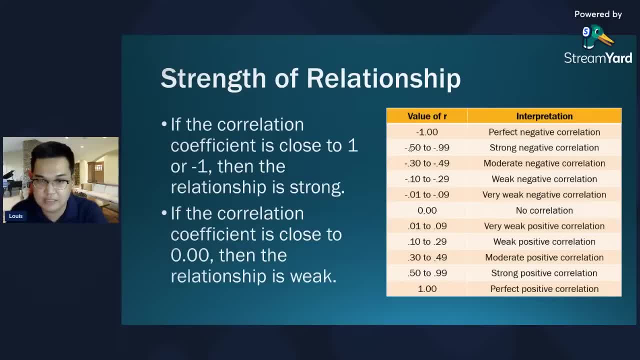 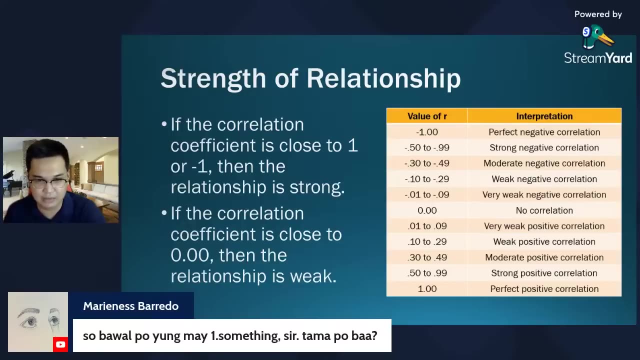 there's a strong relationship Pangalawa, since negative yung symbol, it's a strong negative relationship. Okay, So bawal po ba kunyari lalagpas po ng 1.7. kunyari, Hindi na yun, tama There's. 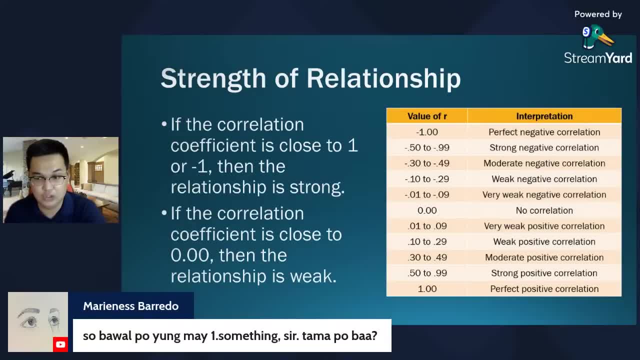 something wrong with the computation. It's impossible that yun yung kakalabasan. Okay, Ayan Ayan Kay Ma'am Jelay daw naalala ni PsychReview PH Nalala ko kasi nung 2017, yung. 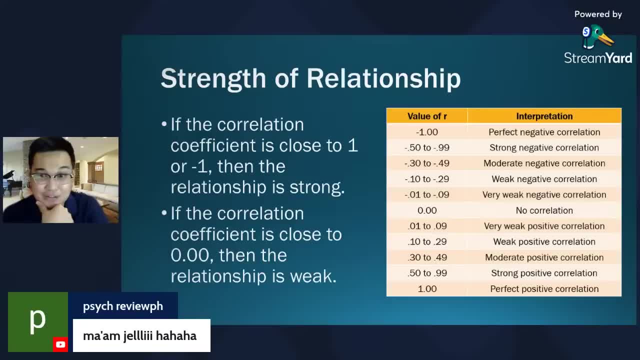 namin, si Ma'am Jelay, gumawa Tapos tawa, kami ng tawa, kasi nga yun yung tamang sagot: hire a new statistician. Mula nun, hindi ko na nakalimutan yung joke na yun. 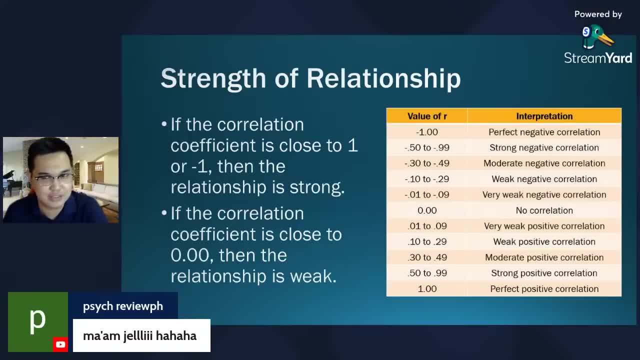 Okay, Dati siyempre review pa ako Alam mo bakit Hire a new statistician? Ngayon gets ko na kung bakit yung sagot ay hire a new statistician. Ayan Item pala. 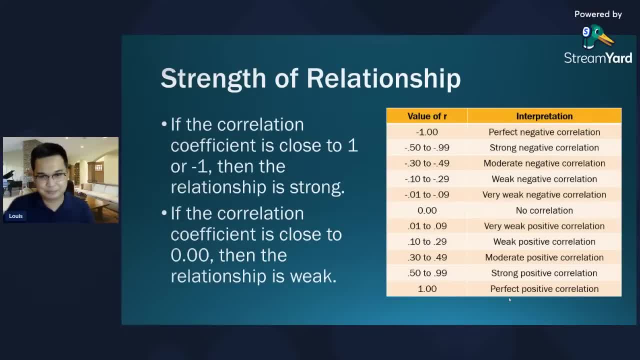 ni Ma'am Jelay, yun Kaya hindi kumatak sa akin yun. Ayan, May tanong kayo dito. Ayan, Yeah, Kapag yung hindi naman lahat, kapag natuwa lang ako sa message yung ko nilalagay. 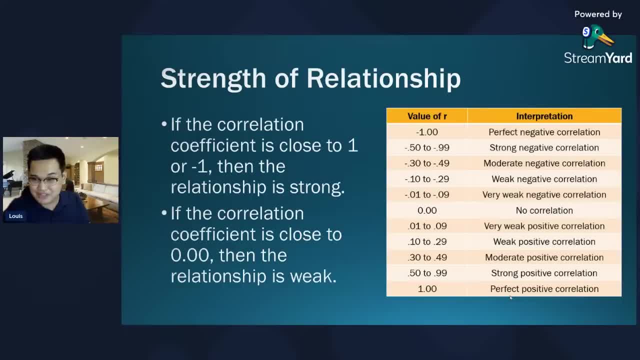 sa screen. Okay, They have questions in about this one. So gagawin natin, I think, mag-aanalyze tayo ng data. Okay, Tapos titignan natin yung, i-interpret natin yung. 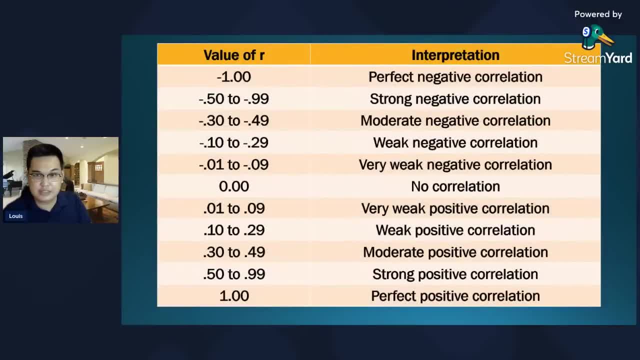 results. Okay, Ano ba. next, Slide 2.. Ayan, Okay, This is just the bigger version. by the way, Okay, I'm preparing the data. Okay, Before we continue, And to visualize. by the way, 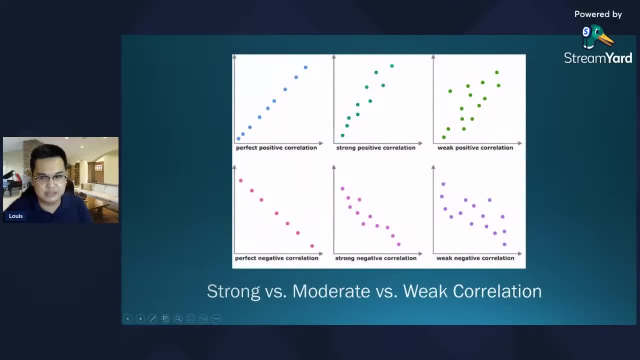 because most of you would like it. if we can visualize, no, Okay, Kung i-visualize, natin ganito yung itsura ng perfect positive correlation: The dots are forming a straight line And tingnan nyo kapag positive correlation. 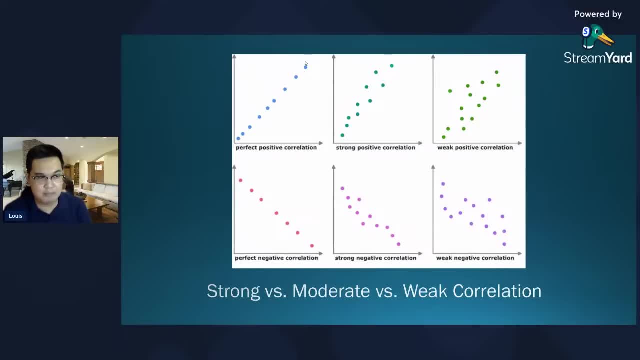 the pattern ay: papunta sa upper right. Pag pa-upper right yung pataas, tapos papunta sa hanan. Kapag positive correlation, The weaker it becomes, the more scattered okay yung mga tundo And the same. 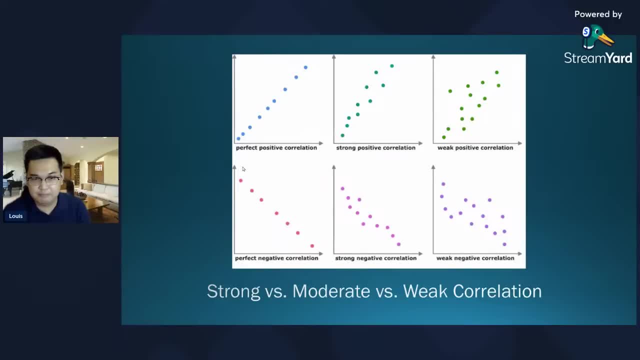 for negative correlation, Pero sa negative pababa siya Papunta sa lower right instead na pataas, And the weaker it becomes, the more spread out. Okay, Ngayon, some you know things to clarify. 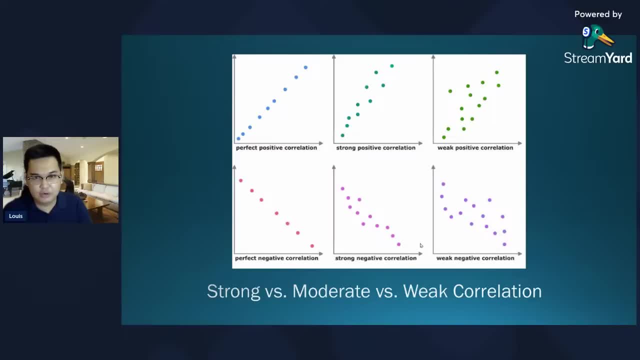 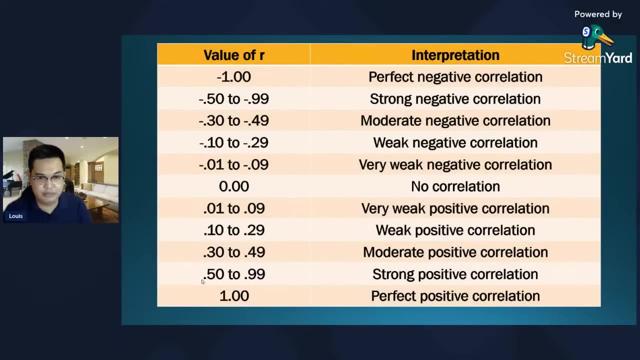 Kunyari, iko-compare natin yung correlation na balik tayo doon sa kanina. Iko-compare natin yung negative 0.5 tsaka yung positive 0.5.. Kunyari yung tanong: no Anong stronger. 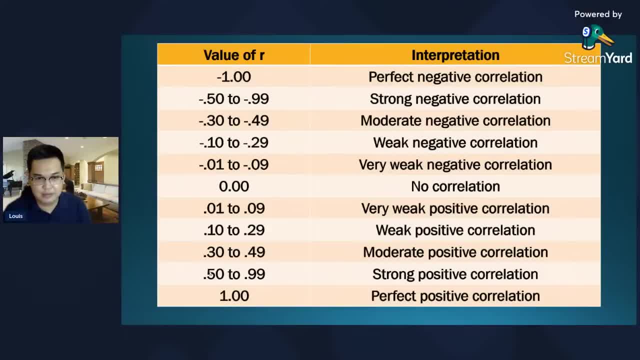 Negative 0.5 or positive 0.5? Okay, Anong isasagot nyo doon, Or same lang. ba sila Kunyari yung tanong. no, Which is stronger: Negative 0.5 or positive? 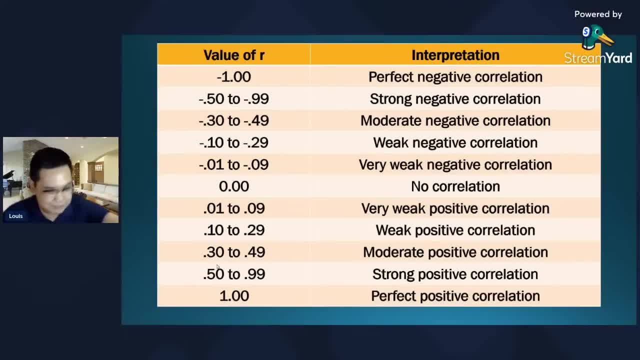 0.5? Or same lang sila. Okay, Kung alam mo hindi kita ipa-flash sa screen kung natatakot ka Yan, Very good, no, Kung ang usapan natin is the strength of relationship. 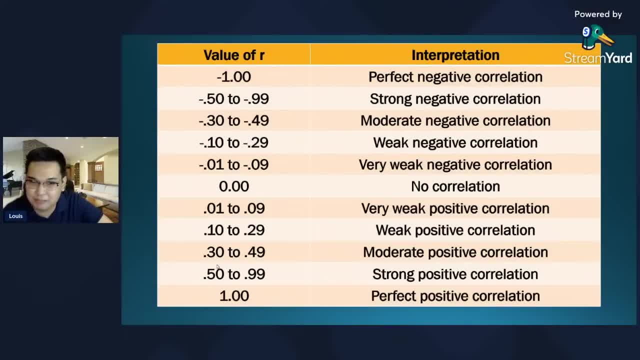 same lang sila Negative 0.5 or positive 0.5? Hindi basihan ang symbol for the strength. Ang basihan ng strength is the number. So you ignore the symbol. Pero kung tatanungin kayo, 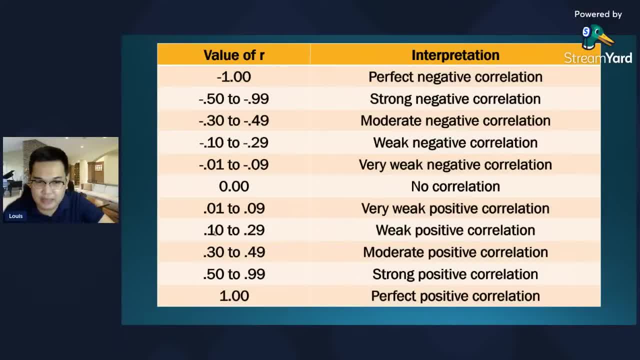 which is stronger: 0.10 or 0.50?? Of course, what is stronger is 0.50.. Okay, Even if negative pa yan, which is stronger? Negative 0.10 or negative 0.50? Stronger. 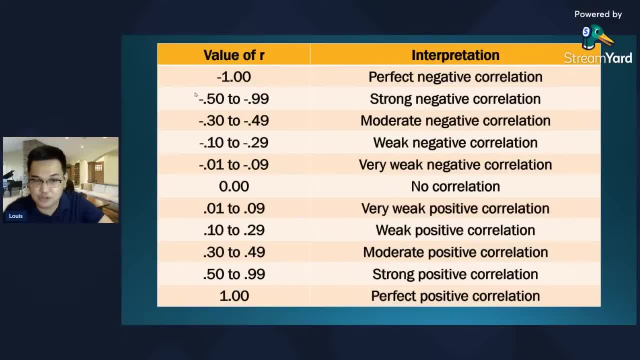 si negative 0.50.. Because you ignore the symbol. The symbol is only for the direction. You look at the value Kung baga sa stats. kung baga sa stats, ang tawag dyan alam ko sa math. absolute value. 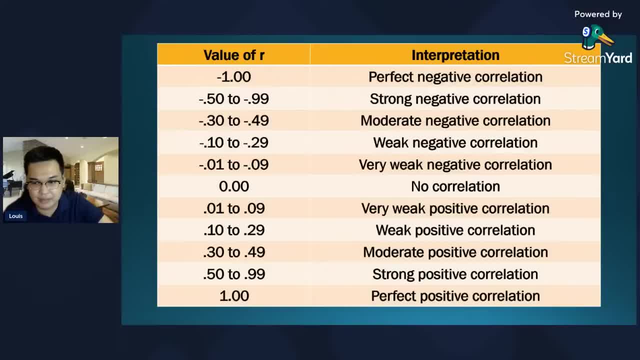 You ignore the symbol. Okay, Yan, Hello, sky. No, Yan Mga familiar names na aalala ko. Baka may iba pa sa inyo na familiar yung name, saan Mararecognize ko yan. 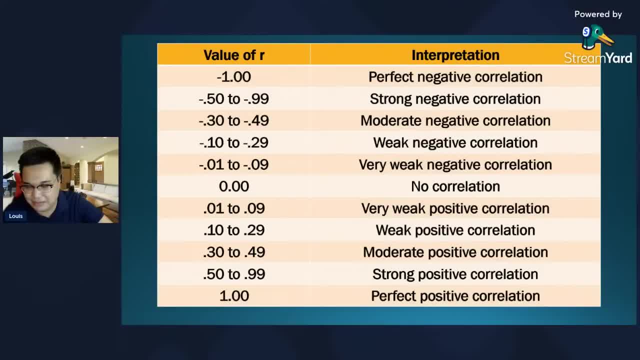 Okay, Yes, Very good, Tama yan. The closer to 0, yan. The closer it is to 0,, the weaker it is Yan. That's correct, Okay, Sige, Masisave naman ito after. 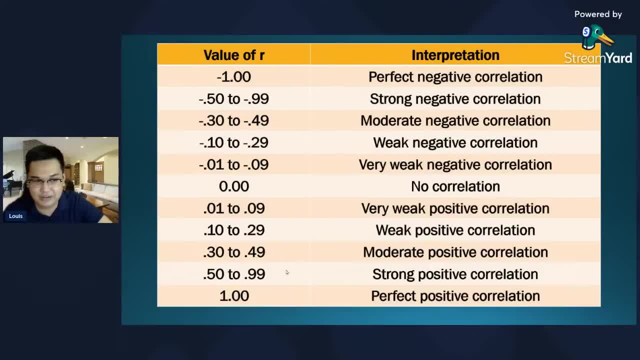 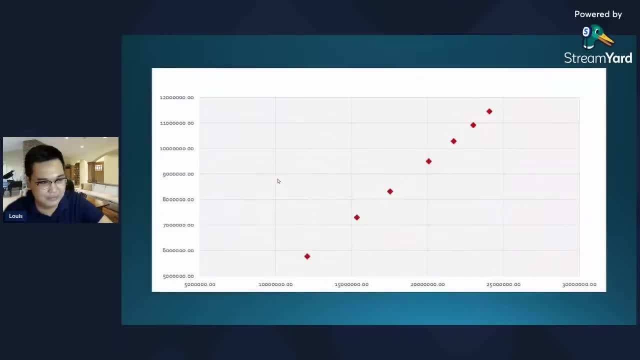 Pero ang gusto ko sa live magtanong kayo, Unlike sa recording. Yan, Okay, Sige, So ito natapos na natin ito kanina. So we're good with this one. Another example of perfect relationship. 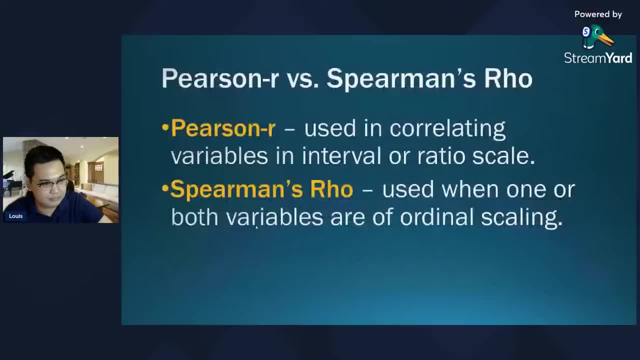 Okay, So yan Straight line. And before our demo: okay, there are different ways to run correlation, Pero inside we usually make use of Pearson R and Spearman Rule. Okay, Yung, Pearson R, gagamitin mo siya. 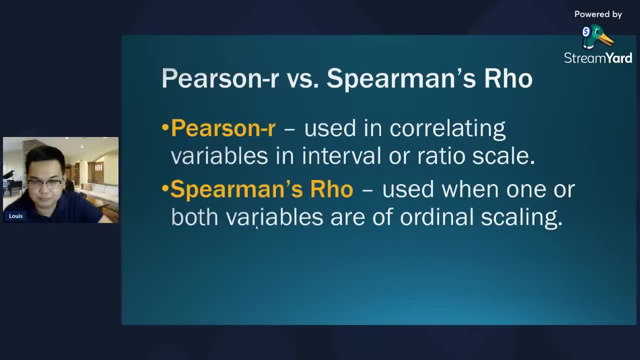 kapag yung dataset mo okay, either interval or ratio, Kunyari yung mga psych test. kasi diba sabi ni Cohen yung sa psych assessment yung data na kukuha mo dyan is treated as interval. 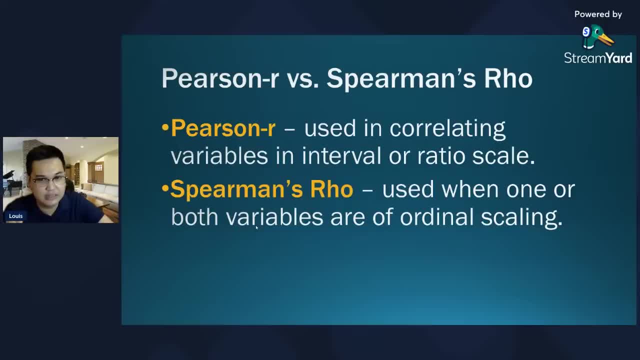 Kaya sa reliability, tsaka sa validity, tsaka sa test development ang ginagamit Pearson R, Okay, Gets yun. na kung ba Pearson R lagi sa psych assessment, Kasi yung mga data yielded by psych test are treated. 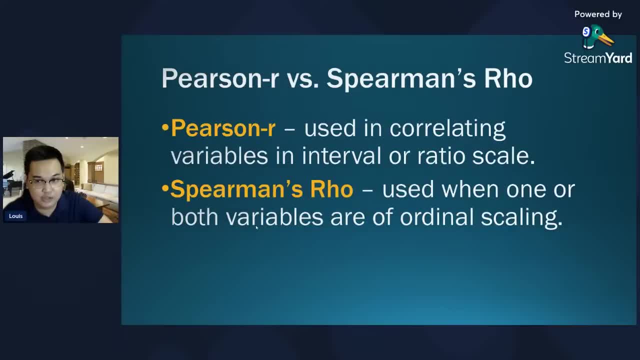 as interval. Pero take note, ah, hindi ito yung usapan tunay. Pero kasi yung sa Likert scale na 0,, 1,, 2,, 3,, 4,, 5, ordinal yun, Pero kapag ginawa mo yung, 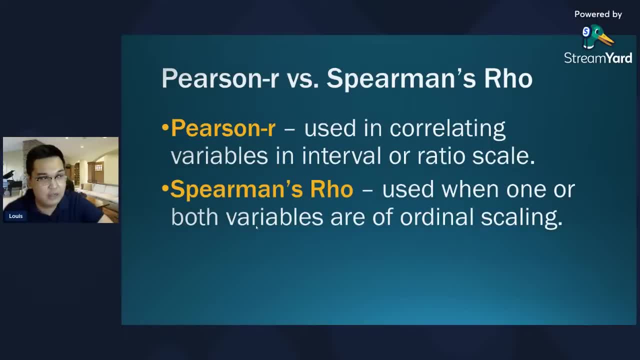 total. that's when it becomes interval Kunyari. no, you would like to correlate MMPI with back depression inventory. Eh, pareho yung interval level kasi pareho yung psych test data. So gagamitan mo ng Pearson R Yan. 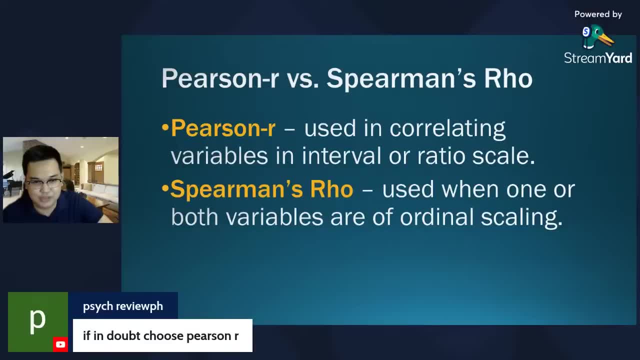 Okay, If in doubt, choose Pearson R daw, Kasi madalas sa psych Pearson R talaga ang ginagamit. Kaya malamang tama ka Unless na lang, kung talagang sure tayo na mali. 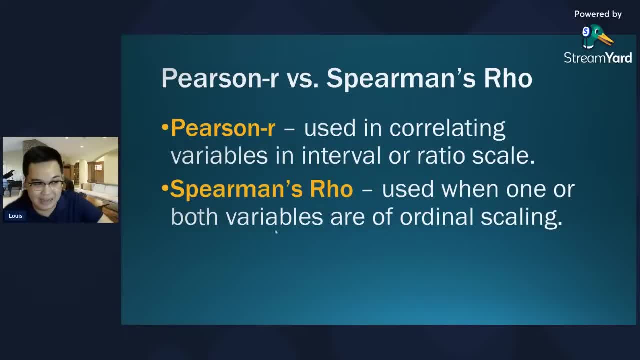 yung sagot Kasi baka yung data ordinal. If the data is ordinal, you use Spearman law or Spearman's rank order correlation, And you use Spearman law when you're dealing with ranks or with ordinal. Okay? 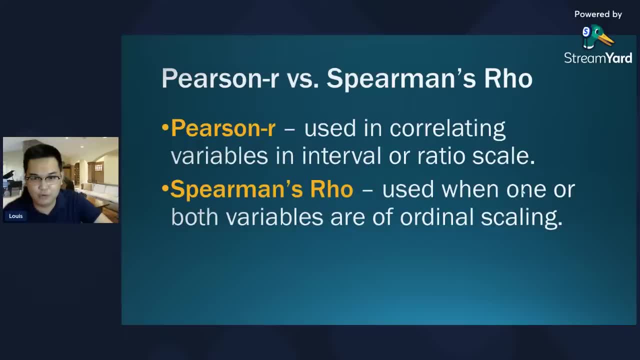 Gagamitin mo si Spearman law. kung isa sa variables mo ordinal or kung parehong ordinal. Okay, For example, correlation of your rank in RGO pre-boards with your rank in the board exam. So, since both are rank and 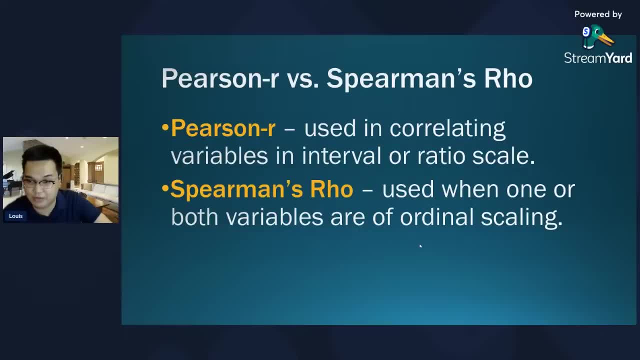 ranking is ordinal. you use Spearman law. Okay, So ayan, Tonight I will cover yung Kendall's Tau. Okay, Hindi antagal ko nang honestly hindi ko ginagamit ito. I do double check ko lang kung. 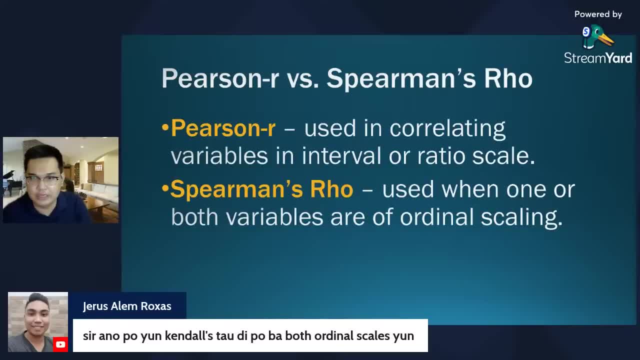 kung nominal ba ito or ordinal. Alam ko nominal ito, I do double check ko lang: Parametric: Ordinal, Ordinal siya. Sorry, Hindi siya nominal. Ordinal pala siya, You're correct, So ordinal siya ginagamit. Pero 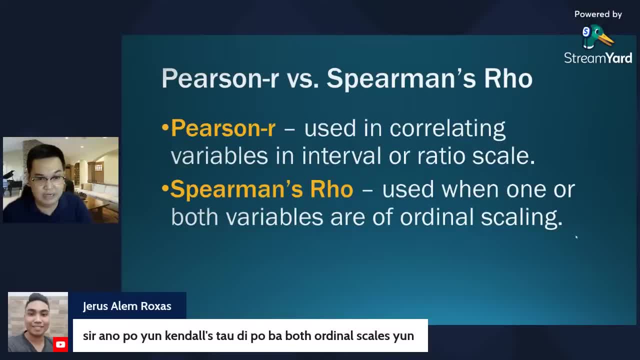 I'm much more familiar with Spearman and I don't usually use Kendall's Tau, Kaya I'm not so familiar with it. kasi di ko siya ginagamit Mas comfortable ako with Spearman's law. Okay, Pero paano. 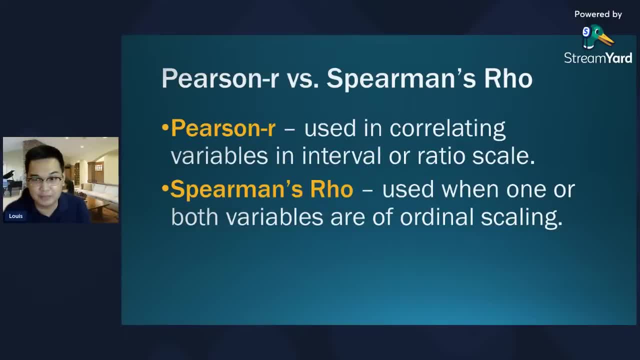 naman kapag parehong nominal, yung i-correlate mo Anong gagamitin mo. Kung parehong nominal, naman, that's the time you use Chi-square, Okay. So in other words, Sir paano malalaman, ano yung appropriate treatment. 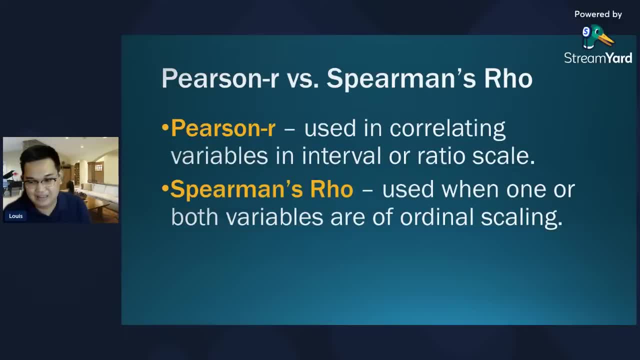 Nakadepende yan anong data meron ka. Okay, Nakadepende yan kung anong data yung meron ka. So kung chi-square nominal, kung parehong ordinal, you can use Spearman rule. 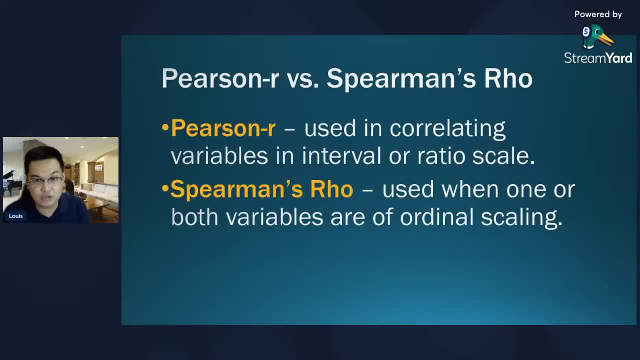 Okay, Kung interval or ratio, you can use Pearson R. Okay, Ayan Sige, I think magde-demonstration na tayo. Okay, Let me just open the dataset so that we can apply what we learned. Here's our. 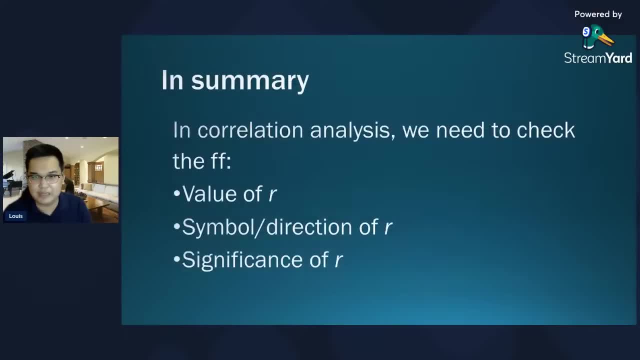 problem, By the way. in summary, okay, when running a correlation analysis, you need to look at the following. Ito yung three-step recommendation ko. Three-step recommendation Una: look at the value of the R. Yan yung una Titignan mo. 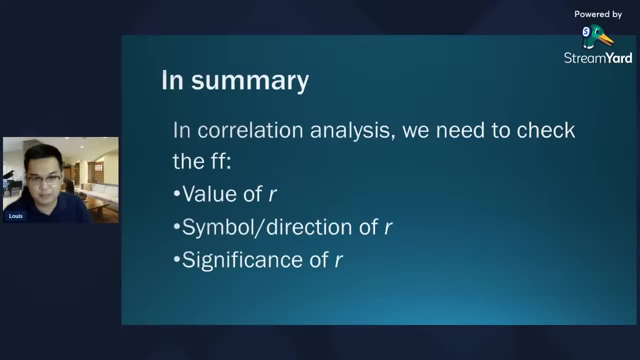 yung value ng R Later. makikita natin yan After mo makita yung value ng R. yun next na titignan mo is the symbol or the direction of the R And lastly, titignan mo yung. 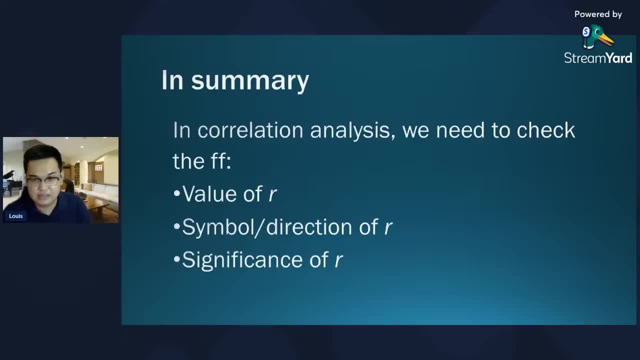 statistical significance. Sir, ano yung statistical significance? no Masasabi nating significant yung correlation kapag yung p-value is less than .05.. Pwede rin siya maging less than .01,, less than .001,. 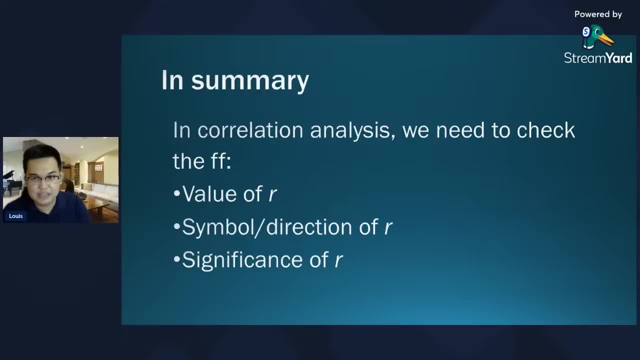 but the cutoff is .05.. Okay, Sir, bakit titignan yung significance? I'll explain in a while. okay, I'll explain in a while. For now, para hindi kayo ma-overwhelm, let me do a quick demo. 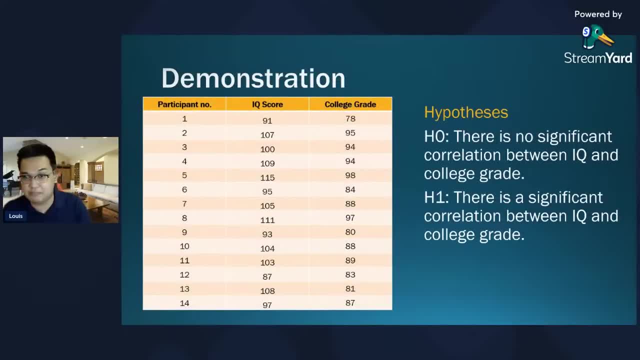 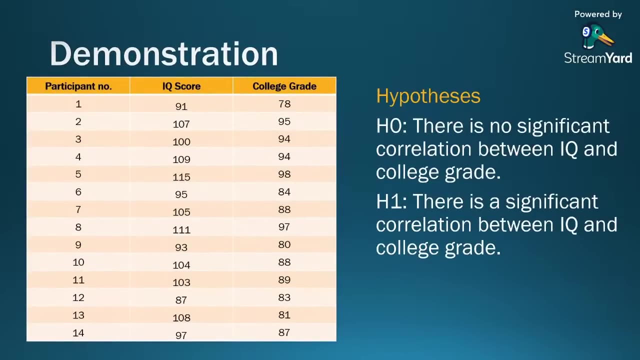 before we instead na mag-stick tayo sa concepts lang. In this data I prepared for you tonight, we will correlate para sa assessment related. we will correlate IQ score okay with college grades Okay. so on the second column, we can. 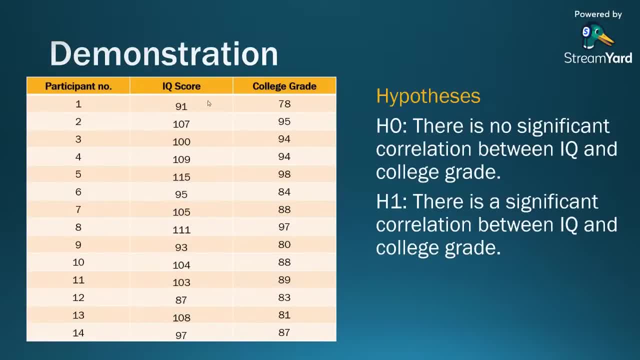 see here the IQ scores of our participants, while on the third column we can see here their college grade. Hindi pa siya na-transform na yung one point, something no pang high school kunyari yung grading system. On the first, 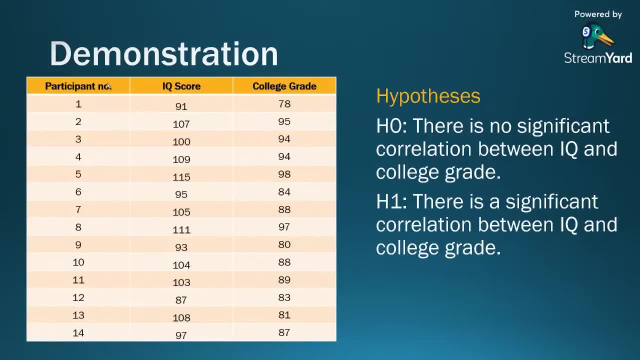 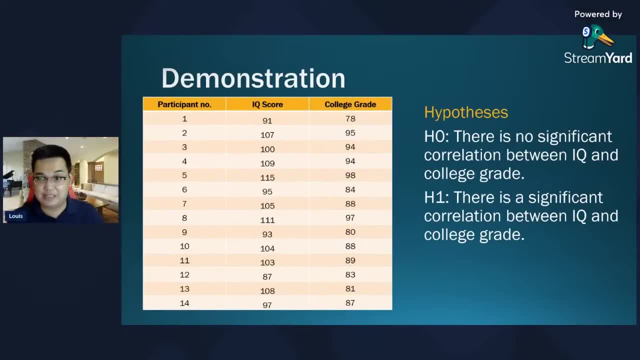 column. you can see here the participant number Yan. Okay, Common question sa mga video ko, sir, saan po nakuha yung values na yan? Nagpa-test ka Ang assumption dito? nakapagpa-test ka, For example, for IQ? 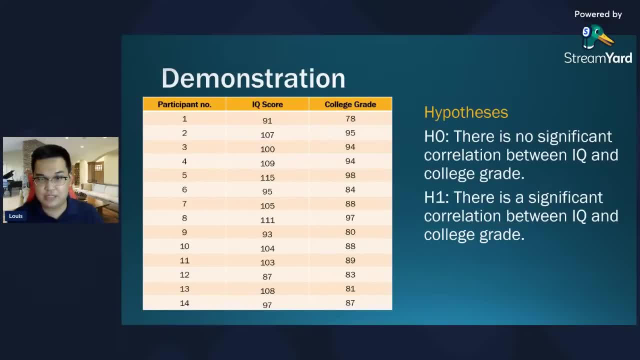 score. kunyari, naggamit ka na ng Raven's Progressive Matrices, Ganun mo may measure yung IQ, Tapos yung college grade. hindi pwedeng tingnan mo yung grade nila sa ano sa. 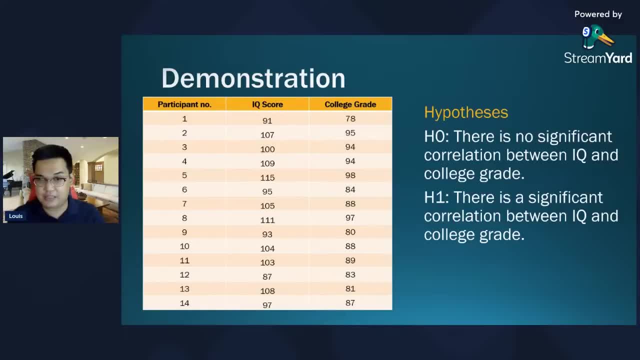 ano yung tawag doon, TOR, Tapos ilista mo sa Excel, Tapos tsaka mo siya i-correlate Yan. And our hypothesis are the following: Our null hypothesis is that walang correlation. no, There's no correlation. 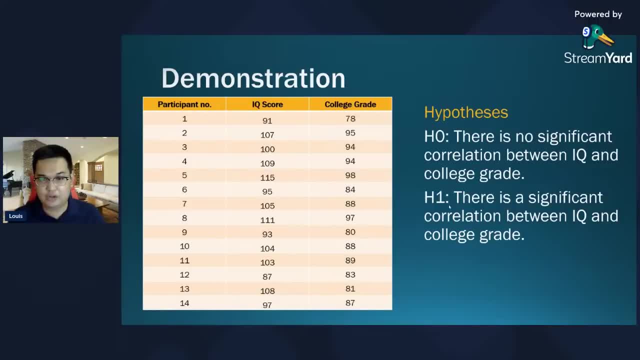 between IQ and college grade, And our alternative hypothesis is that there is a significant correlation between IQ and college grade. So makikita natin, after the analysis, which of the two is correct. Yun bang HO, Or we also call it H0? Or is it the H1?? 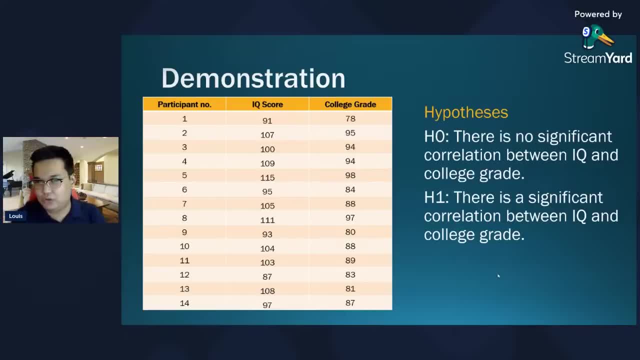 So again, ano, sa tingin niyo, Which of the two do you think will be? Ano, yung ending neto. Do you think it's the H0 or H1? What do you think? Anong hula ninyo, Anong kotog ninyo. 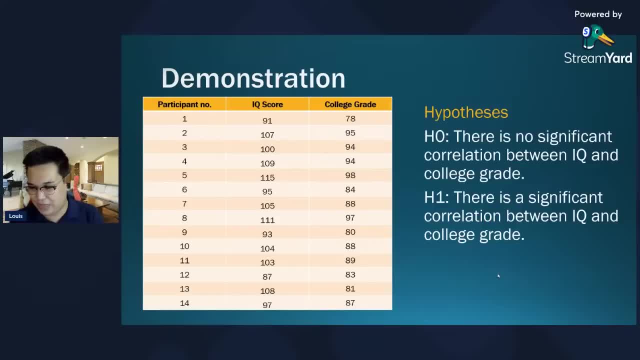 Tapos, tingnan natin kung tama yung kotog ninyo. Can you put your answer sa chat or sa comments? pala yung tawag dito: Live chat or comments. Okay, Do you think ang ending neto totoo? 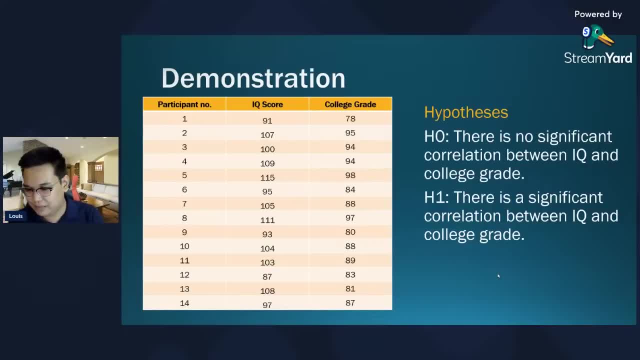 yung H0 or H1? Ayan, Sabi nila H1 daw. Okay, Sige, Yan ang kotog ng taong bayan. Okay, Sige, mag-analyze tayo Whenever I teach stats in the university. 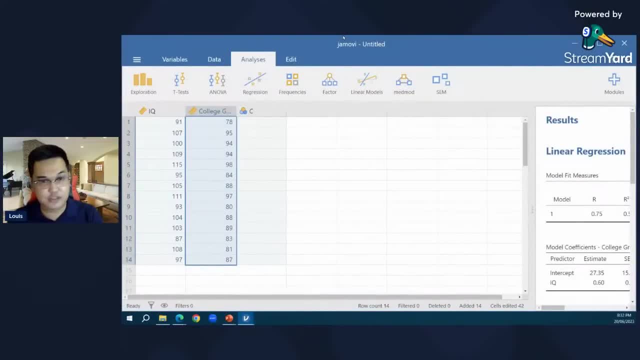 I use Jamovi, I also use SPSS, Pero hindi naman ito stat class. This is an online lecture, Kaya mag-Jamovi na lang tayo. It's very easy to understand Those who have been following my YouTube channel. 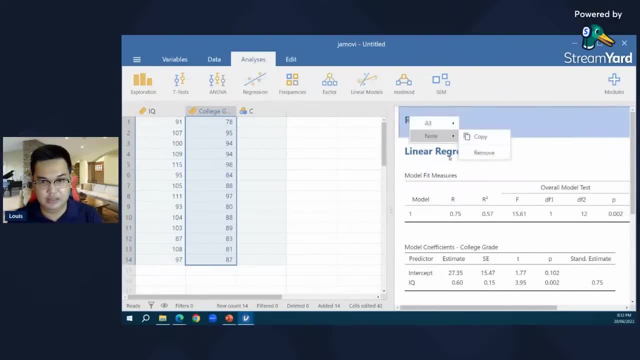 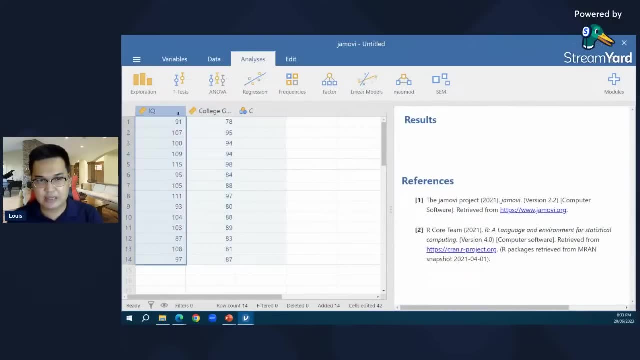 for quite some time know that I love Jamovi. I will just delete this Nag-analyze kasi, ako before we started, So from Excel I copied the data onto It. can be SPSS or Jamovi, whatsoever, Okay, So ito yung IQ nila. 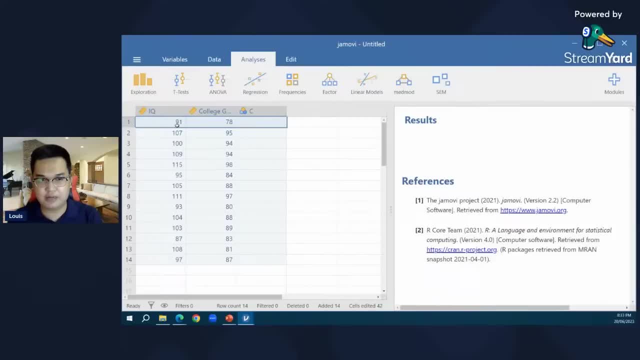 Kunyari ito sa participant 1.. Yung IQ niya 91 sa Ravens College, grade niya 78.. Samantalang si number 2, ito medyo matalino to 107 IQ niya, Tapos grade niya 95.. 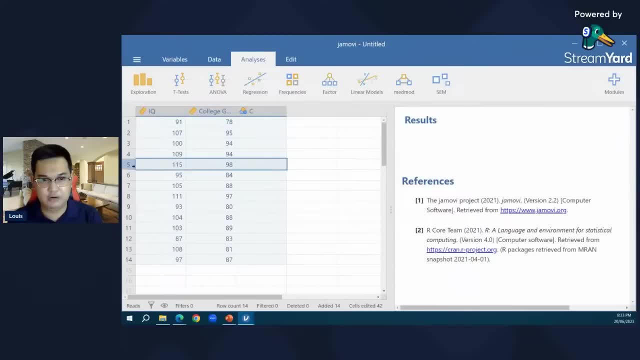 Tapos itong si number 5, ito feeling ko honor student to Or with highest honors, IQ niya 115.. Taas One standard dev above Okay, Tapos college grade niya 98.. So in other words, 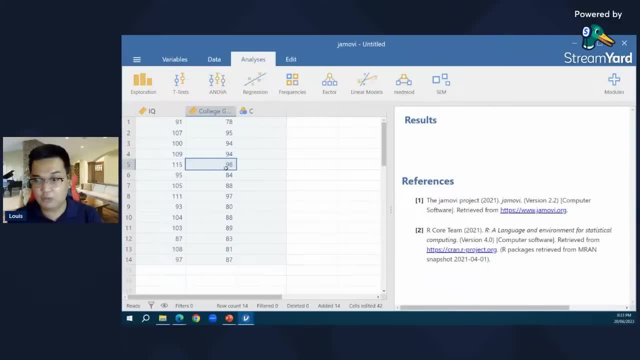 sige na natin related ba or not, Ako gumagamit ako ng JAS, I also use JAS, I also like it, Pero mas fun ako ng Jamovi Sige mag-analyze tayo To correlate. 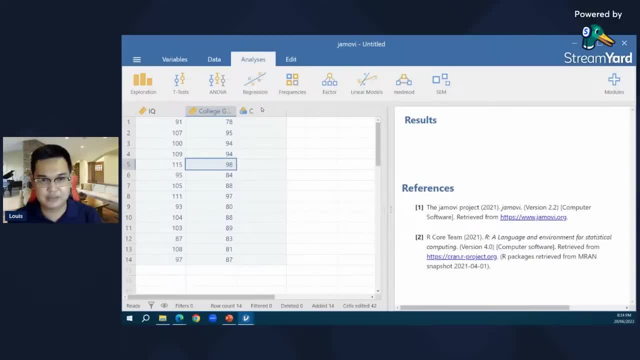 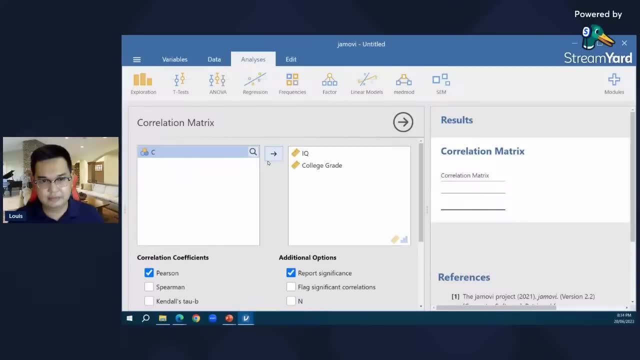 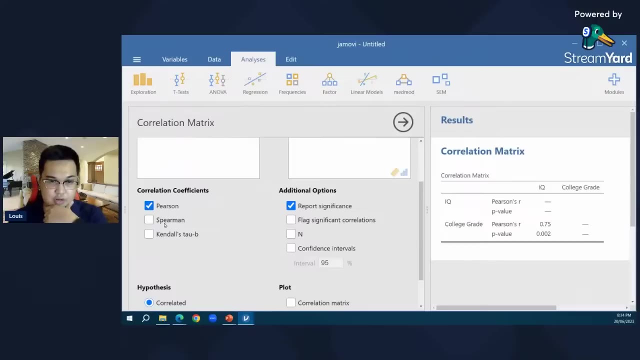 let's click on regression and let's click on correlation matrix. Idrag lang natin yung dalawang variable that we want to correlate sa kanan And may ito check. So na dito sa kaliwa it shows ano bang gusto mo, Pearson or Spearman. 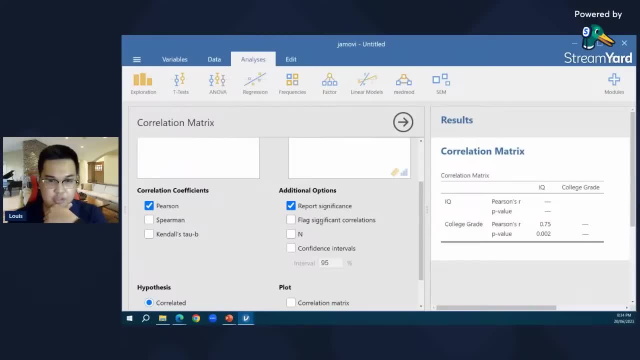 Rook Endels Tau. Okay, And here are some other options. Let me check on flag significant correlations. Okay, And I think that's it. So saan na po yung flag significant correlation Kapag chinekan mo yan? 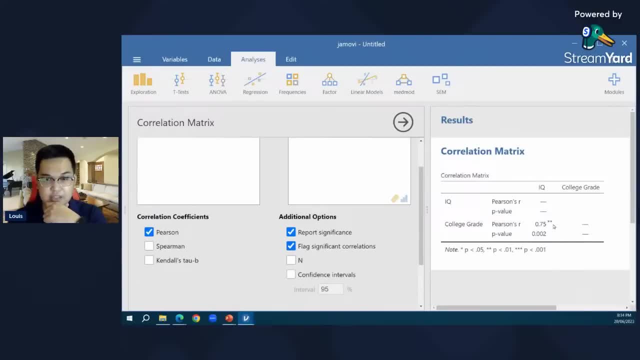 tapos may nakita kang asterisk dito sa kanan. it means yung variables mo correlated. So sabi ko sa students ko: lagi niyo chucheckan yan, Kasi kapag nacheckan niyo yan, 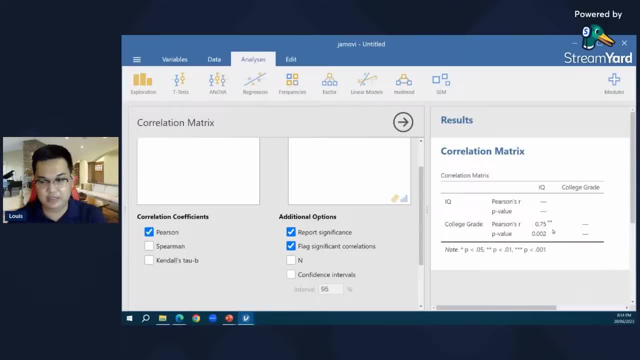 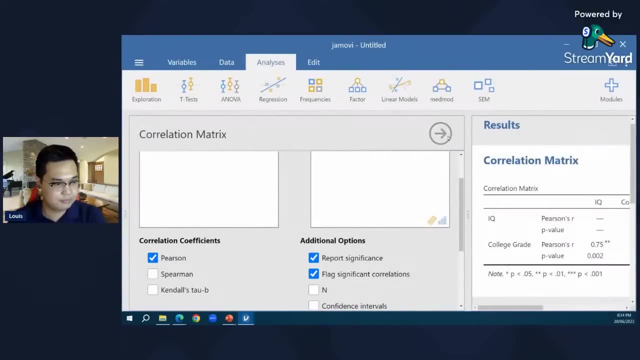 ibig sabihin, kahit hindi mo tingnan yung p-value, alam mo na significant sila. Okay Ay medyo maliit pala on your end, So let me zoom in. Okay, Yan. So ito yung results natin. 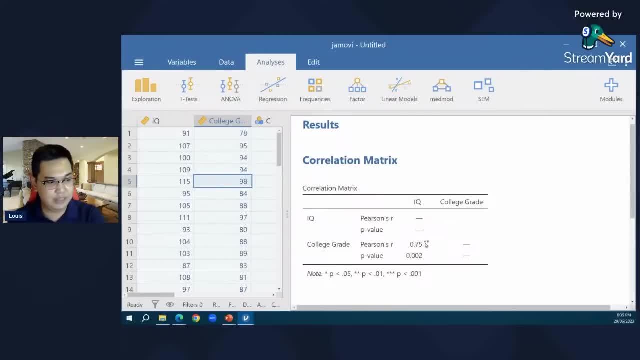 Okay, Point seventy-five may dalawang asterisk. Anong meaning yan? Kung titingin kayo sa baba, pag dalawa yung asterisk, it means significant siya, at p-value less than .01.. So ano ang ibig sabihin? 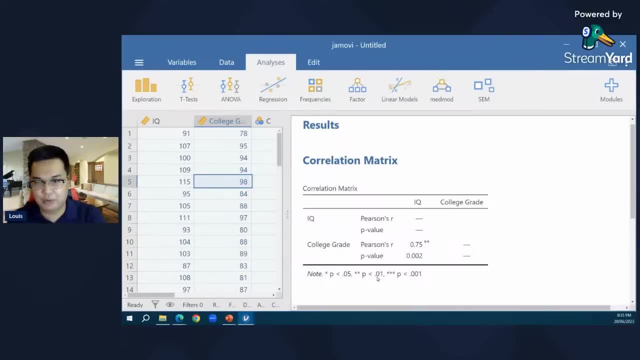 yan Ang ibig sabihin yan: kapag less than .01, sure tayo up to 99% chance na correlated talaga yung IQ tsaka college grade Yan Tapos. so what does this mean, Sige? 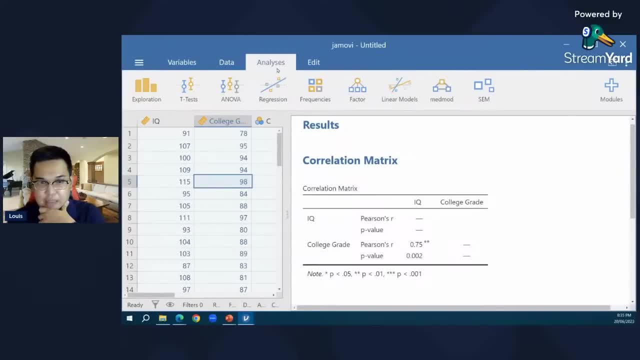 interpret natin ng sabay-sabay yung results. Interpret natin First yung unang tanong ko in terms of direction: anong relationship yung nakita natin dito sa IQ and college grade? Is it positive or negative? 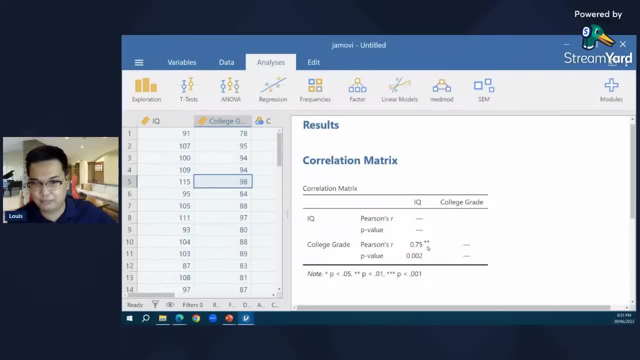 Di ba yun yung. step one: Look at the R. Step two: look at direction. So ano nakita natin Positive or negative? Oo, free din ang jamovie. Very good, There is a positive relationship Kapag walang negative sign. the relationship. 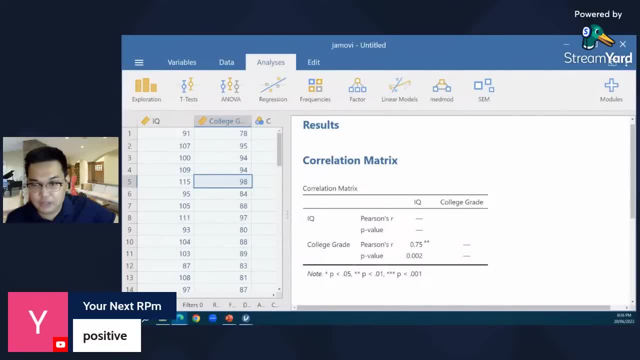 is positive Pangalawa in terms of strength. what can we say about the strength? Is it weak, moderate or strong? Going back to the discussion earlier, So una positive siya Pangalawa. it's also weak, moderate. 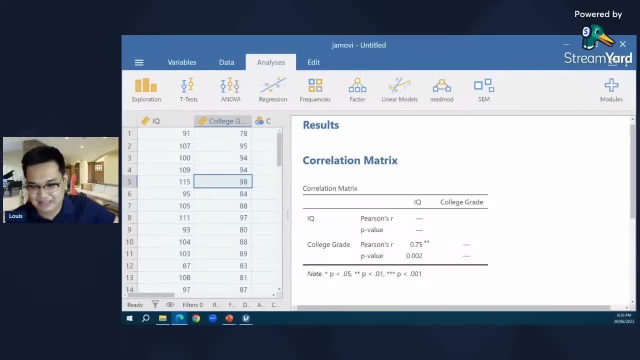 or strong or baka naman perfect. Since .75 is malapit-lapit na sa one, it's already very good, Strong relationship. So if we combine that to one sentence, there's a. there's a strong, positive relationship. 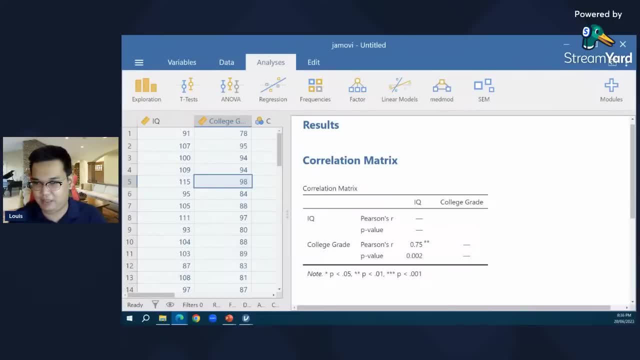 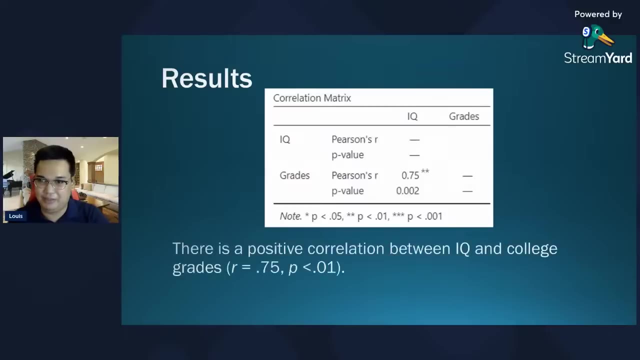 This is correct. Nag-promise pala ako sa hindi kita ipapakita, Hindi ko nalang isi-share sa screen yung sagot mo, Anyway. so, going back to my PowerPoint, here's the result we obtained and here's the interpretation. 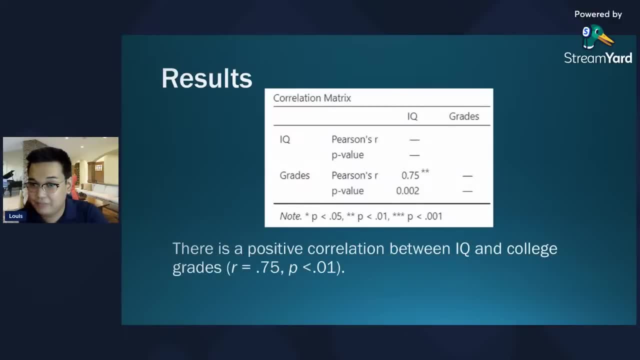 There is a positive correlation between IQ and college grade. Actually may kulang na word dyan, Alam niyo kung anong kulang. There is a significant positive correlation. So ano ulit yung meaning ng significance Kapag yung relationship significant. 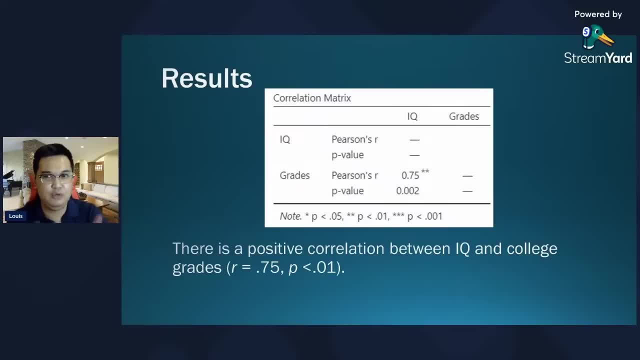 it means generalizable. siya Yung meaning mo sa research mo pwede mo siyang i-generate sa entire population. Meaning etong finding neto is not only true for the small group of people you recruited, it's also generalizable. 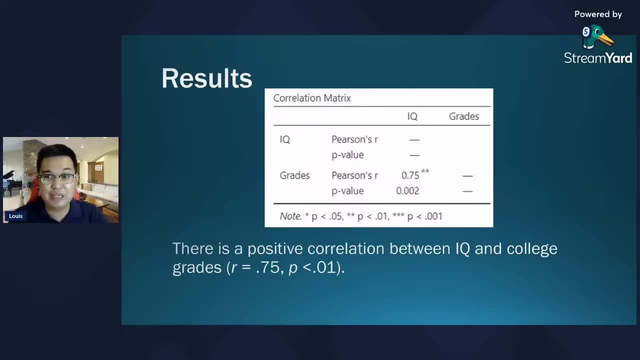 outside your study. Ganon yung meaning ng significant Kapag, significant yung correlation. what is true for the sample is true for the population. So this neto hindi lang siya totoo about the small group who participated in the study. 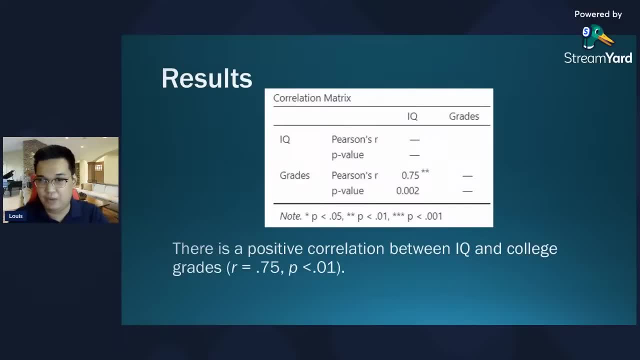 But we have confidence to say that our finding is also generalizable to people not involved in the study. Okay, And other than that, other than that, paano nasabing significant sir, Paano nasabing significant, Una-una may. 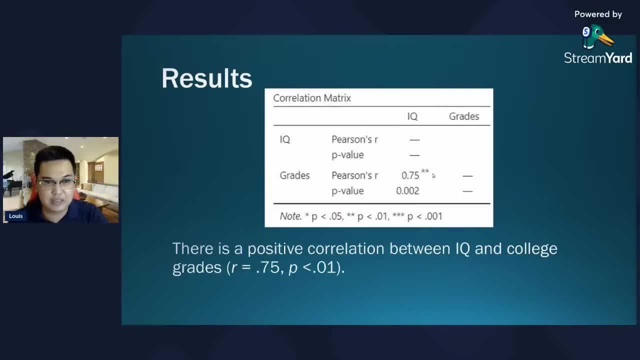 dalawang star: Okay Kapag dalawang star less than .01.. Actually, kapag isa lang, considered na yun na significant e So mas maganda kapag dalawa, mas lalo pang maganda kapag taklo Kumbaga. 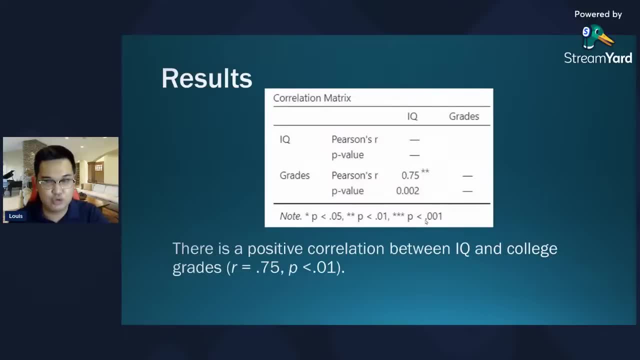 kapag taklong star it means okay, sure tayo, 99.9%. Kaya, napansin niyo sa mga brand. you know this can kill 99.9% of germs. Kumbaga, ire-relate kayo sa stats. 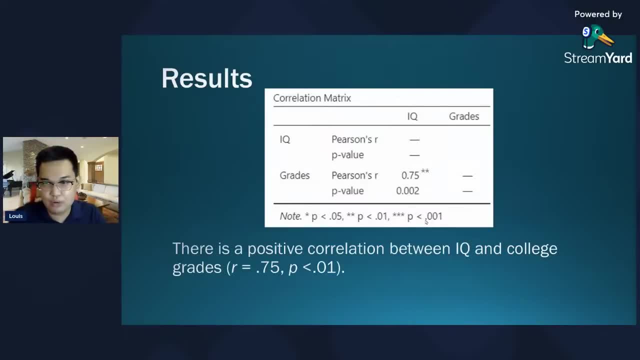 they're saying that significant yung ano nila, yung product nila, in comparison to other products. Ayan, Okay, So statistically significant yung finding natin if we look at the p-value, kasi lowered siya than .05, and 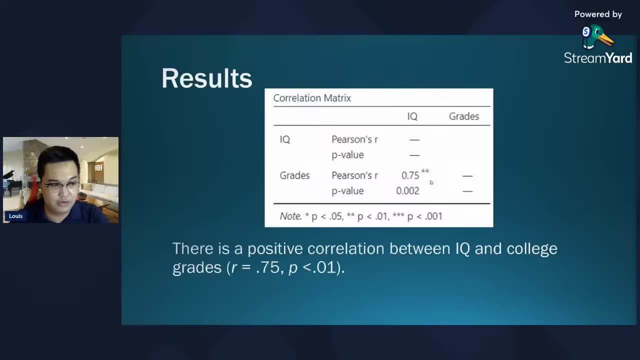 visually we can say it's significant kasi there are also asteris, no, sa kanan nung .75.. So ang conclusion natin: okay, very good, Kapag mas mababa yung p-value sa alpha level, yun yung. 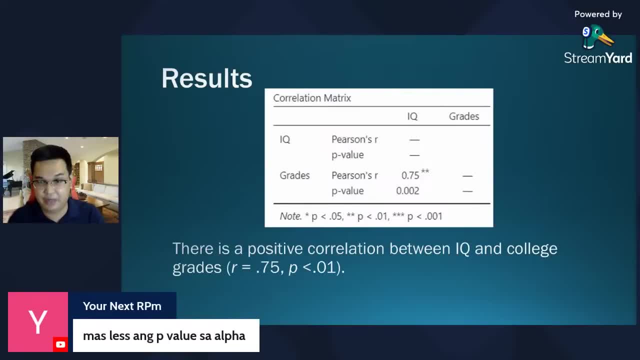 significant. Ano po ba yung alpha level sa psychology, .05.. If the p-value is lower than .05, you say that the relationship is significant. And again, what is significant? What is true for the sample is generalizable to the. 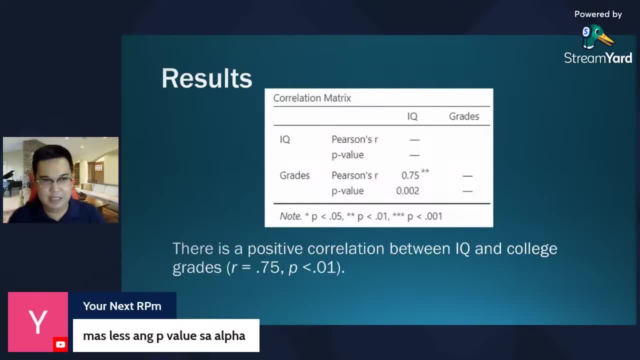 population. Okay. Kapag hindi yan significant, it means wala tayong evidence to say that they are really related. Alam niyo lagi kung mga sinasabi sa students ko na Gen Z. eto yung word na tandaan niyo whenever you. 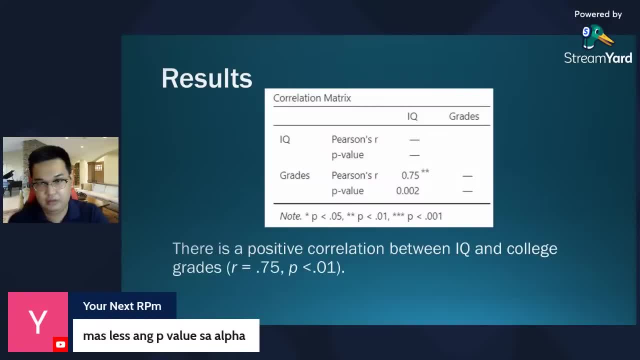 hear the word significant, Tandaan niyo yung word na legit. no, Ibig sabihin legit, yung findings mo totoo talaga yan. Okay, Yung .012 by alpha level din yes, Sa psychology. 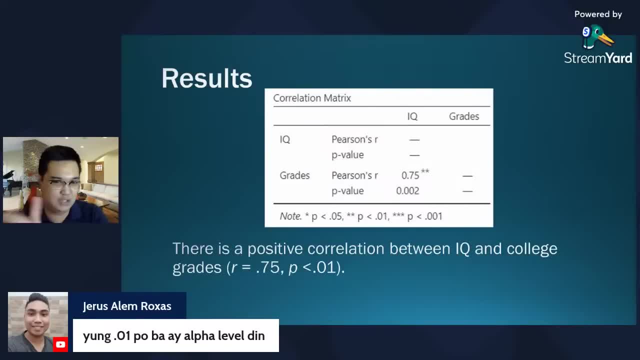 masaya na tayo sa .05.. Pero sa ibang field mas stricto sila. Siguro I'm assuming no Kunyari sa medicine, Kasi I think sa medicine hindi pwedeng ano lang. 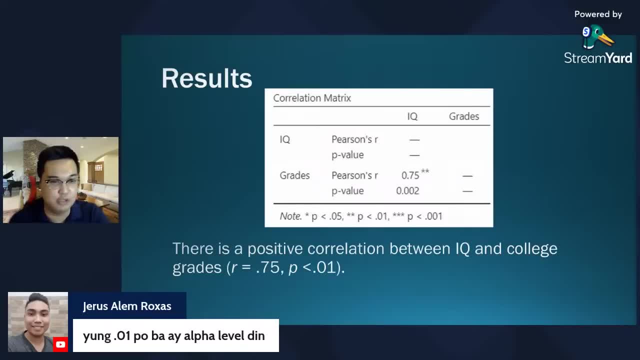 95%. sure ka Kailangan mataas yung accuracy mo dun. So I think siguro I don't know Tanungin yung mga kilala niyong med student kung kapag nagre-research sila. 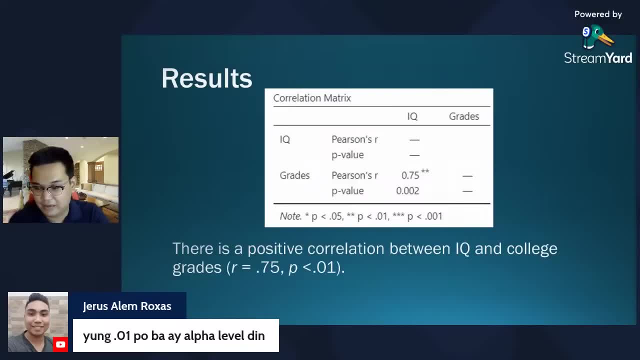 .01 yung gamit Ayan. Okay, This is also correct. no, This is correct, Ayan Pag. less than .01, we are ano, no, 99% sure sa ating findings. Less than .05, mga up to 95%. 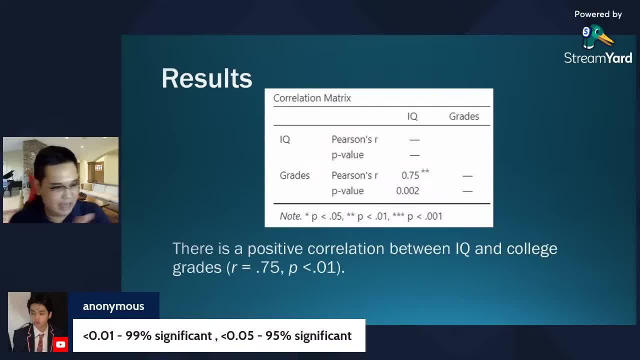 sure lang Ayan. Okay, I hope nakatulong yan. no, Do you have questions, Mamaya? may examples pa tayo. no, Pero at this point parang gusto kong mag-move on to regression. Okay, Pero kung may, 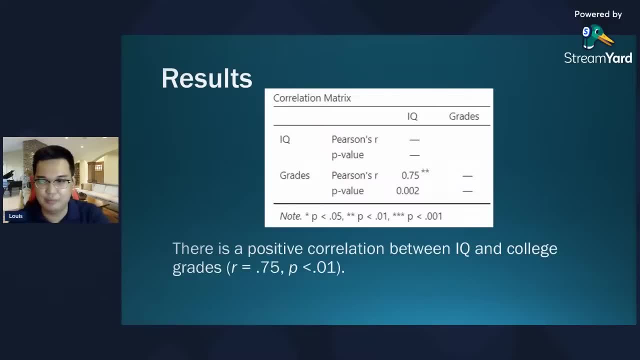 questions kayo. we can look at them one last time before we move on. Bigyan ko kayo ng mga samples Sabi sa inyo thesis mentor ako, So yung mga students ko nagko-correlation din yung mga yun. no One example. 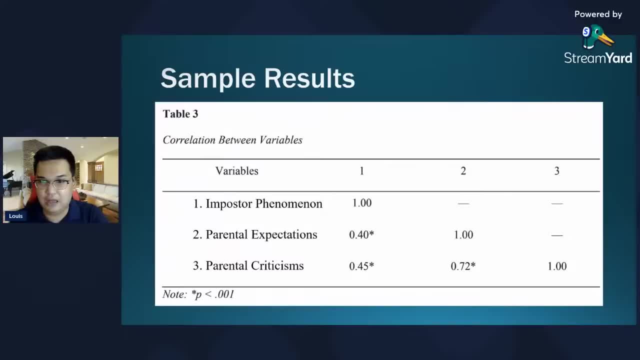 Ayan, Meron akong students eto yung study nila, The relationship of imposter phenomenon with parental expectations and parental criticisms. Okay, So, kung makikita natin, so, paano po ba intindihin ito, Ang tawag dito? 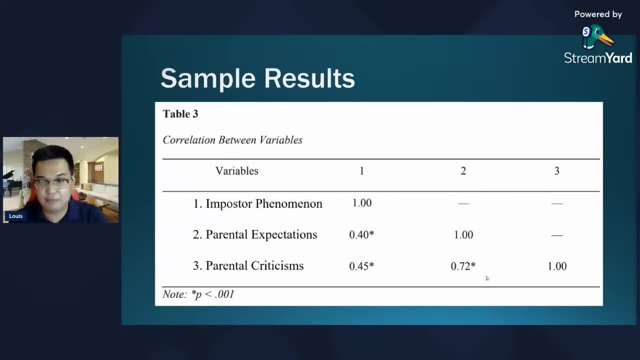 correlation matrix. Kung paano intindihin ito? para ka lang nagmo-multiplication table, Kunyari. no, Paano mo malalaman kung si imposter phenomenon correlated with parental expectations? Parang alam niyo yung imposter syndrome. 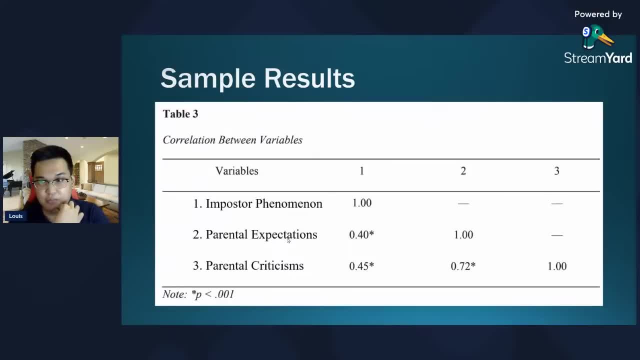 I don't know if you're familiar with that. no, Alam niyo yung imposter syndrome. So tinitingnan nila. ano yung role nung pagiging strict ng parents mo sa imposter syndrome. Alam niyo anong findings nila. 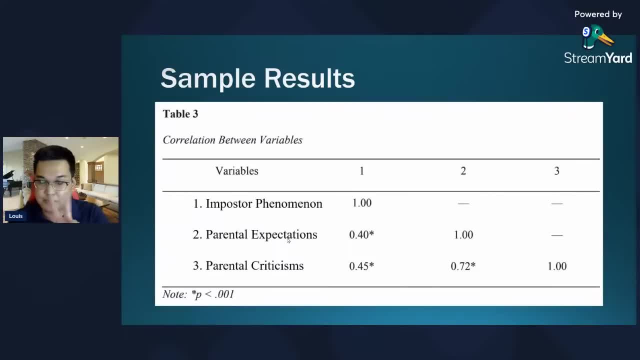 Okay, Dalawa yung sides ng parenting na tinignan nila Expectations and criticisms. Okay, Look at this, Yung si imposter phenomenon, kasi siya si variable one, Siya si number one. Okay, If we look at, 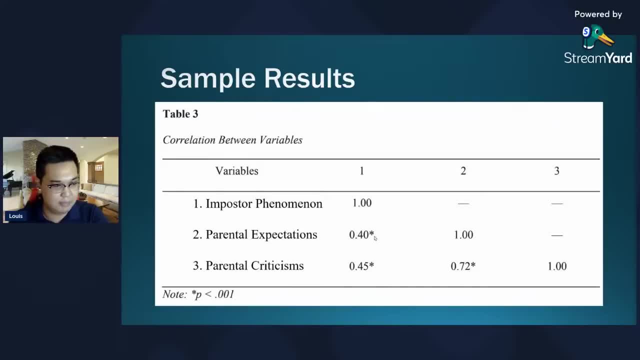 this di ba may point forty, Di ba may point forty, Yung point forty. okay, kung tinitingnan mo siya na parang multiplication table, diyan nagtatagpo yung parental expectations tsaka yung imposter phenomenon. 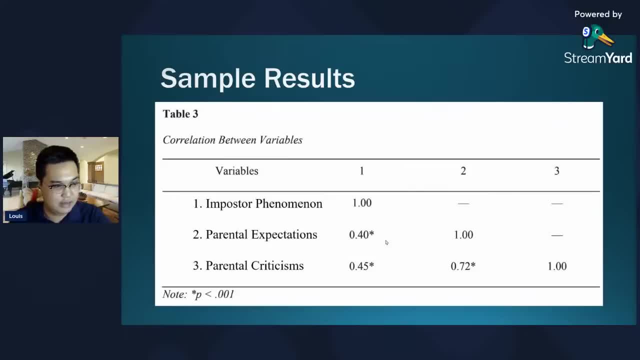 Okay. So meaning the more na maraming expectation yung mga magulang mo sayo kunyari o anak, mag-talk ka sa board exam. ha, Anak, dapat yung rating mo mataas no. 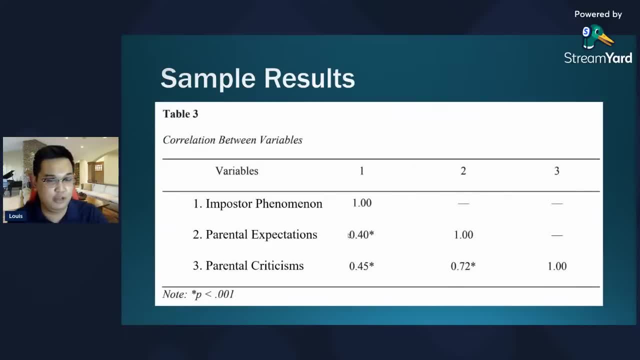 The more na nararanasan mo yung imposter syndrome. I don't know if nakaka-relate kayo. Nakakaranas na ba kayo ng imposter syndrome ngayon? Nagda-doubt na ba kayo sa sarili ninyo? 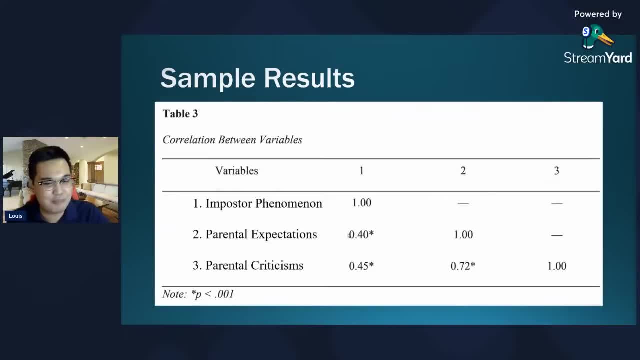 Okay, So yan? no, The more that your parents expect something from you, the more you feel imposterism, the more that you doubt your abilities. Pero you know what's their other finding? Okay, Meron pang isa. 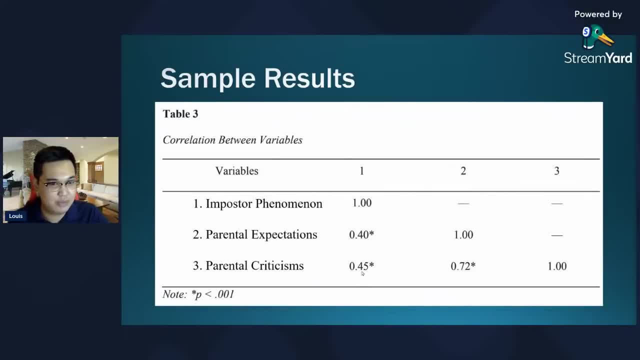 Parental criticisms. Tapos yung correlation niya with variable 1, which is imposter phenomenon- mas mataas, 0.45.. Ay, ay, teka, teka, teka, Um mali ako ng tinignan na value kanina. 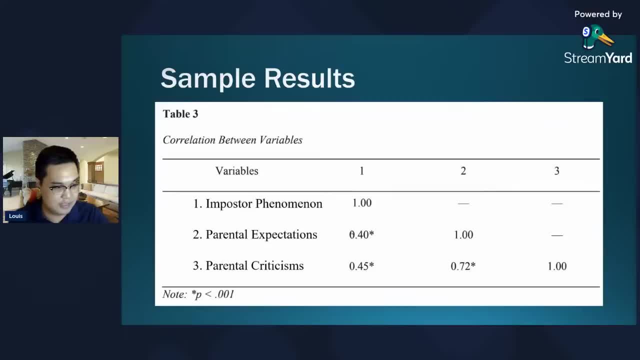 Yun palang correlation ni imposter phenomenon tsaka ni parental criticisms, hindi si 0.40, si 0.45 pala Nakatingin ako sa pangalawa, dapat sa pangatlo. So yung correlation ni parental 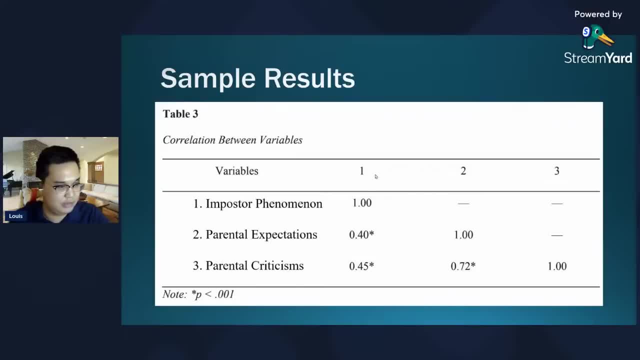 um expectations tsaka phenomenon. ay, tama naman, no Expectations kasi yung kanina. Expectations in imposter phenomenon 0.40.. Pero tingnan natin yung criticisms. Criticism kasi ito yung parang pinapagalitan. 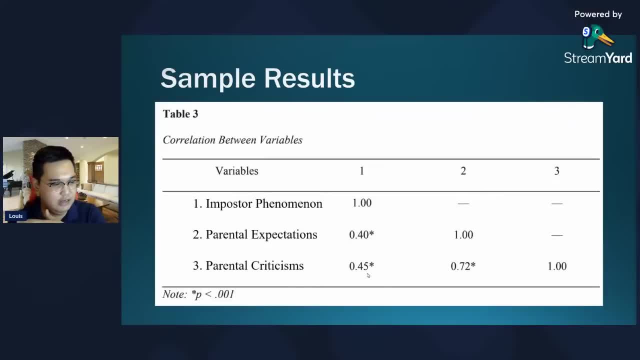 ka na ng magulang mo O anak ba't mababagrade mo Yan O anak ba't hindi ka perfect No 95 na yung score mo, ba't hindi mo pa ginawang 100?. 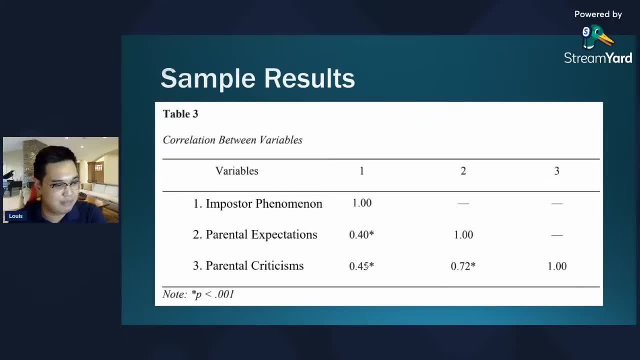 Parang ganun. You know what Mas mataas yung correlation niya with imposter phenomenon. Okay, Kasi yung expectation 0.40 lang, eh, Pero kapag pinapagalitan ka, the more that you doubt yourself. 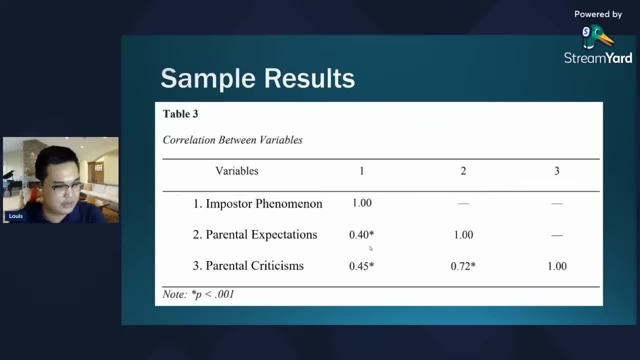 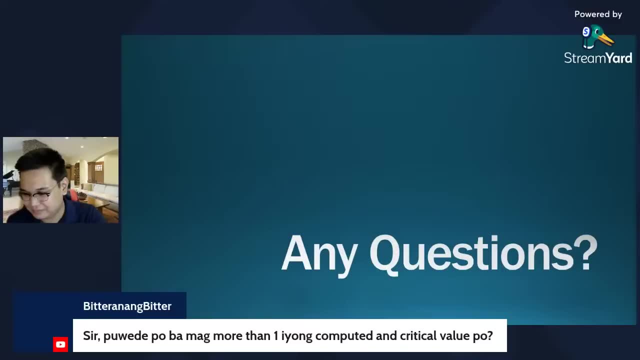 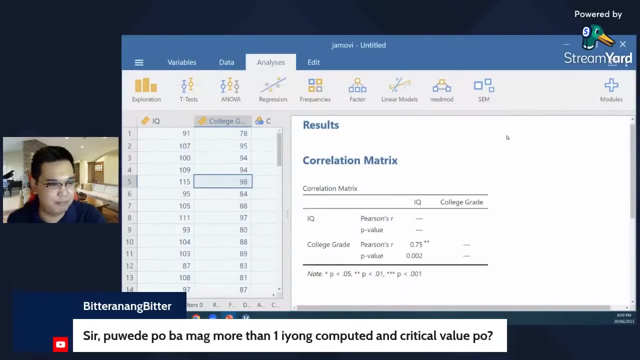 Okay, Yan, yung sa parental criticisms. Okay, Other questions about correlation: Ayan, okay na daw, Sige, no, Alright, Sige sige: Ayan, Okay, So, Okay. So let me prepare my other PowerPoint. 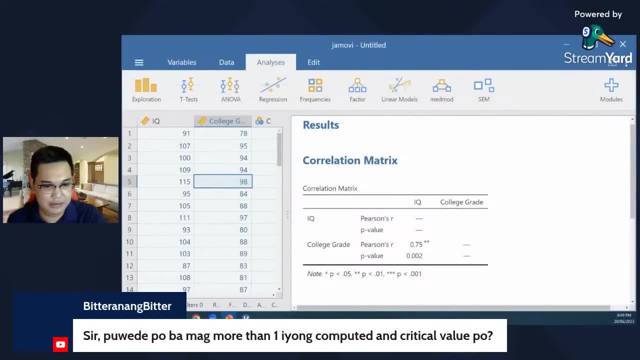 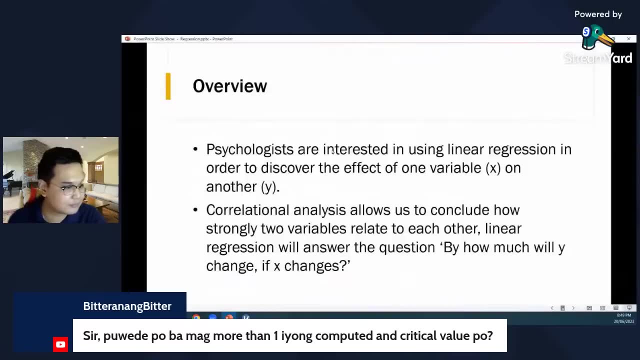 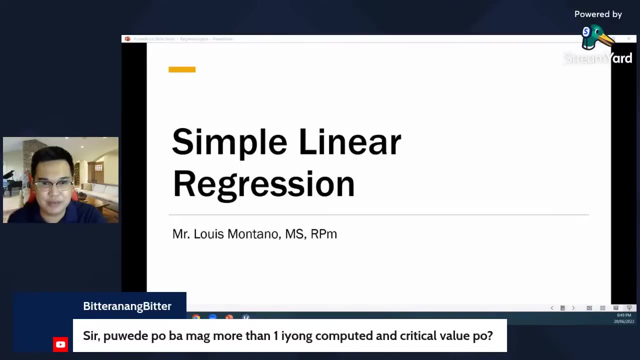 So same yung gagamitin natin na data, pero regression naman this time. Ayan, Sige, at this point we'll be moving on to simple linear regression analysis. Okay, And this is like an extension of correlation. So if you have correlation, 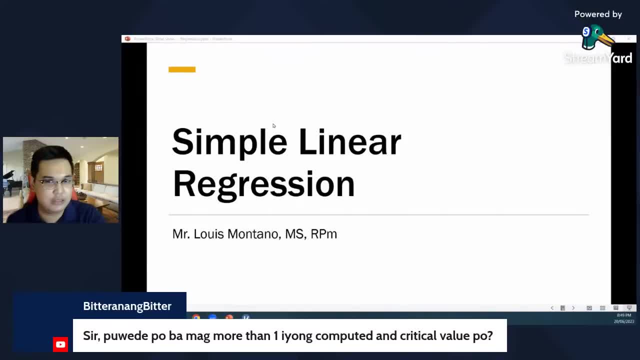 meron ding regression. The difference being correlation is only about answering the question. may kinalaman ba yung dalawang variable sa isa't-isa? Kunyari, kapag bumatalino ka are you more likely to succeed sa trabaho. 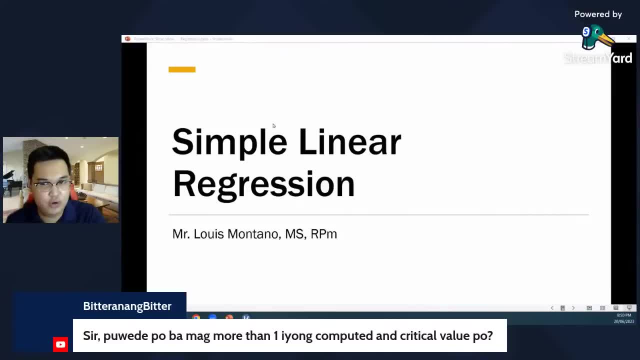 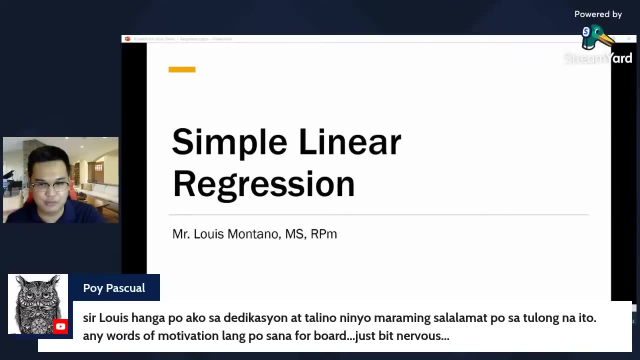 Ganun sa correlation, Pero sa regression you are now making predictions. Okay, You are now making. Okay, Meron daw bang words of wisdom for the board exam. Sige mamaya, may mga isishira akong words of wisdom. 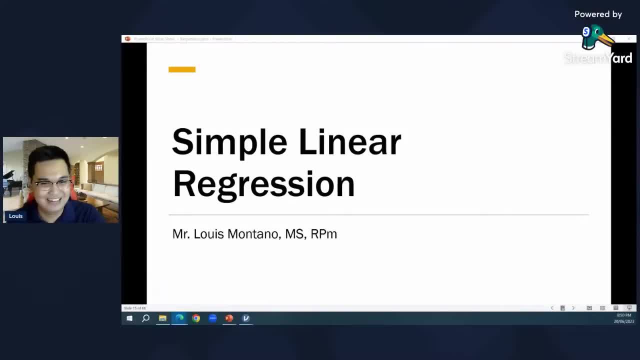 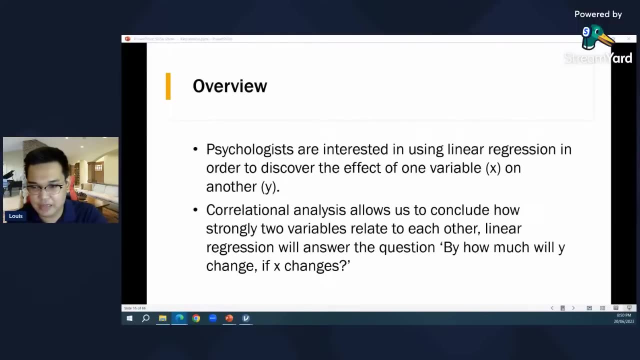 before tayo matapos Ayan. Okay, So sa regression analysis. we use this naman when we are making predictions. Sige, let's start with simple regression analysis. Okay, Very good, The key word in regression is the word prediction. 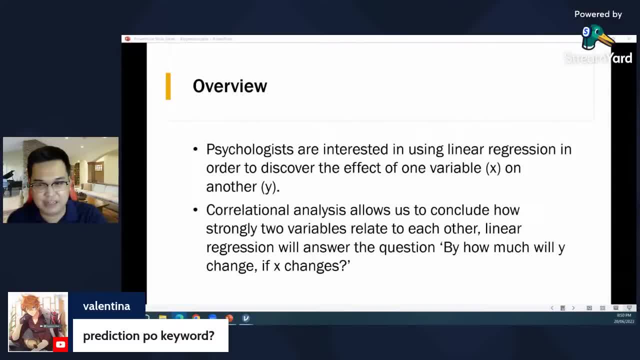 Okay. So kapag prediction ay usapan, it's no longer correlation. You are now making use of regression. So what is regression Ayan tama yan? Correlation is relationship. Regression is more of prediction. Okay, Sige. 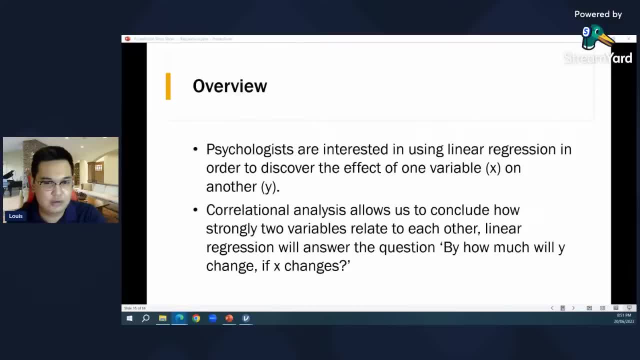 So what is regression analysis? So psychologists are interested in using regression to discover the effect of one variable on another variable. So at that point, parang correlation pa lang siya. Pero how does it differ Kunyari? no may efekto ba yung. 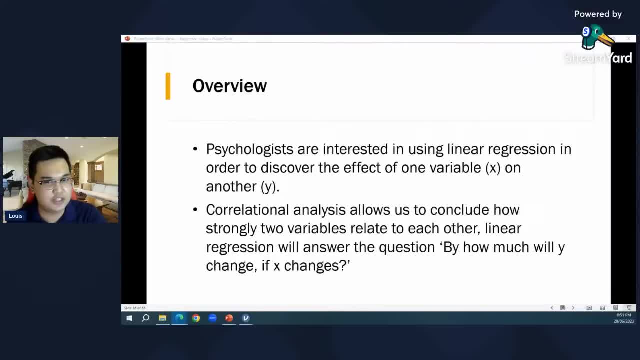 IQ ko dun sa grade ko sa college. Parang ganon, no Mukha pa siyang correlation, Pero ito yung kaibahan nila. Correlation analysis allows us to conclude how strongly two variables are related. Is the relationship weak or strong? 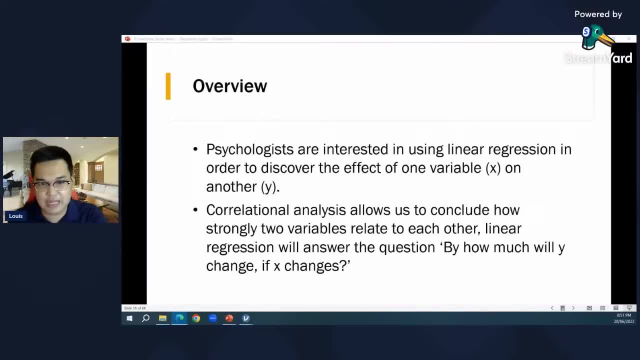 Pero sa regression. regression will answer the question: how much will y change if x changes? Kung kunyari, kung tataas ang IQ mo by 5 points, ilan yung magiging increase sa grades mo You are now making. 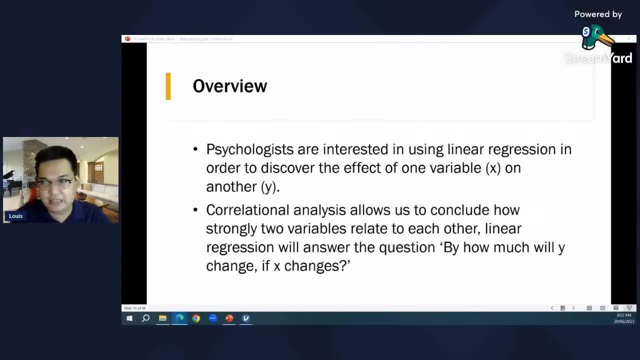 predictions. Kung yung IQ mo is 85,, paano kunyari yung IQ mo maging 90?? How will that affect your grades In business? parang ganito siya, Kung dadagdagan natin yung presyo. 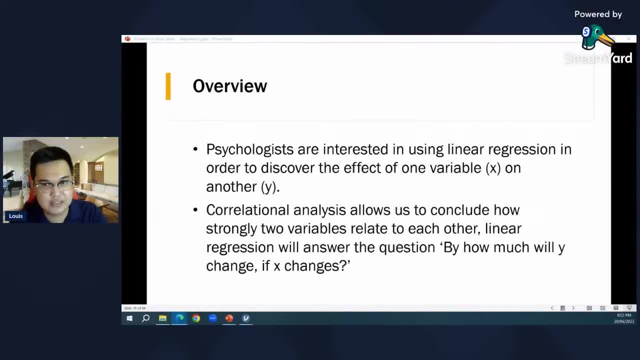 ng piso. how will that affect the sales? Kung dadagdagan natin ng sampung piso, dadami ba yung bibili or kokonte. Okay, So if I change one variable, how will that affect another variable? Yan yung ginagawa natin. 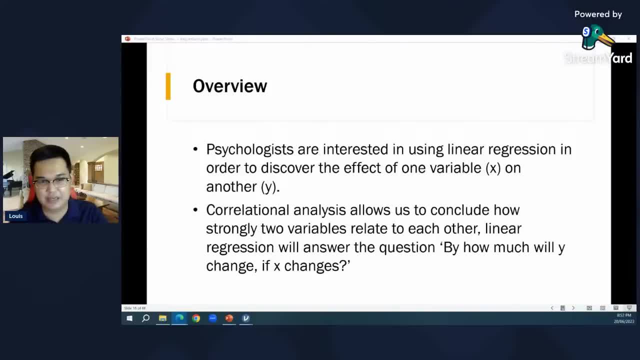 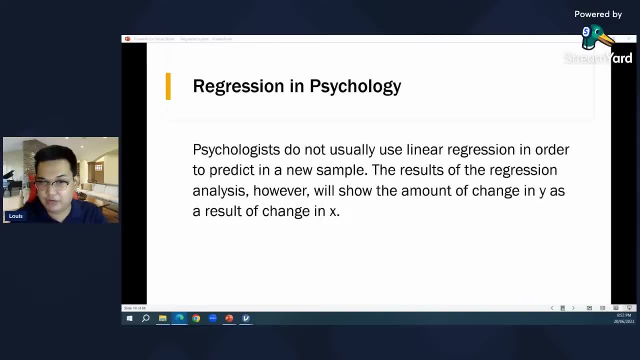 sa linear regression. So paano natin siya i-a-apply sa psychology? Okay, Tatandaan no. But in psychology, even though regression statistically is used for prediction, in psychology hindi natin talaga masyadong ginagamit. 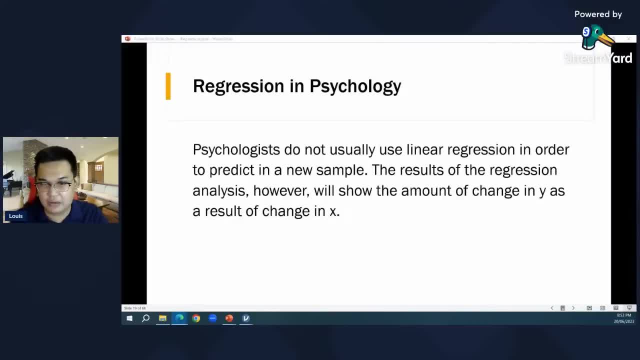 yung regression to predict. Psychologists do not usually use regression to predict. Instead, the results of regression will show the amount of change in Y as a result of change in X, Like what I said sa psychology. hindi tayo nagpe-predict dito, Unlike sa. 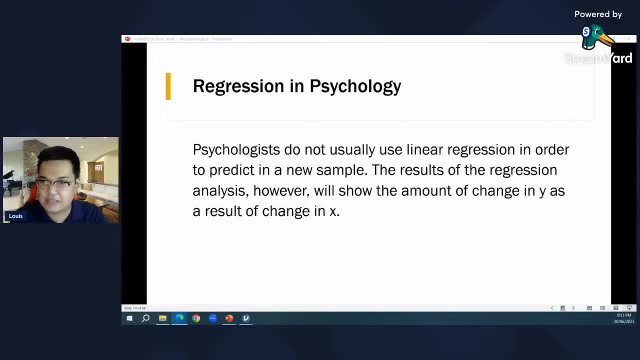 economics, unlike sa business, unlike sa marketing. sila kasi mahilig sila mag-predict. Ipipibenta ko yung iPhone, kunyari ng 60,000, ilan yung bibili, Ganon yung concern nila, Kung may kilala kayong. 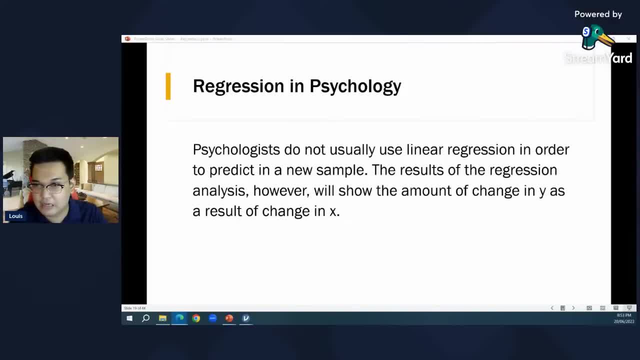 business. major kapatid nyo, nanay nyo, tatay nyo, ganyan nila ginagamit yung regression, Puro sila ang analysis: If ganito yung presyo, magkano yung? 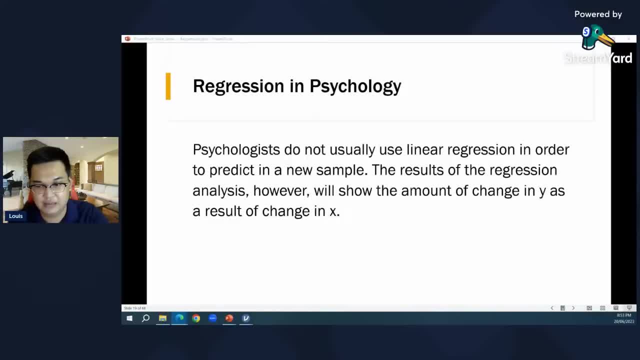 return of investment natin Ngayon sa psychology. we don't do it that way. Sa psychology, tinitingnan natin, instead of predicting ang tinitingnan natin, gano'ng kalaki yung effect Maliit ba. 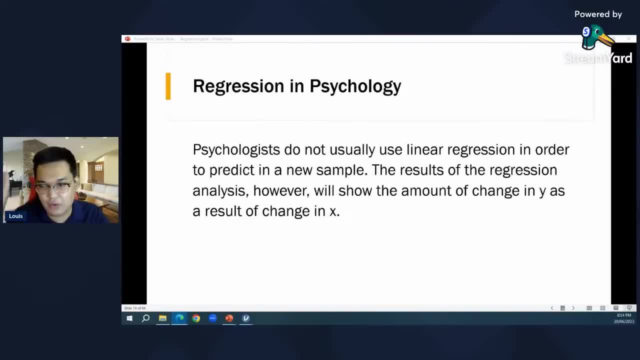 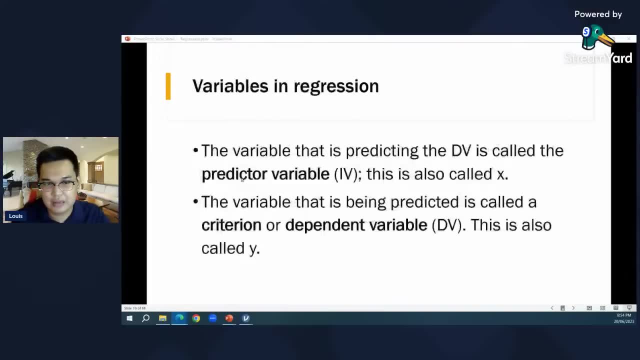 or malaki yung effect? Is the effect positive or is it negative? Okay, So, moving forward in regression, ito yung mga terms natin. The variable that is predicting the DV is called the predictor Si. predictor siya si. IV Siya si. 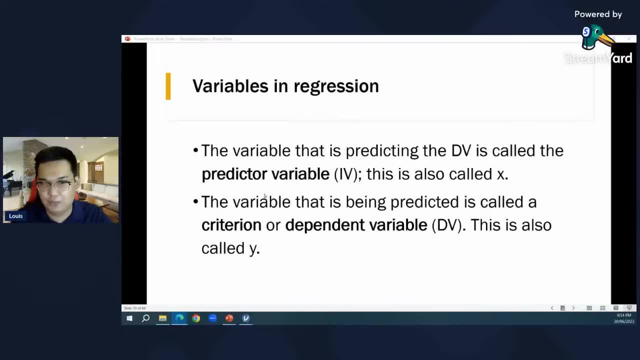 independent variable, Kaya predictor, yung tawag. kasi, going back sa purpose ng regression, we use it for prediction, So ang tawag mo sa IV predictor, We also call it X, While the variable being predicted is called the dependent variable. 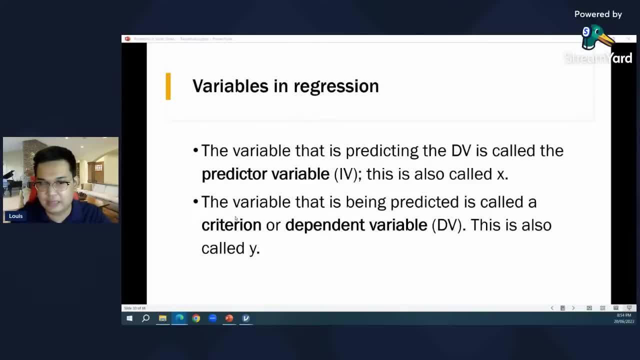 or, of course, the DV, or the criterion. In symbol. we call this the Y Okay, Yan Yan. Like what I said after nito, marire-record siya sa channel ko, So you can go back to it. 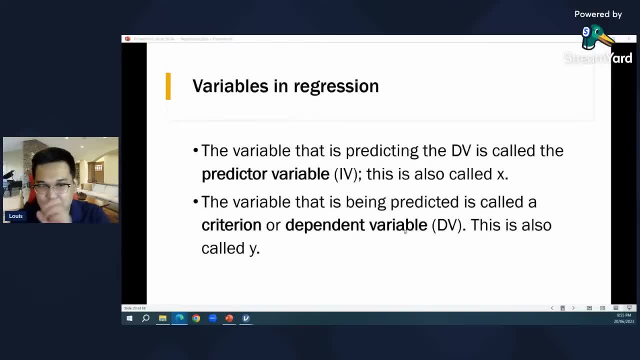 afterwards. Okay Now, so yung nagpe-predict, si predictor, siya yung parang parang lang. ha, hindi ko sinasabing siya yung cost, Siya yung parang cost, While the outcome is. 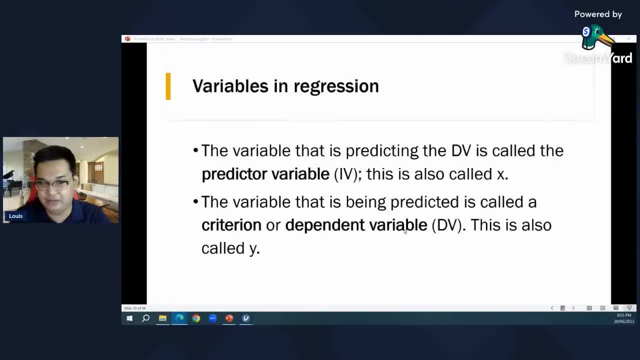 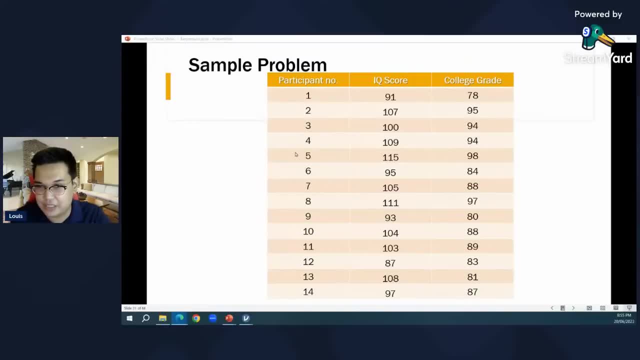 the dependent variable or the criterion. Okay, So babalikan natin yung same dataset. Wala akong binago dyan, It's still the same dataset. So this time titignan natin. Okay, Kapag mamatalino ka. 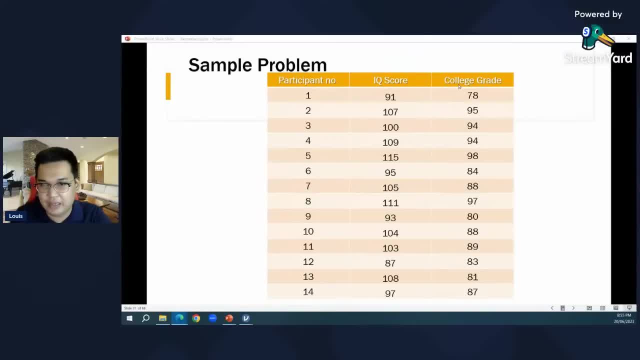 mas mataas yung IQ mo Okay, Mas mataas ba yung grades mo Very good. no, Kaya natin inaaral to Kasi lahat nung dinidiscuss natin will make sense kung ang usapan natin kunyari. 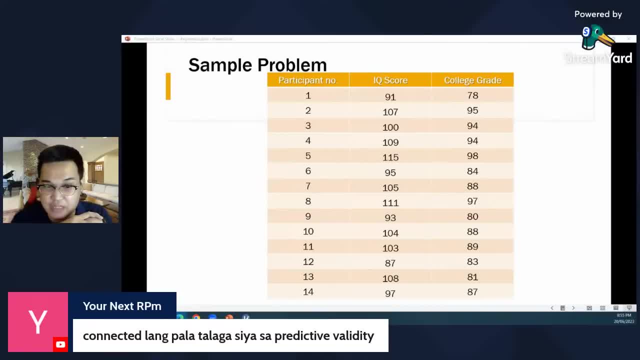 validity. Paano natin masasabing valid yung test? Kunyari predictive validity Di pwede natin tingnan yun bang mga pumasa sa entrance exam. sila rin ba yung mga mataas, yung GPA. 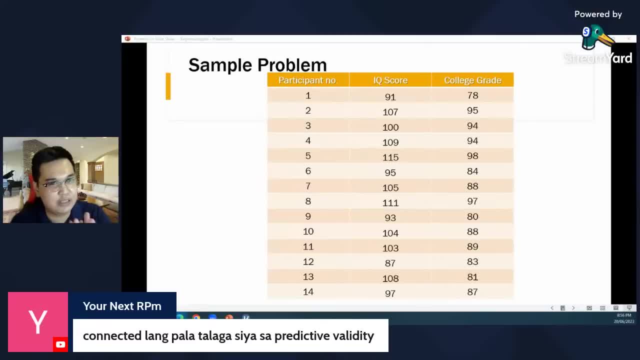 By doing so, you're proving that the entrance exam is valid. That's your way of testing the predictive validity of the test. Ayan, Okay sige Going back. no Titignan natin Kapag mamas matalino ka gano. 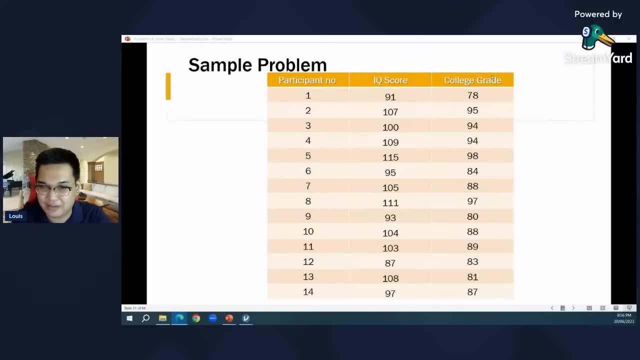 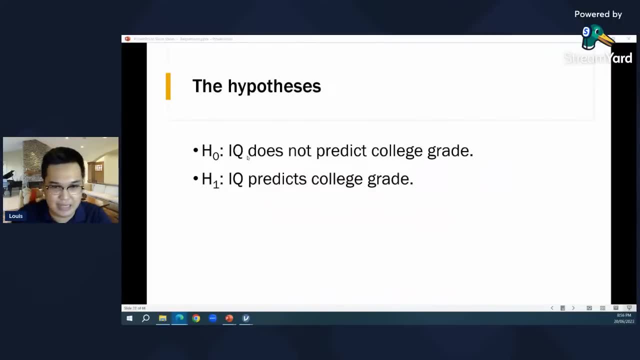 kalaki yung effect nyan sa grades mo. Okay, These are our hypothesis. Our null hypothesis is that IQ does not predict. Hindi na siya correlate. Hindi na siya correlate. Okay, We now use the term predict or not predict. 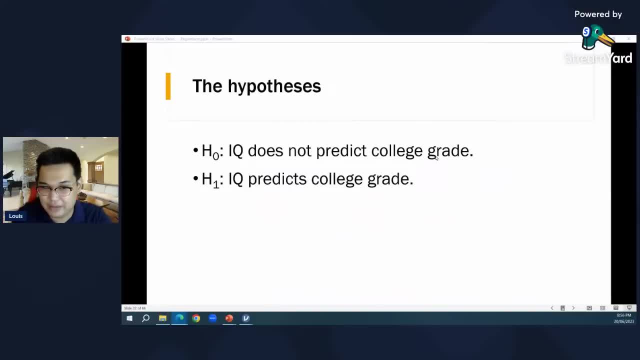 IQ does not predict college grade, while our alternative hypothesis is IQ predicts college grade. So ano kayang ending neto. Which of the two will be true or will turn out to be correct at the end? Is it H0 or H1?? Only di ba. 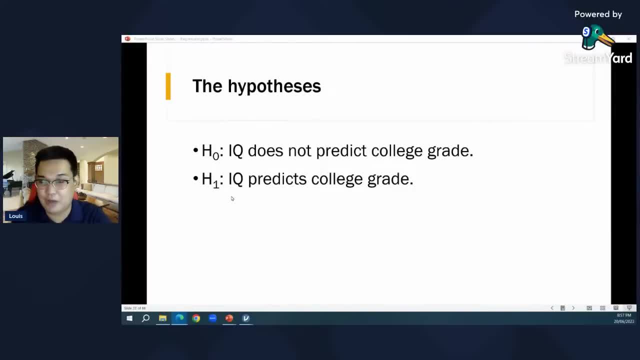 Only the test will tell us what the outcome will be, Pero I think may clue na kayo Kasi nga significant yung correlation, So highly likely pati regression yan magsi significant na rin. Okay, But before we analyze the data, 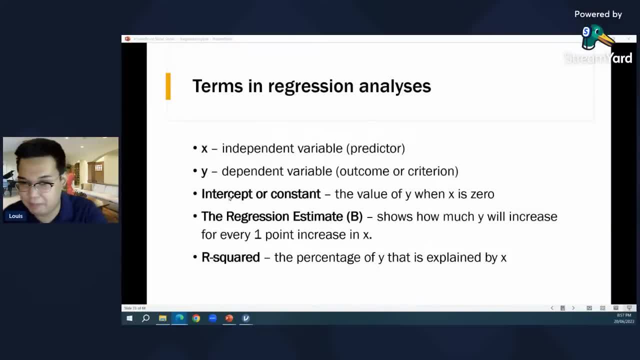 here are the terms to remember. Ang regression: kapag gets mo na siya, madali na siyang intindihin. Pero kapag beginner ka, ma-overwhelm ka. Pero kapag gets mo na siya, ang dali na niyang. 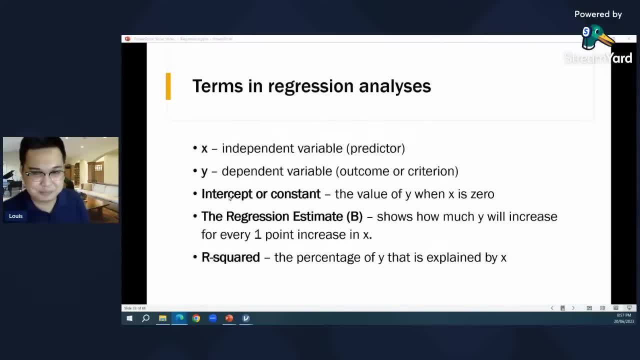 itanim sa utak. Okay, Ang dali na niyang mag-gets. Okay, Okay, So ito siya. no, Ito yung mga terms. So tandaan ninyo: Yung x is the independent. 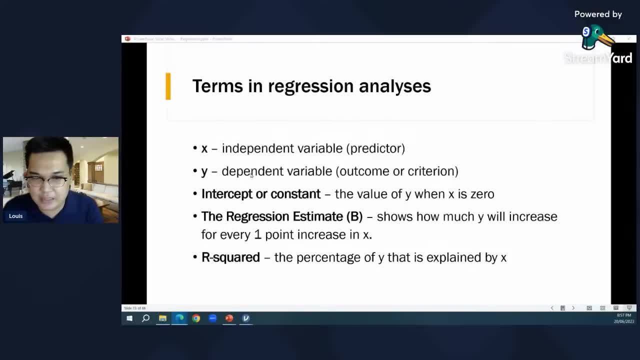 variable nabanggit na kanina. The y is the dependent variable. So sa study natin or sa data natin, yung x yung IQ, Yung y yung grades, Okay, Tapos sa regression, ito yung mga. 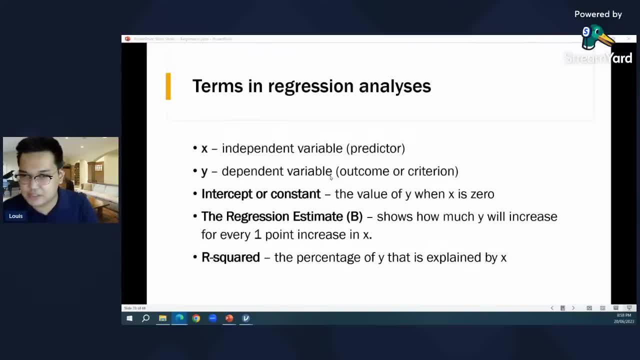 terms na ginagamit. If you check any psych stats book, pati sa psych assessment okay, One of the terms we will encounter is the intercept or constant, Defined technically as the value of y when x is 0. Pero kahit anong stat textbook, 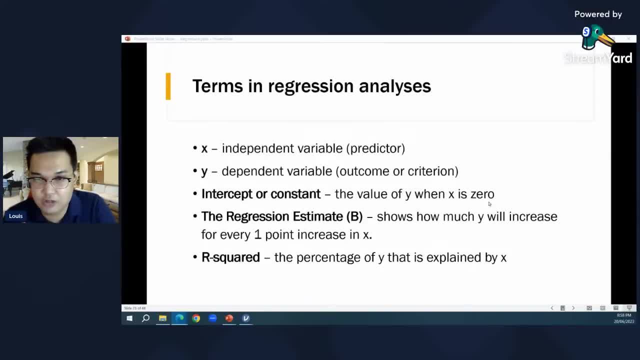 basahin nyo ito yung makikita nyo dyan In psychology. we ignore the intercept. Wala tayong paki sa intercept. Sa psychology Depende sa situation, pero most of the time we ignore that. 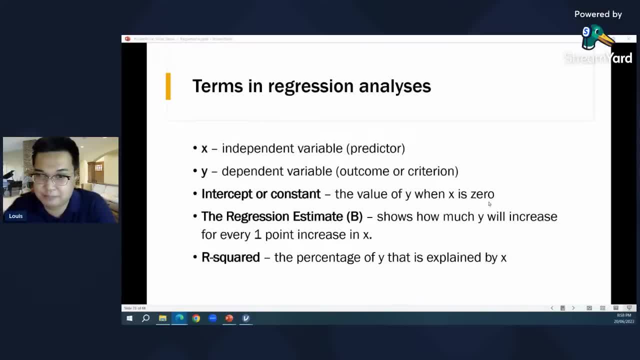 May mga libro nga nilalagyan ng slash, yung intercept, Kasi hindi mo na siya kailangan sa psychology. Pero kung kunyari kapatid mo econ, major, business, major, tinitingnan nila. 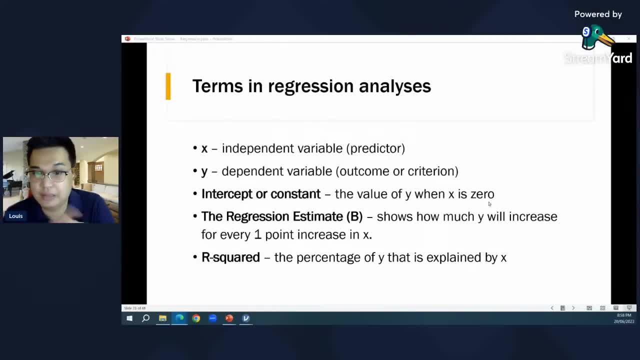 yung intercept The value of y when x is 0. Kunyari ilan ang bibili ng lapis kung ito ay libre? When the price is 0, how many will buy pencils? Ganon sila, Ganon sa economics. 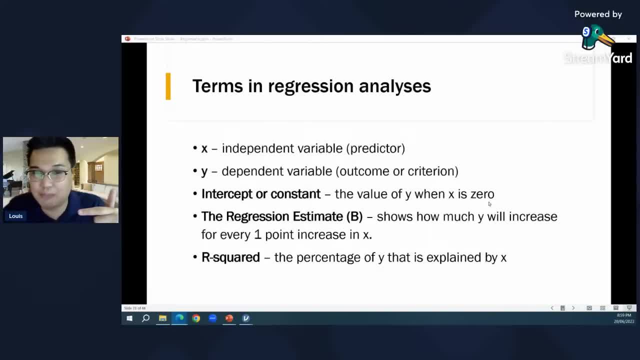 The more nagtaas yung presyo niya. bumaba ba yung bibili niyan Parang ganon. But in psychology we don't care about that. Hindi naman tayong business majors, Hindi naman tayong. 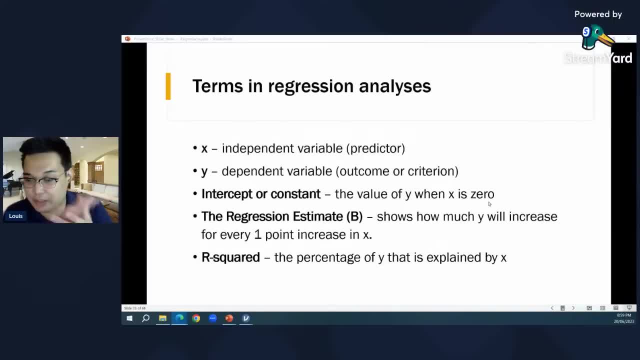 mga econ majors. In psychology, what we care about, nagge-gets nyo ba yung point. Am I making sense? In psychology, what we care about is yung letter B. We look at the regression estimate. The regression estimate. 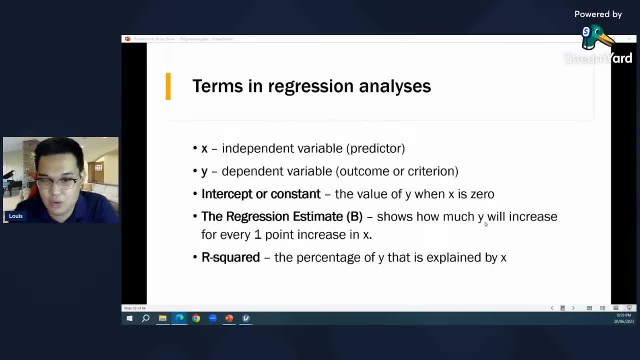 this is what we care about. It shows how much y will increase for every one point increase in x. Okay, So yung regression estimate, ito yung effect. Gusto natin malaman. malaki ba yung effect, Maliit ba yung effect? Wala. 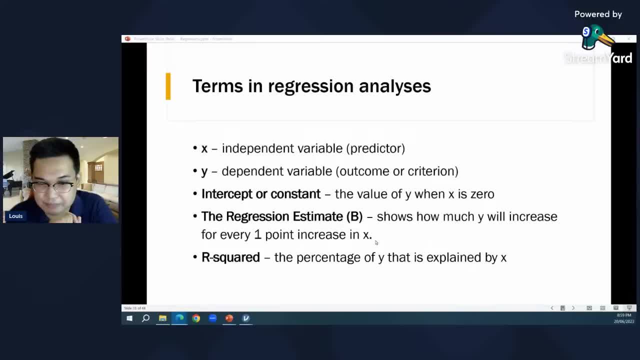 bang effect. We look at the regression estimate And another thing that you usually see in the textbook, pati sa site assessment, is the r-squared. The r-squared is ilang percent nung outcome variable mo yung ine-explain nung x. 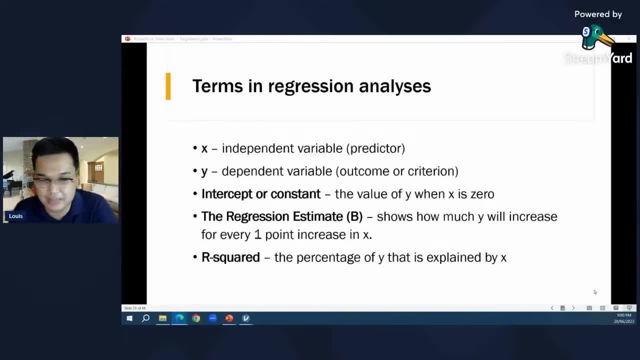 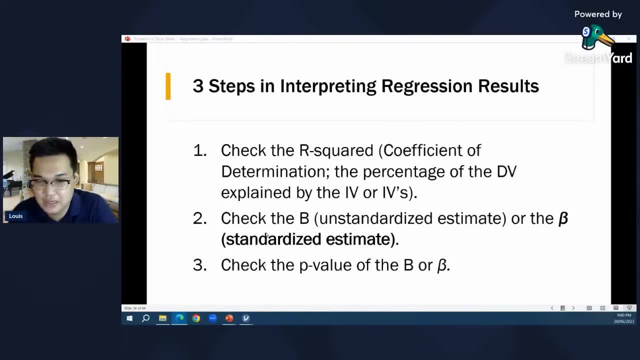 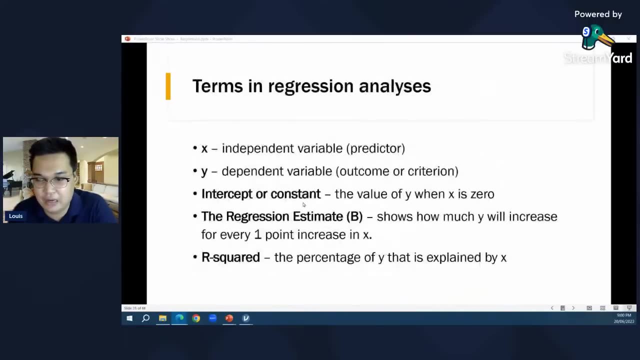 Lahat yan makikita natin when we do the analysis. And here are my three steps in interpreting regression results. Okay, if you followed these three, hindi iba yun, Iba yung ay tama yun. 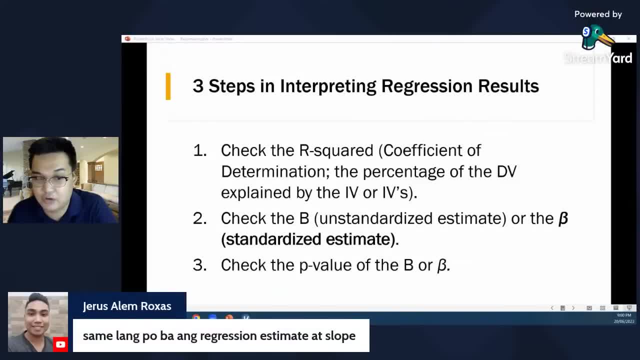 Tama ito Nasa isip ko constant. This is correct. Jerusalem Or Jerusalem. Hindi ko alam kung iwalay ba yung pangalan mo or iisa, lang yan, Tama yan Jerusalem. The slope is the regression estimate. 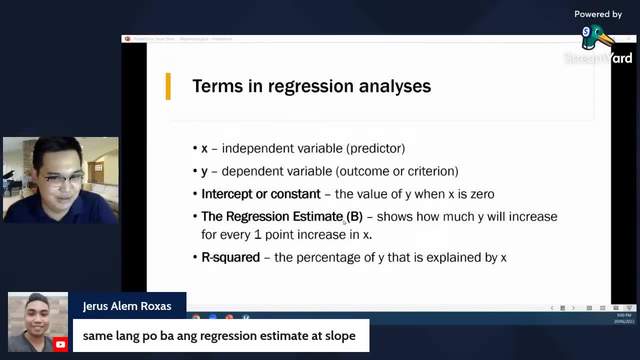 Okay, I don't want to be a math nerd here, pero the more na steep yung slope, the more na malakas yung effect. Ganun siya, Pero the slope is the regression estimate. Tama yun. 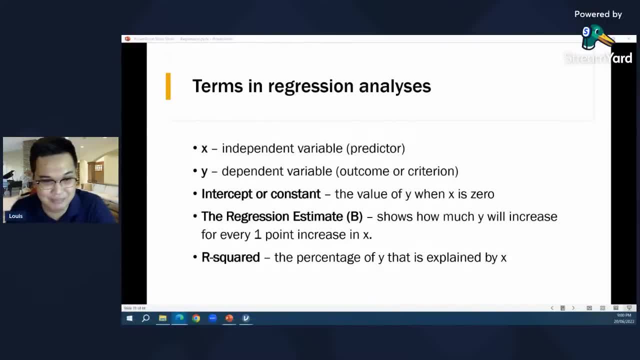 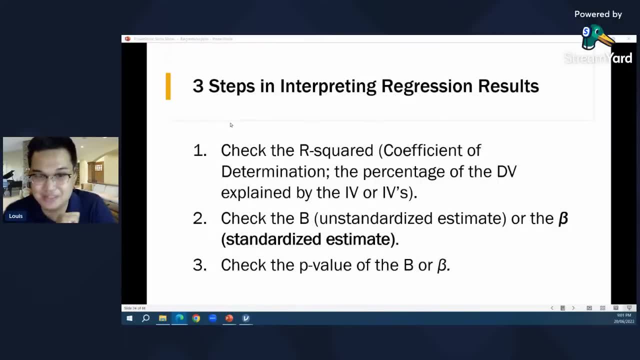 Tama yan. Jerusalem and Alem talaga. Okay, Sige, tawagin kitang Jerusalem. Okay Going back. So ito yung three steps. Kapag mag-i-interpret ka ng regression, ito yung titignan mo Una. 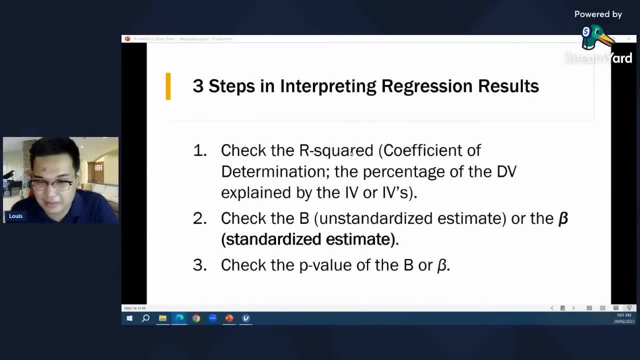 tingnan mo yung r-squared. Okay, Gano kalaki ng percent nung y. ine-explain nung x. Okay, How much of the y is explained by x? Malaki ba Maliit lang. Okay, Naalala ko lagi. 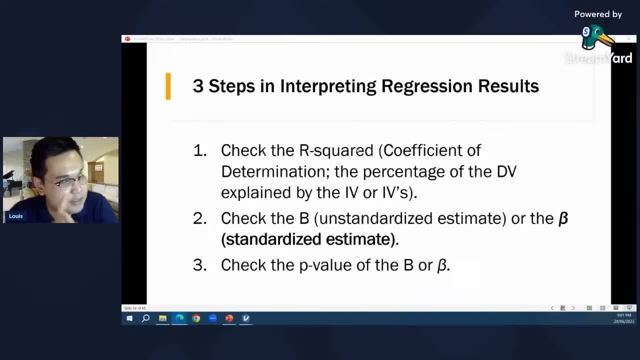 example ni Mam Meryl dyan, Sixty percent of brain development of the baby comes from the mother O para siyang r-squared. Ilang percent nung brain development ng baby yung galing sa nanay. Sixty percent. 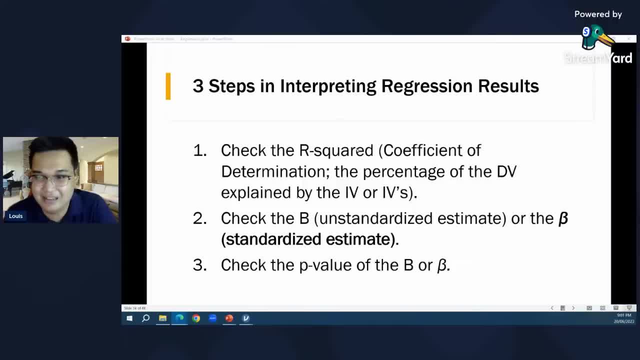 Parang ganun yung r-squared Makikita natin yan later Pangalawa, after you check the r-squared pangalawa. by the way, kulang explanation ko If sixty percent comes from the mother. 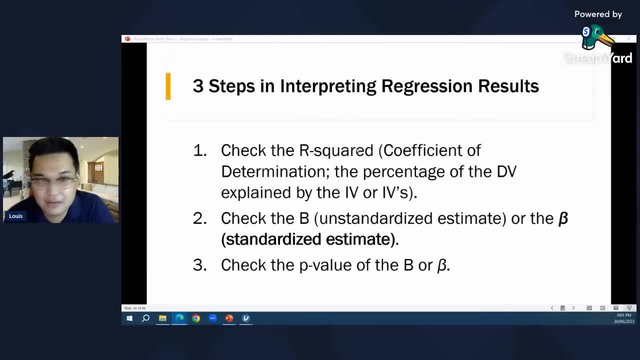 the remaining forty percent, hindi natin alam kung saan galing, In statistical terms, yun yung error? Okay, Sixty percent of your outcome is explained by the predictor, While the remaining forty percent okay. hindi natin alam where it's coming from. 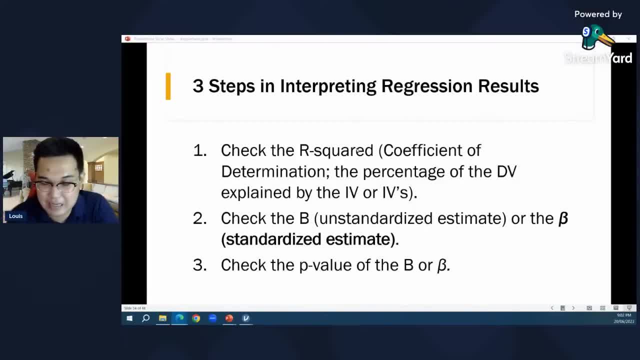 So yun yung number one, the r-squared. Basically, the bigger the r-squared the better. Okay, Kasi, the bigger the r-squared meaning mas nape-predict ni Ivy si Dee Ayan Pangalawa. you look at the. 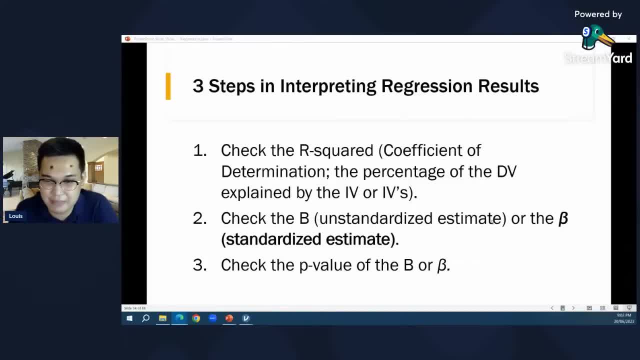 b. you check the b, the regression estimate, or you can also check the beta, Ang basa dito: beta Yung b na italicize yung b na Greek. you call it beta Ang kaibahan nung b. 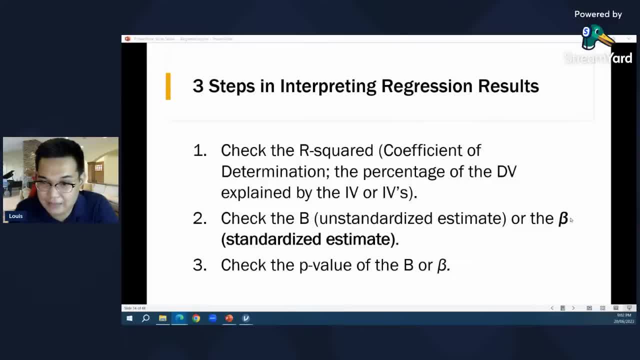 sa beta, yung b? r-score, yung beta z-score. So yung tanong ko sa inyo: ano dyan? kaya sa tingin nyo, yung mas magandang interpret? Most of you are reviewing for the board exam. 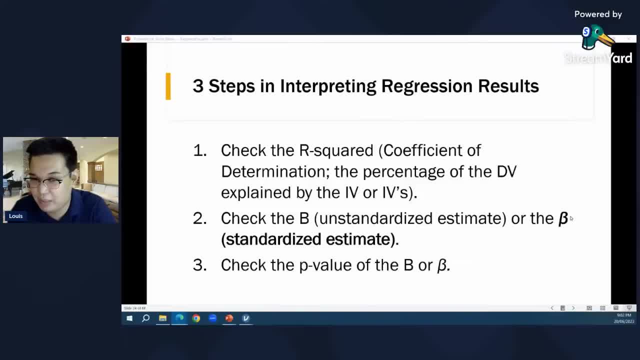 Do you think it's the b or the beta? You can type the word beta if you can find the symbol beta. Which of the two do you think is mas accurate i-interpret? Do you think it's the b or the beta? Kasi yung b? r-score. 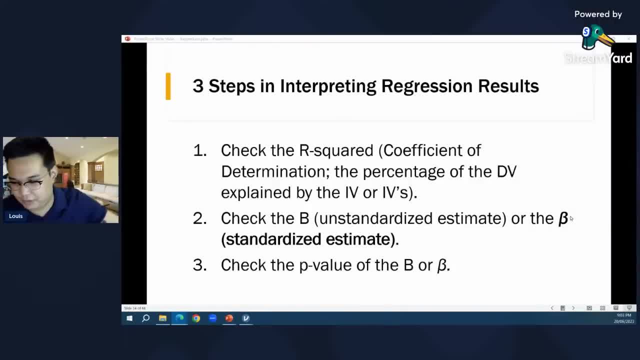 yung beta, z-score yan, Ayan, We can use either, Pero mas accurate yung beta. And finally, number three, just like in correlation. yung last na titignan mo is significant, ba by looking at the b value. 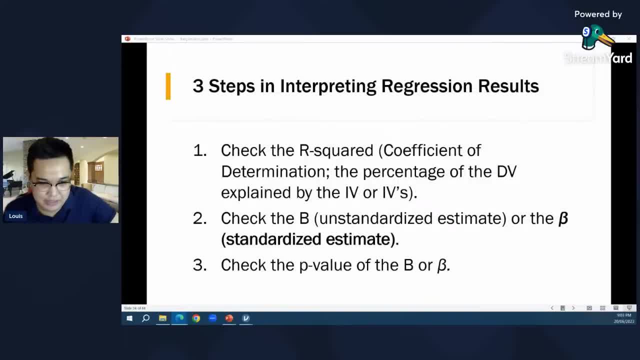 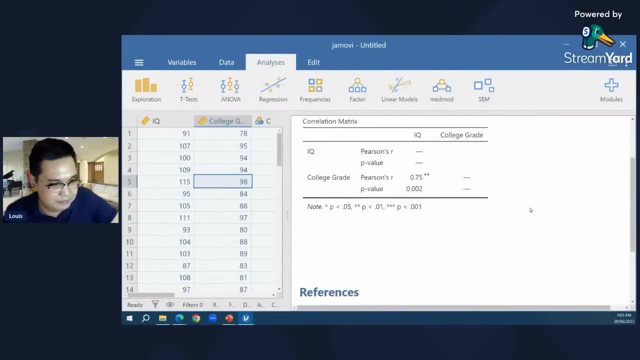 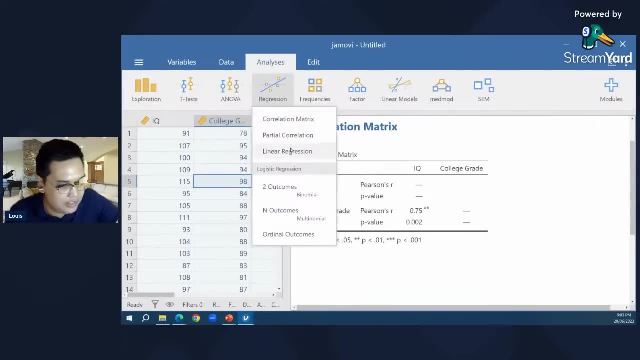 Ayan, Very good Results na pala yung next Sige mag-analyze tayo. Here's our data set once again. So to run our regression analysis, let's click on regression. Let's click on linear regression. 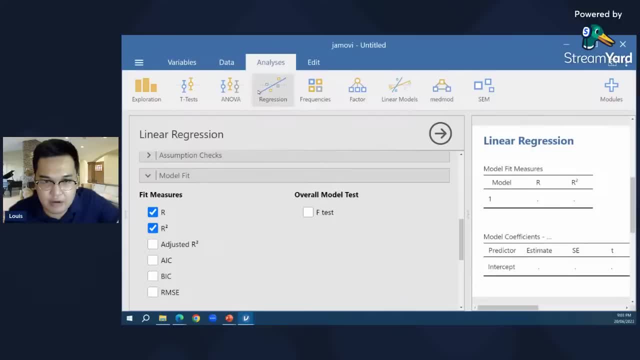 Ulitin ko. no, Ang ginawa: kinlik ko yung regression, tapos kinlik ko yung linear Ayan. So kung correlation, correlation lang, Kung linear regression, ito yung i-click mo: Linear regression. 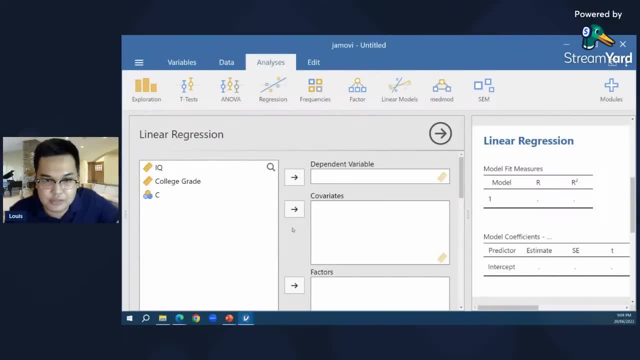 Okay, Tapos, yung outcome variable mo, which is yung grade, ilalagay mo siya sa dependent variable, While yung predictor mo ilalagay mo siya sa covariate. Okay Tapos, bago mo tingnan, 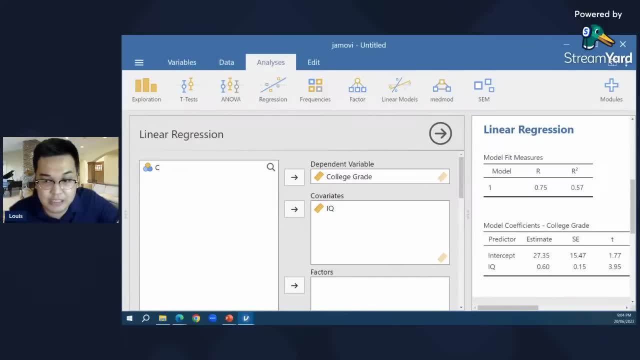 ano po yung b, yung b, yun yung regression estimate. Oo, yun yung regression estimate. While yung magandang b, yung italicized beta, Na beta. siya, Yun yung basa. 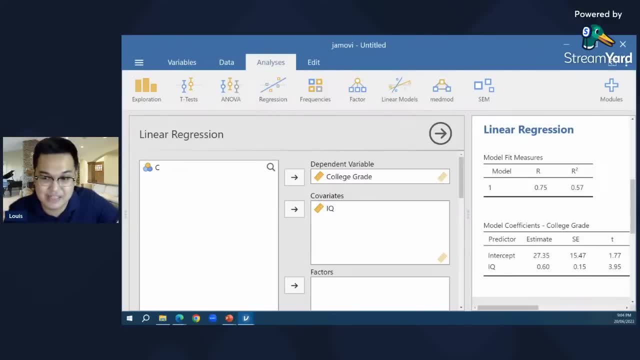 dun Greek letter yun. Tapos yun naman standardized estimate. Okay, The b is regression estimate, While the beta, the magandang b ano, the beta is the standardized estimate. Tapos parang mag-scroll. 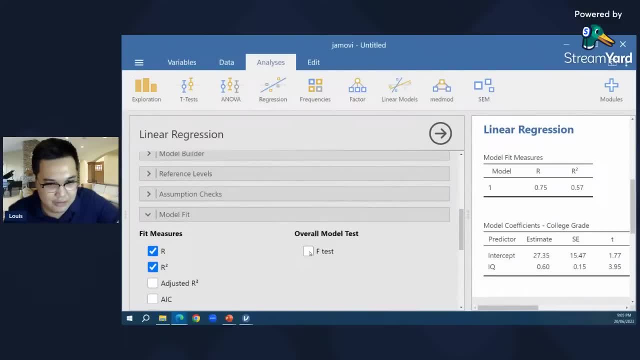 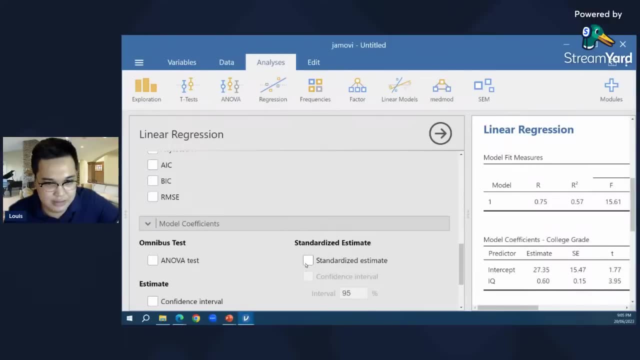 down lang ako a bit sa left may mga iti-check lang ako no, The F-test, And para makita yung beta, iti-check natin tong standardized estimate. Kasi yung nandito raw score lang yan, Gusto natin gawing z-score. 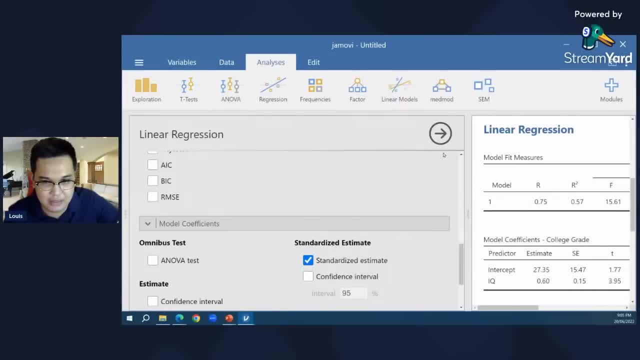 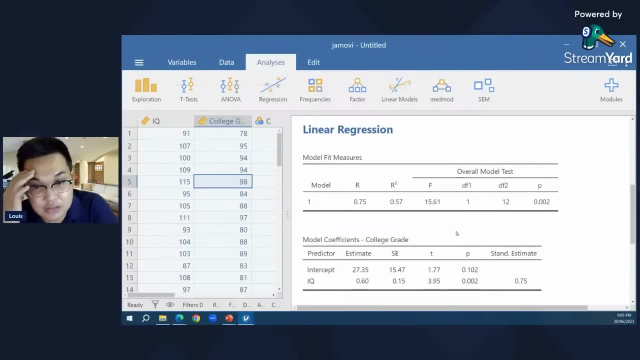 Iti-check natin yung standardized Ayan. Tapos ito na yung result. Diba Nakaka-overwhelmed pa siya at first, Parang sir ano, titignan ko dito spit sa ulo Anong unahin ko. 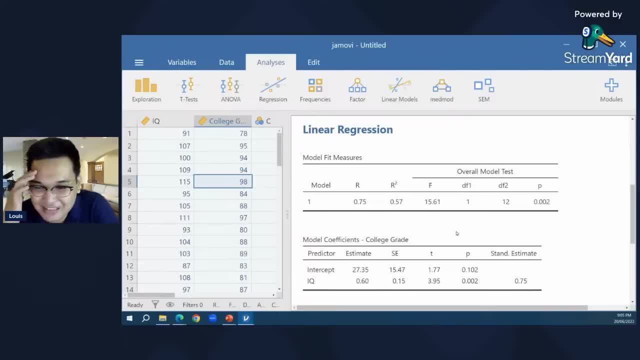 dito Anong unahin ko dito Ang dami. Makinig kayo mabuti, Sabihin ko sa inyo ano unahin niya dyan. Okay, Pero isa munang papansinin natin. Look at the R. 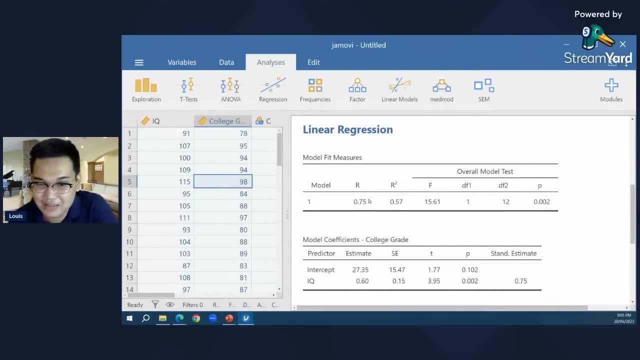 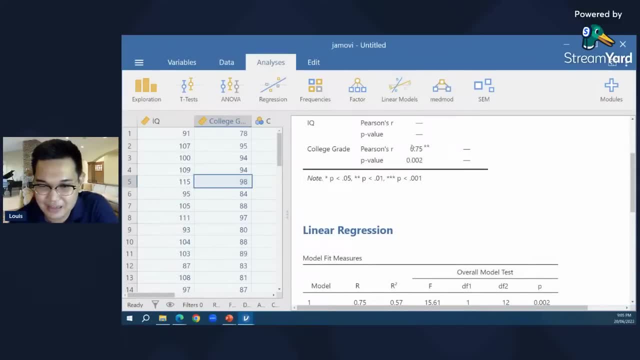 Yung R na yan. yan yung correlation ni IQ tsaka college grade. Kung mag-scroll up tayo sa taas, tingnan niyo The R that we got kanina is just the same as this one Diba. 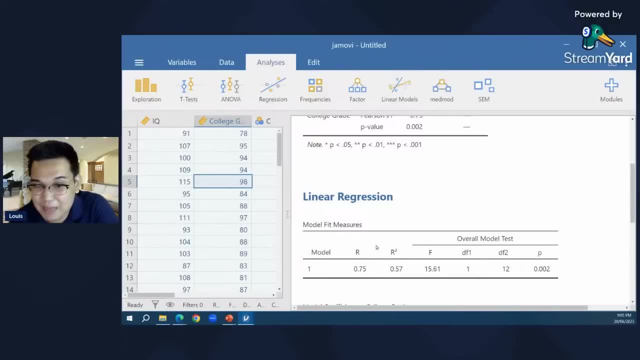 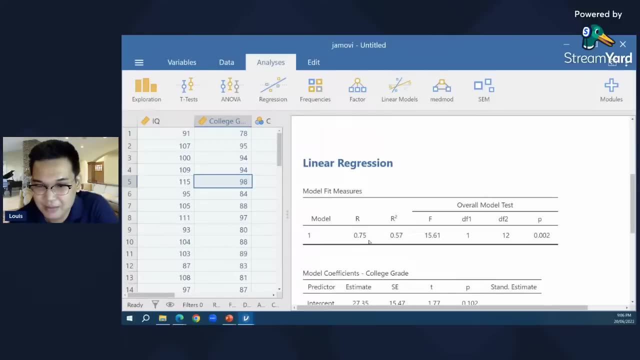 Diba. Same lang sila Ngayon. paano naman yan naging R-squared? Paano yan naging R-squared Yung .75, minultiply siya sa sarili niya, Inisquare siya. 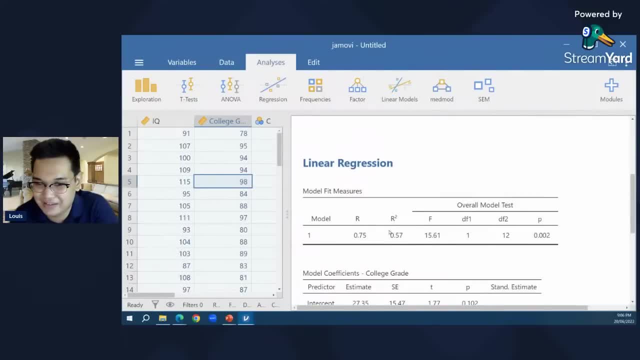 Doon, siya naging R-squared. Doon, siya naging R-squared. Ayan, Okay, Sir paano natin interpret yan Sige, interpret na natin. Sir, paano natin interpret yan Sige, interpret na natin. 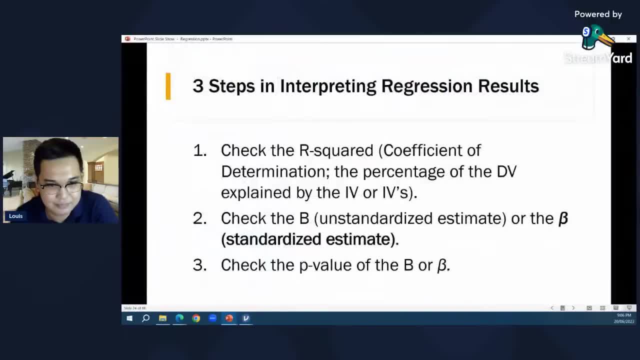 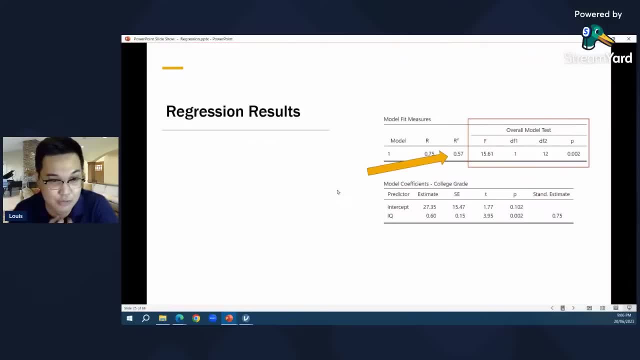 Balik tayo sa PowerPoint. Isa-isahin natin yung himay-himayin natin na parang manok na kinakain, Para hindi tayo mabulunan. First step, Tingnan natin yung R-squared. 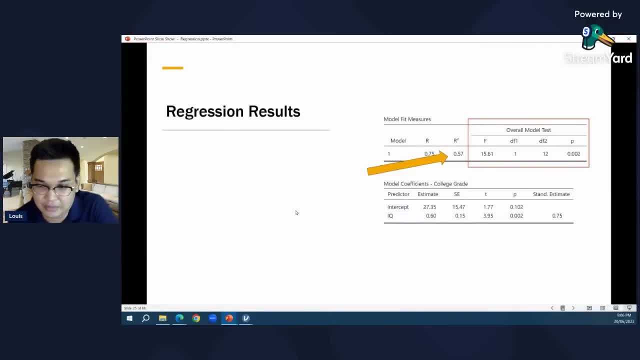 .57. Anong meaning yan. Anong meaning yan Remember the R-squared. by definition, the percentage of the D be explained by the IV. Ilang percent nung grade mo nung college. ini-explain nung IQ mo. The interpretation is: 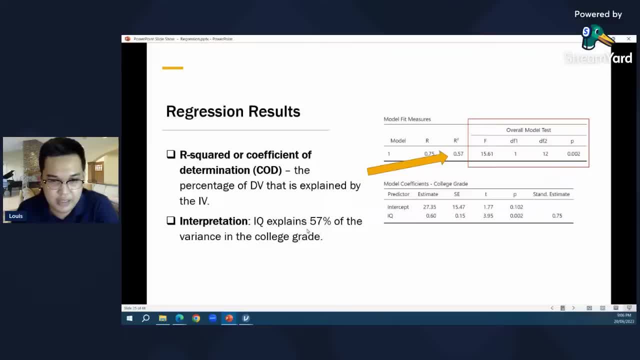 The interpretation is: The interpretation is 57%. sorry, IQ explains 57% of the variance in college grade 57%. okay, nung grade mo nung college ang ipinapaliwanag nung IQ mo, Malaki-laki yan. 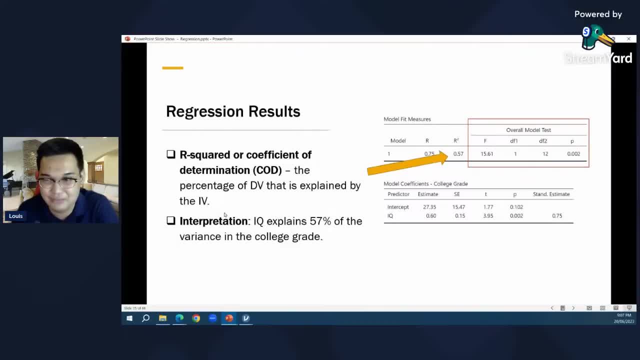 Okay, malaki-laki yan. Again, 57% of your grade is explained by your IQ. The remaining 43 comes from other predictors or other factors. Ano, kaya yung other factors Pwede kung masipag ka ba, Kung hindi ka ba uma-absent. 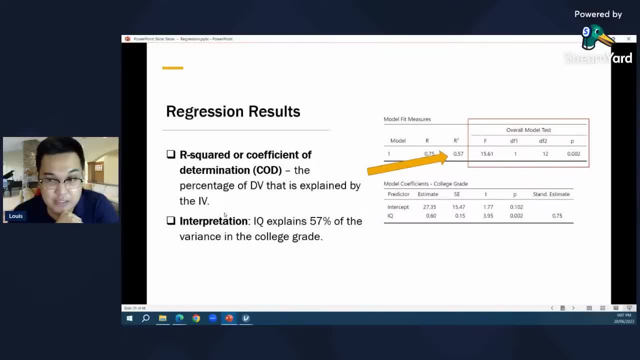 Kung lagi ka ba nakikinig sa teacher mo. Pero 57% of your grade is explained by your IQ. So basically, the smarter you are, the higher your grades will be, At least according to the data. Okay, And sir paano. 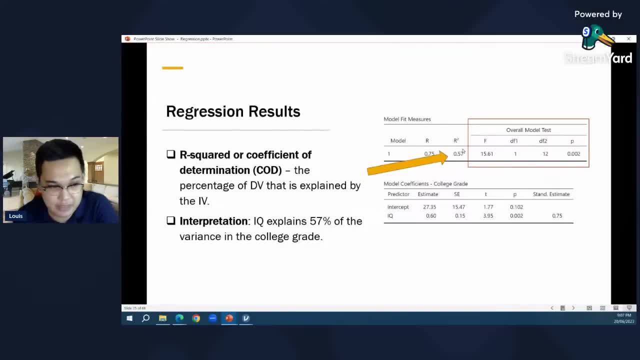 natin malalaman kung yung 57% na yan ay significant or not. Kung makikita nyo, sa kanan there is what we call overall model test. Yan yung nagsasabi sa atin Indicates if. 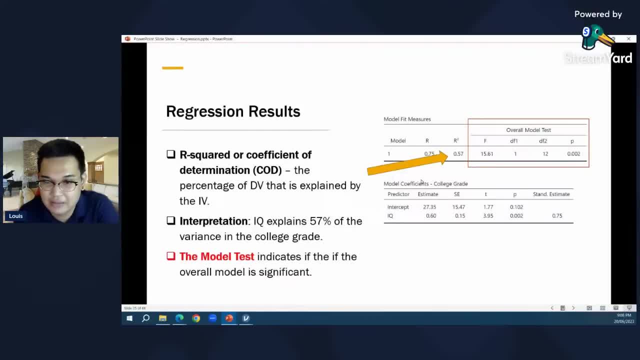 da na doble. no, If the model is significant. So if titignan natin yung p-value diba Maliit lang lower than 0.05.. Meaning significant yung r-squared natin. 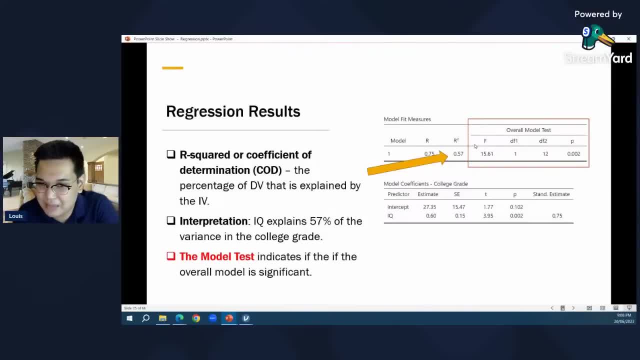 Yun yung interpretation niya. Kapag nagsignificant yung r-squared, pag tumingin ka sa baba dun sa model coefficients, mag-expect ka na significant din yung results. Okay, So that's for the r-squared. May tanong kayo sa r-squared? 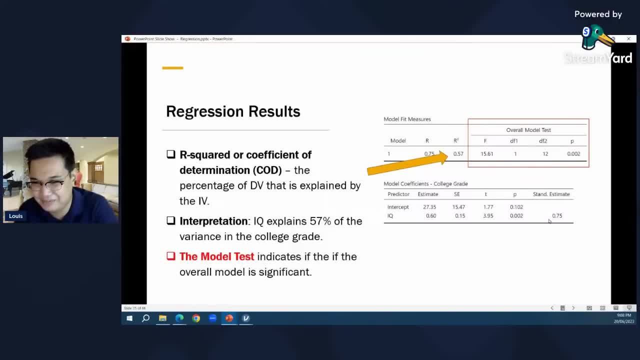 Or nagets ba yung r-squared. Nagets na ba yung r-squared? Kung may tanong, kayo sabihin nyo lang along the way, para before ako mag-move on. So yan yung r-squared, Once again: 57%. 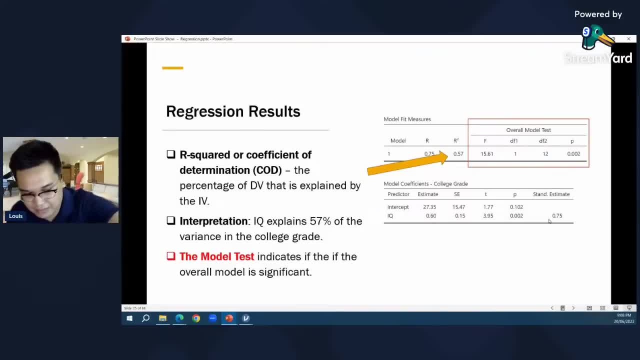 of the DV is explained by the independent variable. Right Ngayon, step 1 is the r-squared. Step 2, you look at the regression coefficient And sabi nga natin, kanina, it's better to look at. 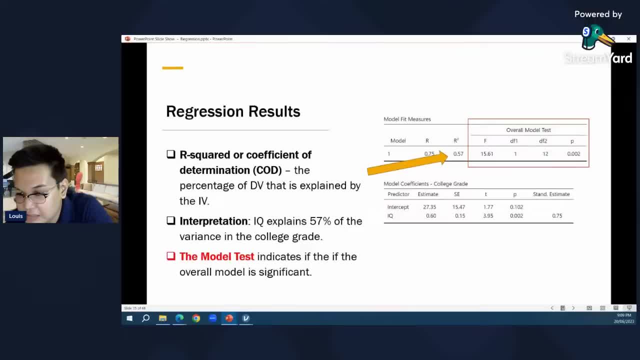 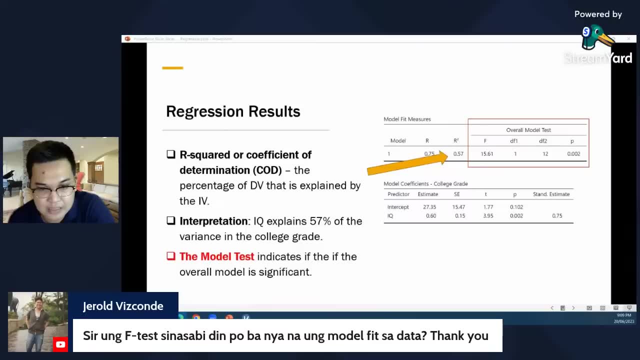 Okay, Tama yan. no, That's a good way to say it, Gerald. Tama ito, Tama ito, no. Yung F-test po ba na sinasabi nyo yung model fit Very good. 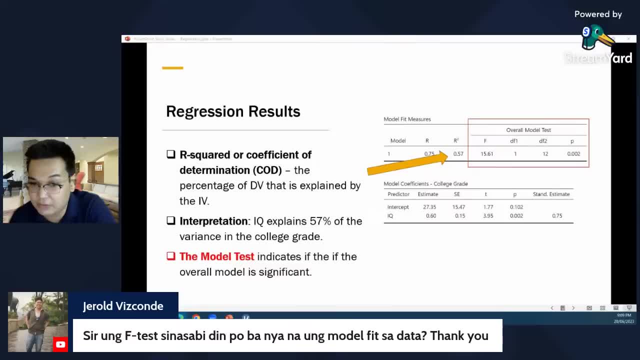 Okay, Ayoko maging technical, kaya hindi ko siya ginamit, Pero very good Siya, yung model fit Okay. So in technical terms, kapag significant siya meaning maganda yung statistical modeling mo. 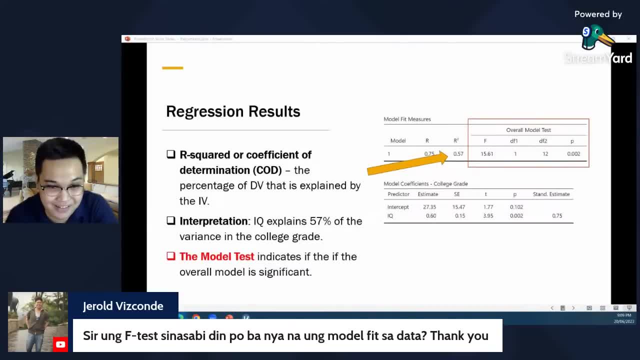 meaning nagwo-work yung formula mo. Tama yan? no, Correct yan. I agree with that, Gerald. no, It's the model fit coefficients, Kapag hindi nagsignificant yung p-value ng r-squared mo. 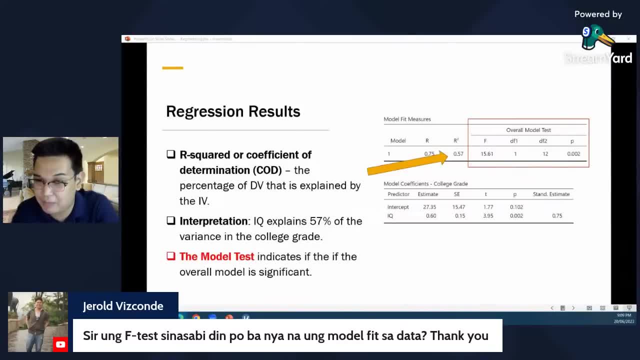 ang ibig lang sabihin yan: huwag ka na mag-expect na may effect yung mga variables mo. Okay, Nangyayari yun kapag sobrang baba, nung r-squared May research kami ngayon yung. 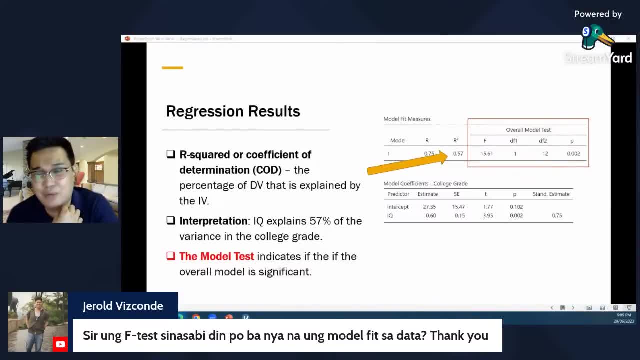 r-squared, May iiyak ka na lang, eh. 0.05, 0.07.. So yung mga variables namin walang effect. Yun yung nakita namin, Yun yung napansin namin. 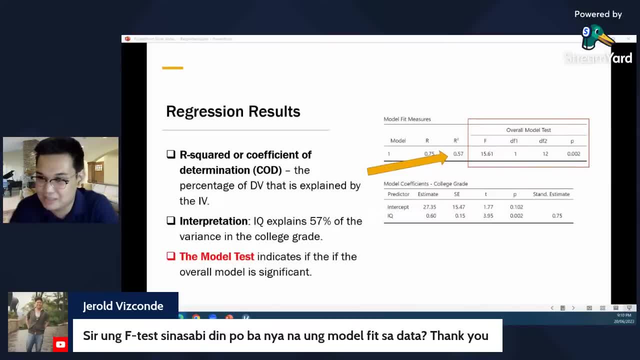 Nakakaiyak lang yung r-squared. So kapag wala kay r-squared mo, it means talagang. okay, this is correct, It's the goodness of fit. Okay, It's the goodness of fit Yan. 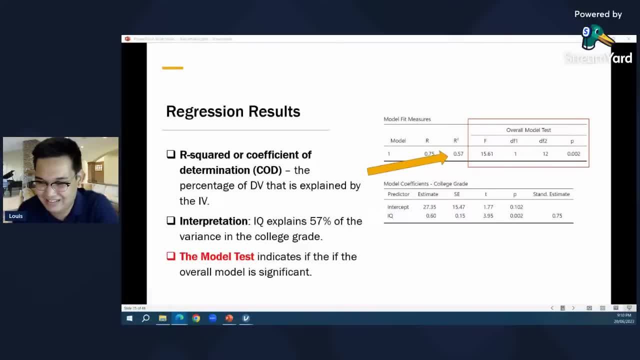 It's the model fit, It's the goodness of fit. Yan Okay, Kami nato, nagagandahan kami sa r-squared kapag lumalagpas na siya ng 0.10.. Medyo pangit kapag sobrang liit. 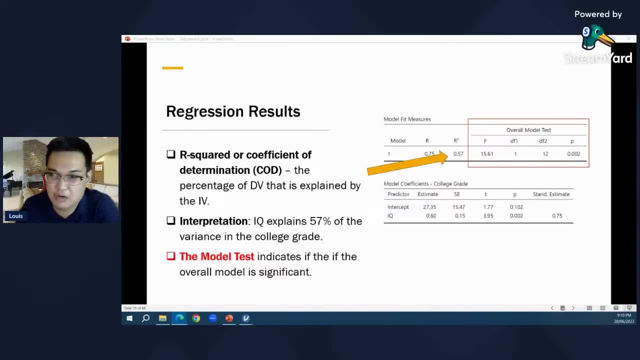 yung mga 0.01, 0.02.. Okay, Medyo ano na yun. Questionable na yun Sige. Step number two: You look at the, you look at the individual effects of the variable, You intercept. 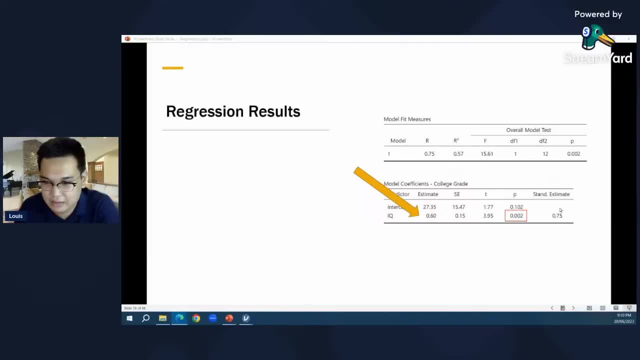 yung first column, first row pala. Okay, Yung model test, no Yung model test. ang sinasabi sa atin ito is: kung talaga bang may effect yung predictor or predictors mo kung marami. 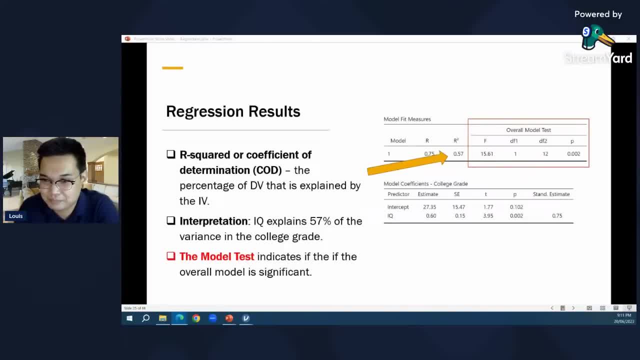 Dito um ibig sabihin na ito talagang yung napili mong predictor, talagang may impact siya on your outcome variable. Basically, that's what the model test is telling you. Okay, If the r-squared 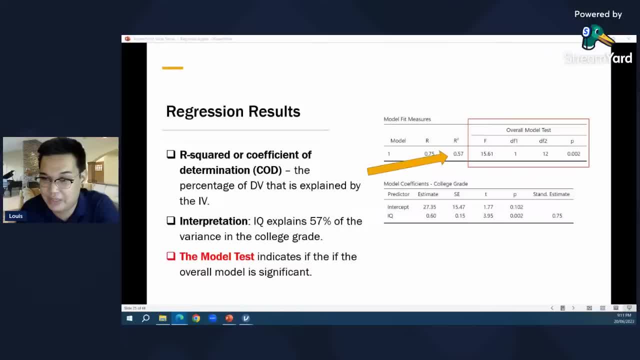 is significant or not, Kung may effect ba talaga yung variables mo or wala. Yun yung sinasabi sa atin ang model test. Kapag yan hindi significant, tapos kapag sobrang baba ng r-squared, it means yung variables mo. 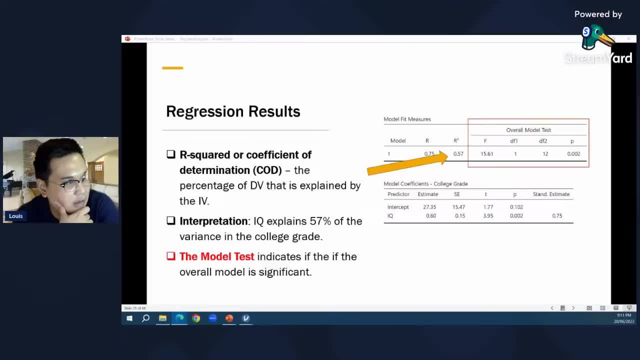 walang effect Kunyari, no Kunyari yung mga mataas sentence exam. not necessarily sila yung gumagraduate ng college, Meaning walang effect yung score mo sa entrance exam sa college, success mo. 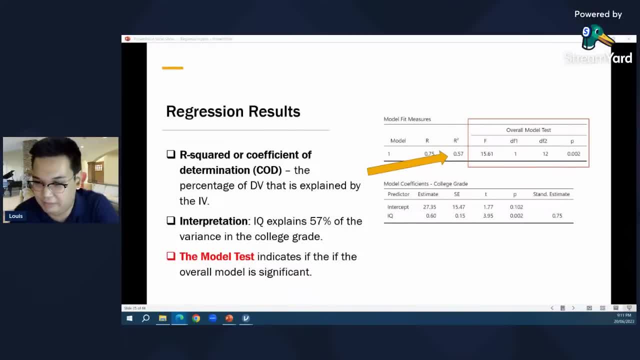 Yun Pangit, yung model fit. nun, kapag gano'n Hindi siya significant, Okay, Pero sa psychology you know what we're interested with. It's not really um, it's more of the second part, Ito na inidiscuss ko. 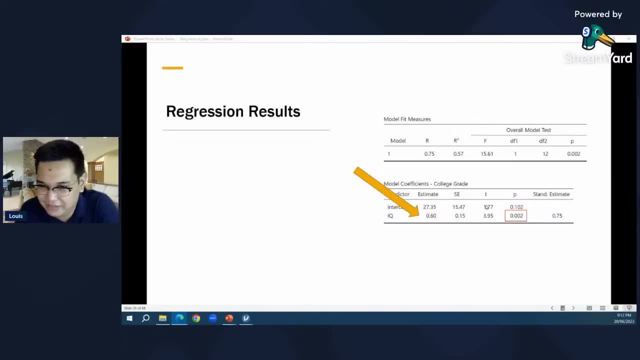 ngayon. Okay, yung intercept, just ignore it. Okay, We don't talk about the intercept in psychology, Pero in business, yes, pinag-uusapan siya Dati may client ako econ major, mahalaga sa kanila yung. 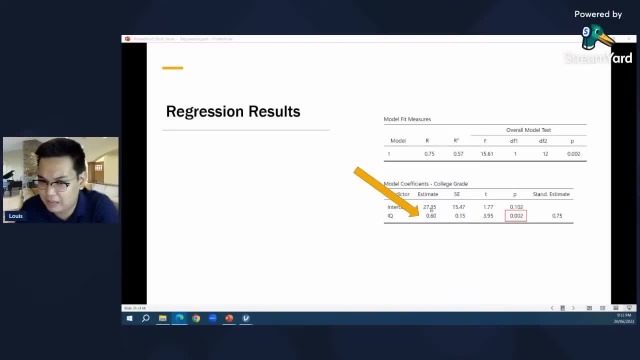 ano yung intercept Kasi ausapan nila pera eh GDP ganyan. May client ko dati yung study niya GDP Mahalaga sa kanila yun. Pero sa atin iba kasi yung gamit ng psychology sa. 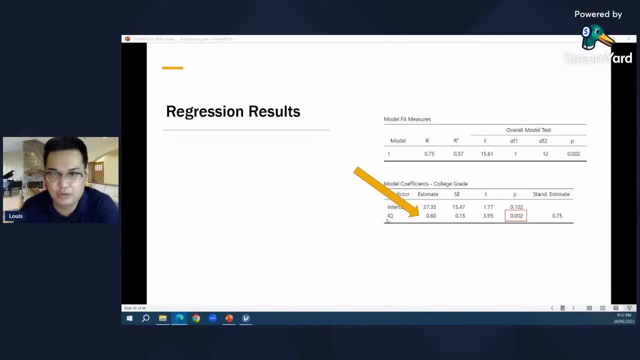 regression. eh, It's more of gano'ng kalaki or kaliit yung effect. Ganon tayo Ngayon may effect ba yung IQ dun sa college grade mo, Yung R, ay sorry, hindi R. 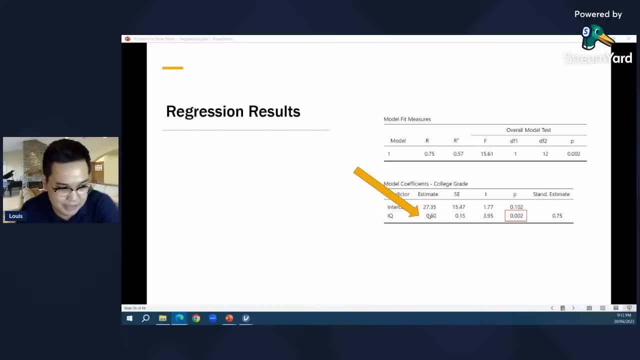 Yung B in this table is the estimate Yung point 60. Okay, How do we interpret that? The regression estimate tells us the amount of increase in the DV for every one point increase in the IV. So ano, ulit, sir. 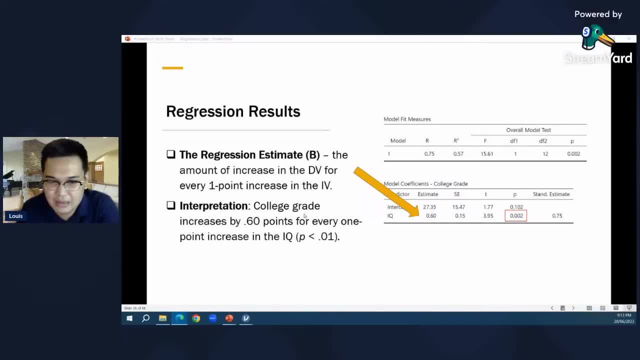 Ibig sabihin, every time tataas yung okay College grade, our outcome variable increases by 0.60 points every time for every one point increase in IQ. So yung 0.60 na yan ang ibig sabihin yan. 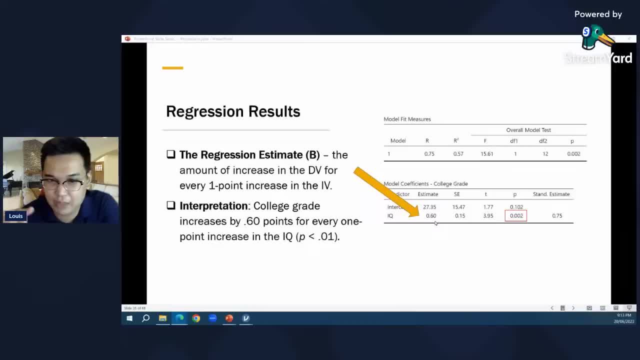 every time yung IQ ng tao tataas by one point, yung college grade niya tataas ng 0.6.. So, going back to correlation, anong klaseng relationship meron sila? Positive or negative? 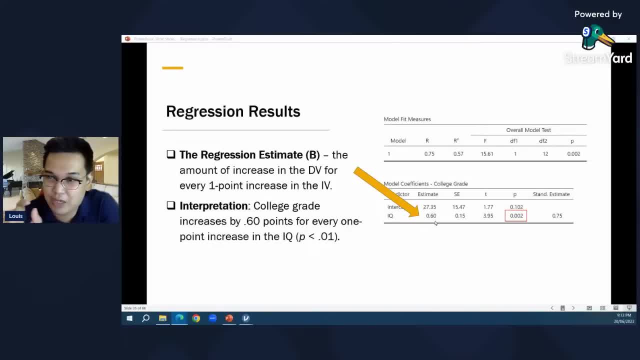 Ulitin ko: ha, every time tataas yung IQ mo ng isang puntos. yung grade mo sa report card tataas by 0.6.. Kunyari IQ 100,, 101,, 102, tumataas siya 1 point, 1 point, 1 point. 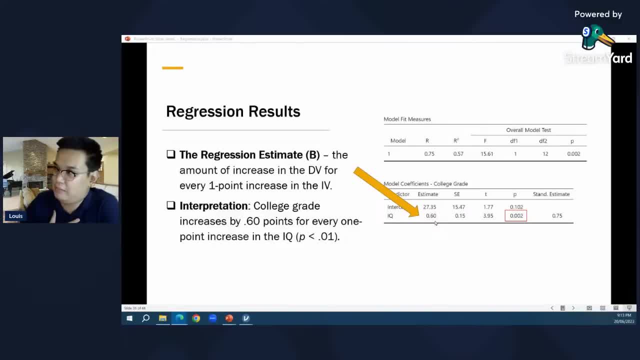 Ako 100 IQ, kunyari, Tapos yung kapatid ko 105, mas mataas siya sakin ng 5 points E di mas matalino siya. Diba Ganun yung meaning, nun, Kung mas matalino siya. 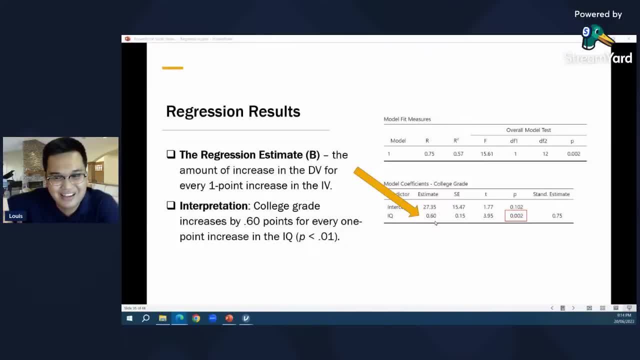 mas mataas yung grades niya Kasi 105, siya ako 100 lang. Very good. There is a positive correlation between the two Significant ba You look at the p-value Diba Lower than 0.05? Yes, 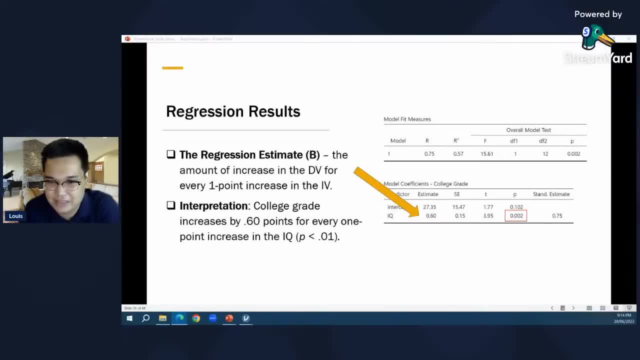 Since napakaliit ng p-value, it is significant Ang interpretation neto, significant yung effect Ni IQ on college grade. Pero, like what I said, aside from this one, aside from the B, mas pagandang tingnan. 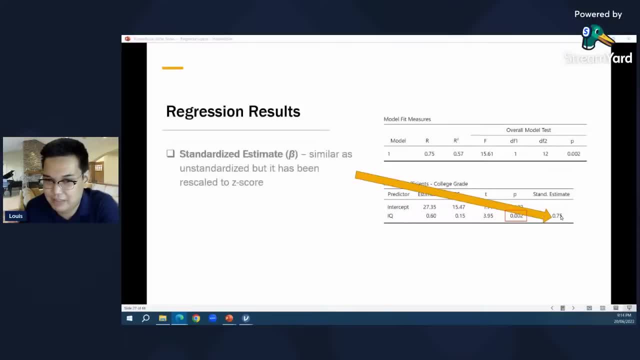 yung standardized, Kasi nga it has been rescaled to z-score, So diba mas accurate siya. Mas gusto natin z-score Sa psychology. Mas bakit, sir, later may example ako mas malilinawan kayo. 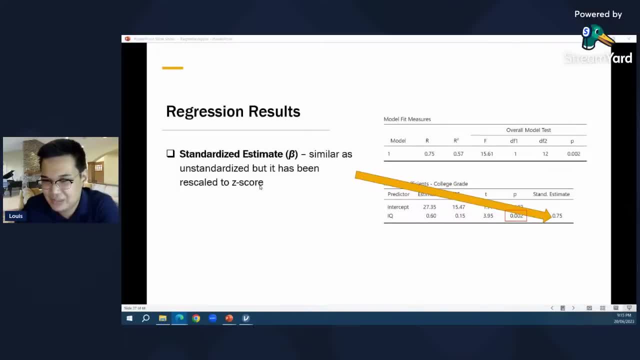 Mas useful siya. kung marami kang variables, Kumbaga mas accurate ito. How do you interpret this As IQ increased by 1 standard deviation unit, college grade increased by 0.75 standard deviation unit? Ano daw. 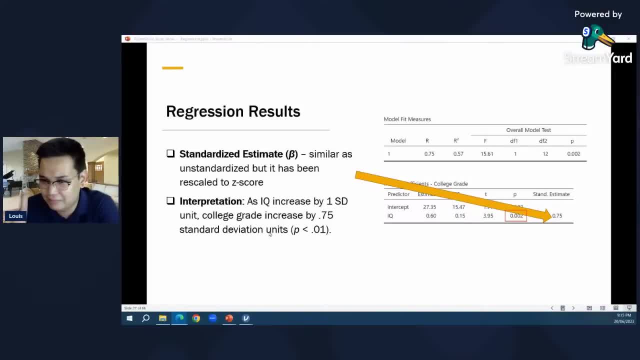 Anong ibig mo sabihin, sir? Hindi namin naiintindihan. E di pasimplihin natin. kung magbabasa ka ng research paper, hindi nila i-interpret yan, katulad nung nasa second bullet. 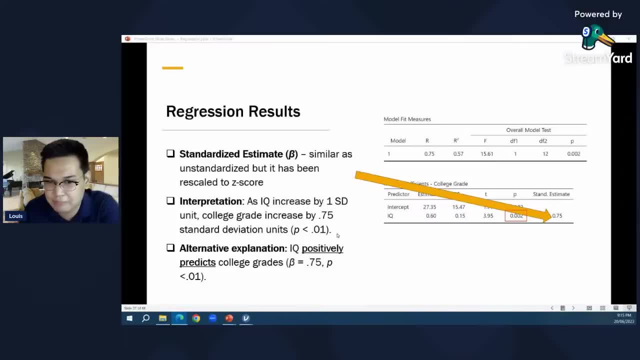 Although alam natin that that is the correct interpretation. Pero kung magbabasa ka ng research paper ganito yan: IQ positively predicts college grades. Anong mas maganda explanation Yung second bullet o yung third bullet? Ano dito. 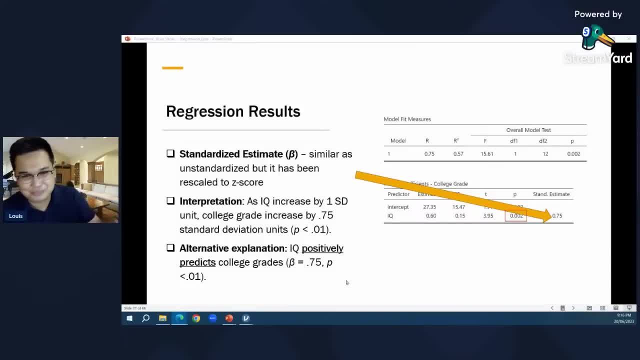 yung mas nagigets ninyo Yung third bullet. Ito yung sinasabi ko sa students ko. Technically tinuro ko yung pangalawa, kasi that's how you interpret it, Pero sa research paper. 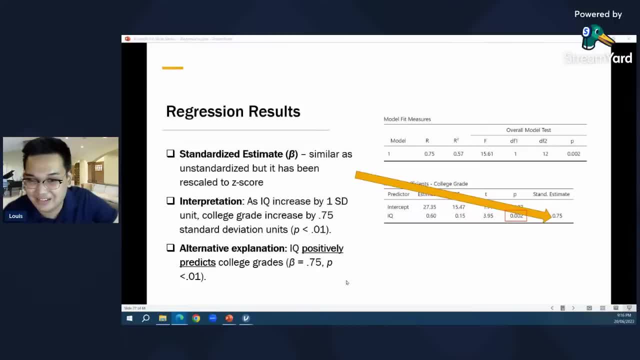 enough na yung third bullet Meaning: the smarter you are, the higher your IQ, the higher your grades. That's the explanation for that Ganyan sa regression. Tapos, by running some analysis, by running some computation, pwede na nating. 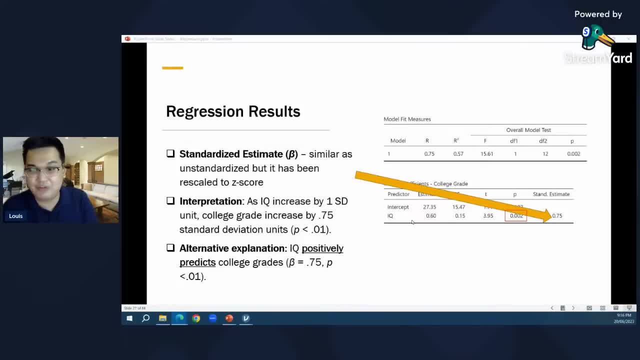 i-predict For some: mas natutuwa sila sa second, Kasi nga sa bell curve. Pero in research usually we report it like yung third. Pero mas tama naman talaga yung second, because it's. 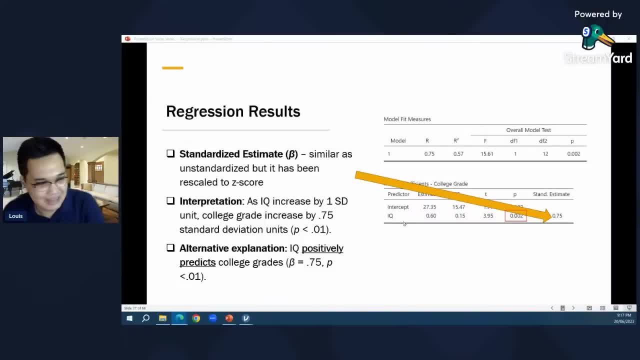 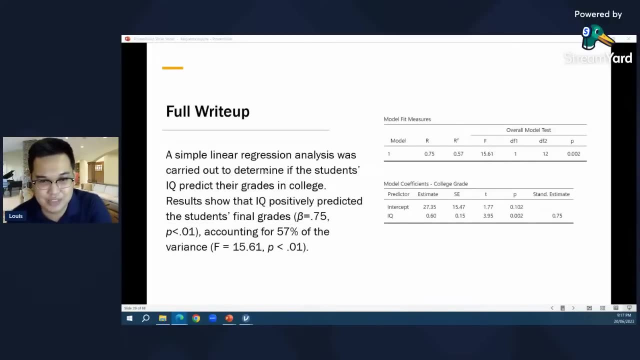 how it's supposed to be interpreted. Okay, Alright, Sige, All in all, this is how you report it. A simple linear regression analysis was carried out to determine if the students' IQ predict their grades in college. Results show that IQ positively. 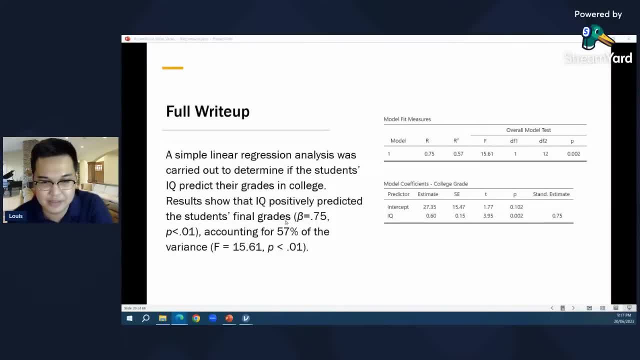 predicted the students' final grades. Nilagay yung beta. nilagay yung p-value. nilagay yung r-squared, Accounting for 57% of the variance. nilagay yung model fit indices. That's how you. 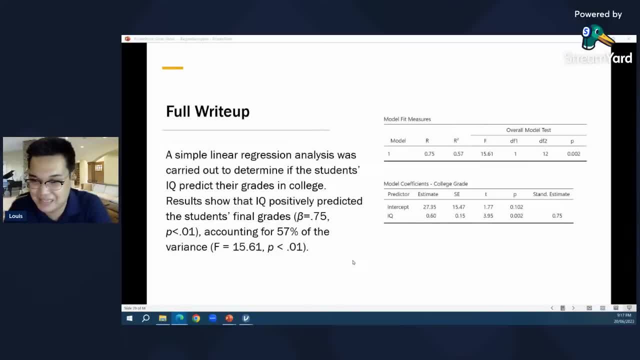 report: regression results. May demo ako after this, But for now meron ba kayong tanong. This is the part na magtatanong ako. kung may questions kayo Before I do my last demo. I think I prepared two. 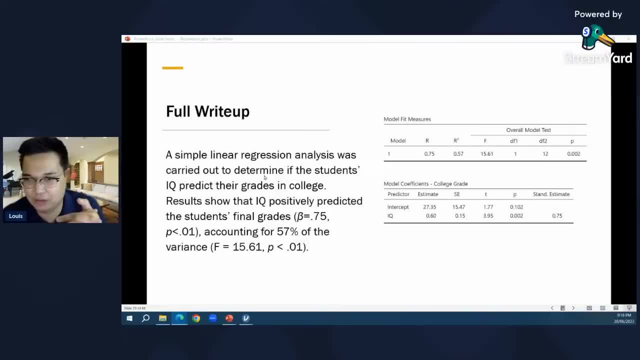 Depende kung makaya, Wala naman tayong limit. kung gusto niyo ito, gawin natin hanggang alas 3 ng madaling araw, Pero dalawa na lang yung demo ko. Pero at this point, 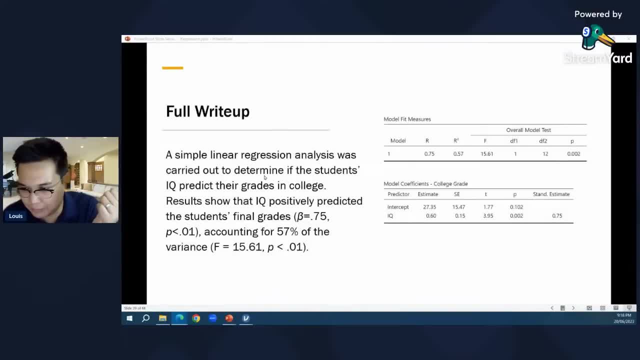 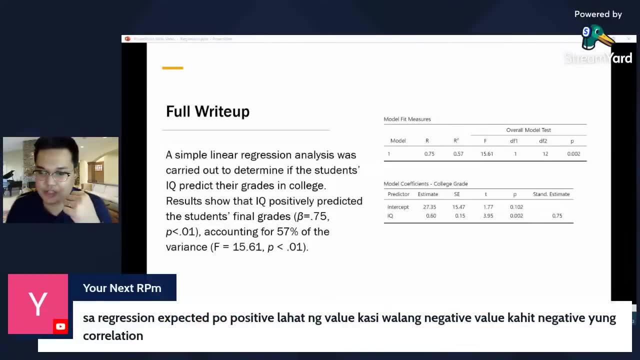 before we go to the demo, do you have? Okay? This is a very good question. Sa regression po ba positive, po ba lahat ng value, Kasi walang negative value, kahit yung negative, mamaya. Tingnan natin, Meron ba. 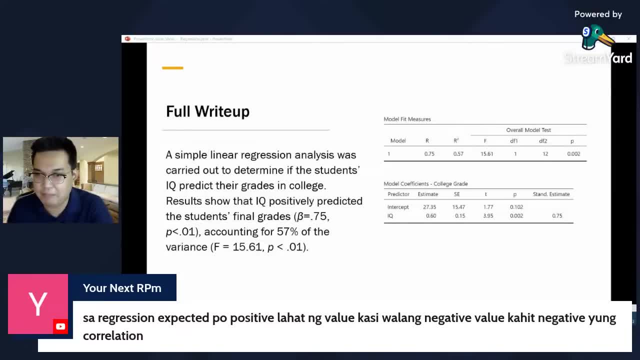 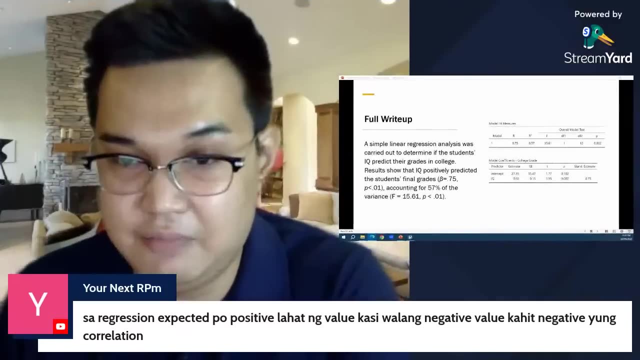 Tingnan natin, ha, Parang may makikita tayong negative mamaya. Pero your next RPM, kapag yung estimate o yung standardized estimate negative, siya dun, siya magiging negatively predicts. Okay, Dun siya magiging negatively predicts. 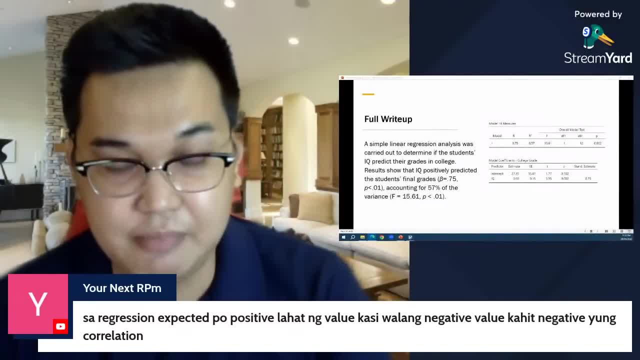 Kapag yung estimate value or yung standardized estimate has a negative symbol. Kailan lang nangyayari, sir, yung negative symbol Kapag negatively correlated, sila Kunyari kapag mas mataas ang presyo ng gasolina. 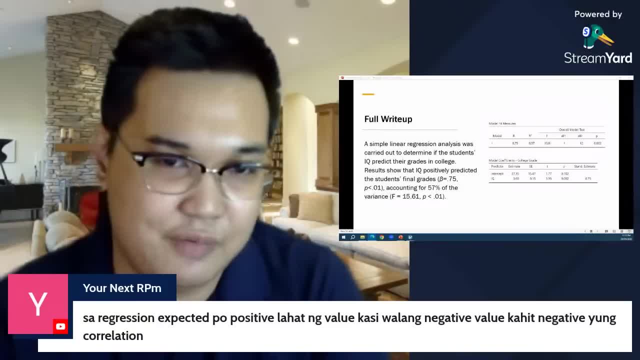 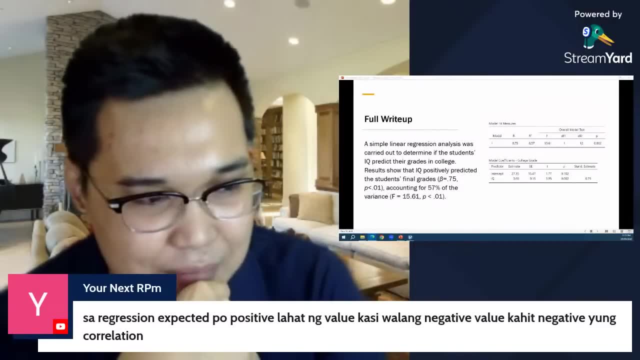 ano kayang apektado dyan. Think of a run Okay, Or what else. Kunyari, kapag mas mataas yung ano ba maganda example for negative: Okay, Titingnan ko ha, Parang mamaya. meron akong example dito na. 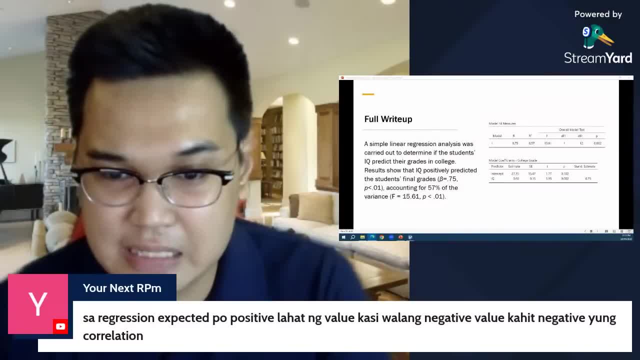 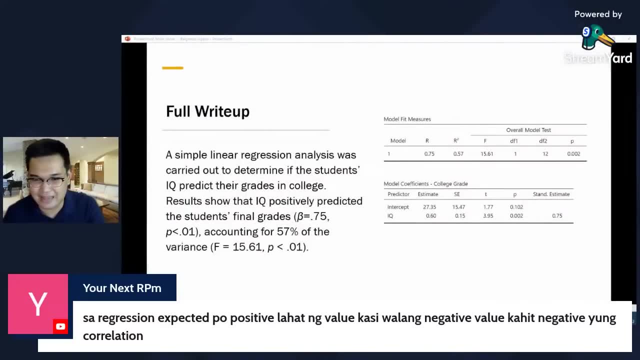 posibleng may negative, Pero so far kasi example ko puro positive. Ayan Sige, Ayun Ayun Ayusip ko na Kapag mas mataas yung presyo ng gasolina, mas konti ang gusto mong. 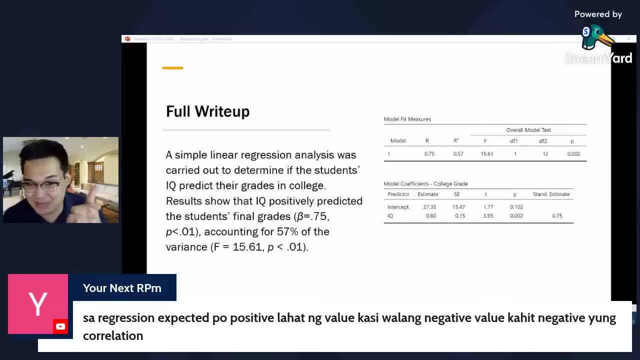 pag-gasolina, Parang ganun, Parang ganun siya, kapag negatively predicts. Okay, Ayan To end the lecture part kasi magdedemo na. Ay hindi, I will cover multiple regression, then last demo na Okay. 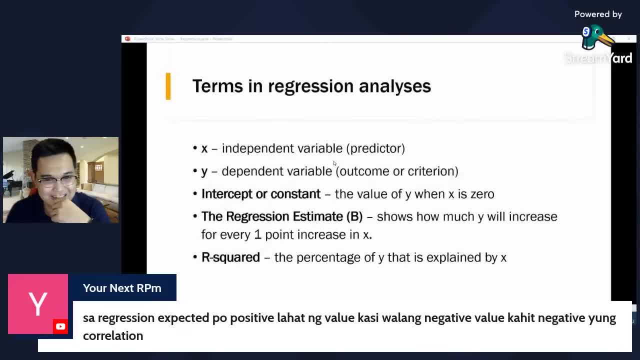 Other questions Na Ayan, Pinapakita ko lang ulit yung terms Na-discuss na siya kanina. Maybe you're wondering, Sir, paano ko- Diba sabi mo originally yung regression- ginagamit siya to predict. 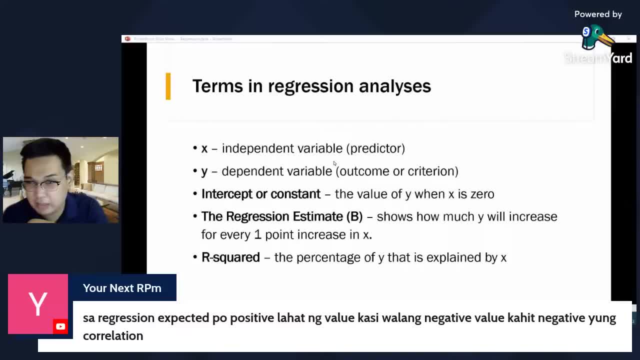 Eh, Sir, paano kami magpe-predict using that- Although I rarely discuss this in psychology, kasi nga we rarely use regression to predict Sa business, talaga ginagamit siya. Yung econ teacher ko pinagpe-predict. 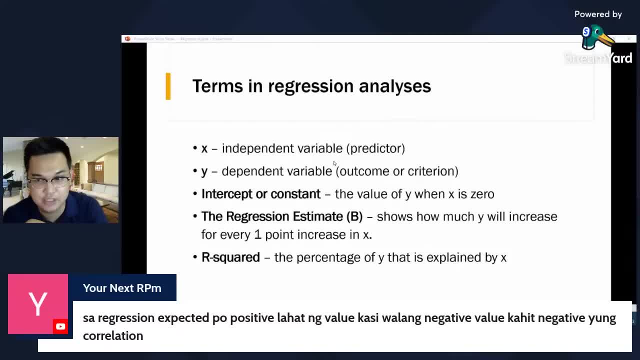 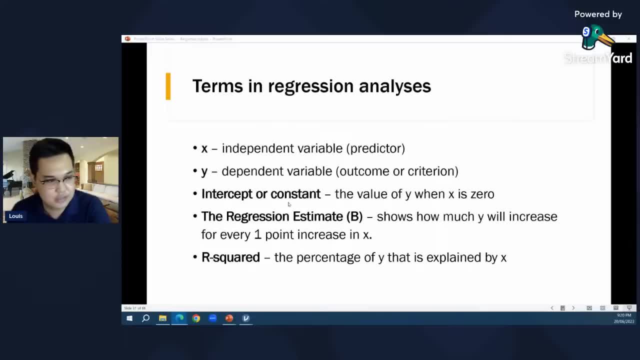 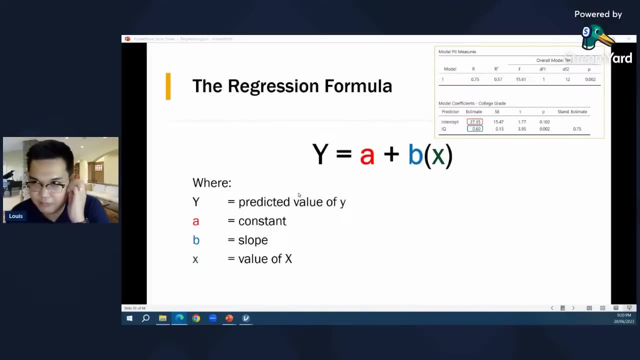 kami using regression Nung college. ako may econ subject kasi kami. Pero just in case you're curious, Just in case you're curious, Okay, This is the regression formula. Feel ko curious, kayo dito kasi nakikita nyo to sa textbook. 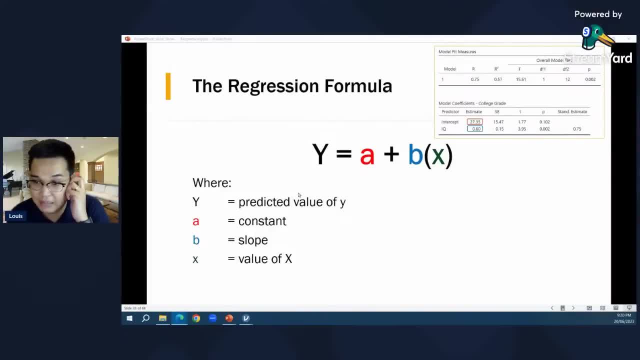 Kunyari, ni Cohen tsaka ni Kaplan Diba. The regression formula is: y equals a plus b times x, where y is the predicted value of y, the a is the constant. and tama ka sa tanong mo kanina, The b is the slope. 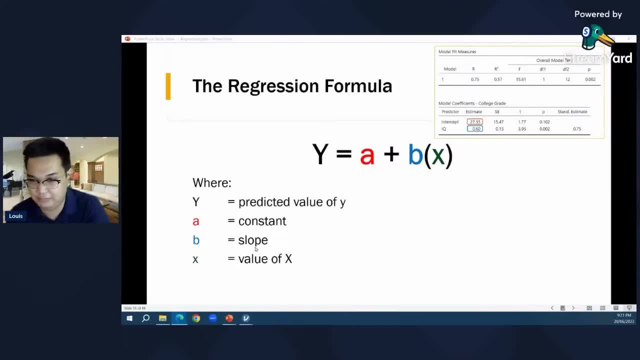 or the regression coefficient, and the x is the value of x. In other words, kung magpe-predict tayo, eto yung formula na gagamitin natin. Ginawa kong makulay para mas madali ninyong. 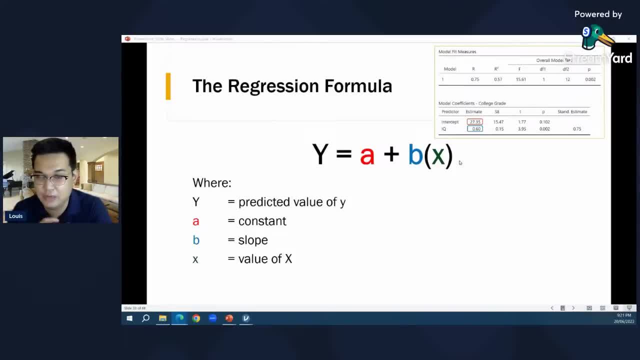 mahanap dun sa table sa upper right kung anong values yung gagamitin Ngayon mag-predict tayo Kunyari. this is my example. What would be the predicted grade of the student kung yung IQ? 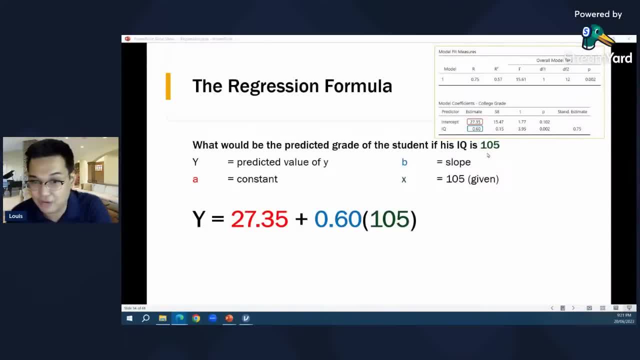 nya is 105?? Ano yung magiging grade nya? Eto prediction na tayo. So kapag nag-run ka ng regression analysis sa SPSS or whatever, tapos nakuha mo yung mga values na to dun ka na pwedeng mag-predict. 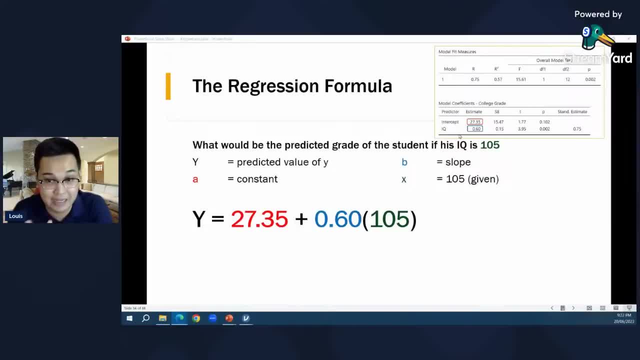 Kaya bumabalik tayo sa purpose ng regression, which is prediction. What would be the grade of the student if his IQ is 105? Definitely mataas, yan kasi matalino. Hindi naman matalino, pero 105 above average. 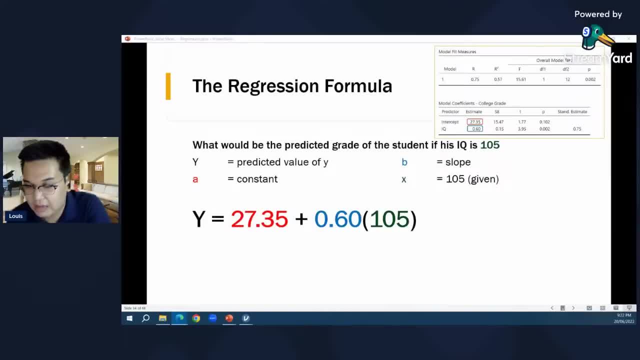 Bakit mas maganda gamitin si Beta- Una standardized score siya- rather than raw score? Pangalawa mamaya, ipapakita ko kung bakit May sagot na si Grecia. Grecia was my student. 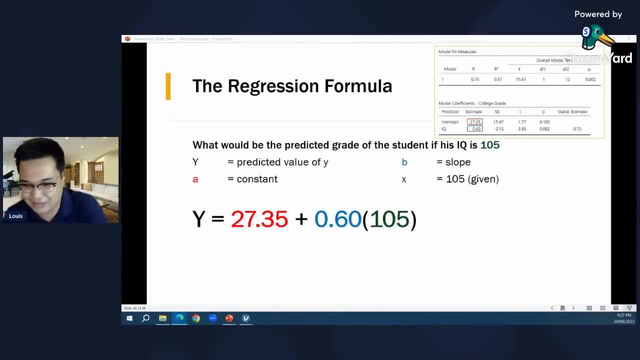 before: Hello, 90. Tingnan natin, Pareho ba tayo ng computation, Kinumpit ko siya. So this is how you will do it. sa formula A plus B times X, The A is the constant. So this is it. 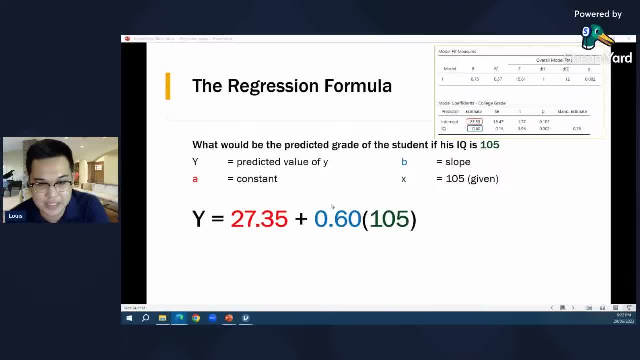 27.35.. The constant or the intercept, The B, is 0.6.. While the X is koning, given 100, 110 or whatever, After doing some computation, 90 or 90.35.. Meaning kapag yung IQ mo. 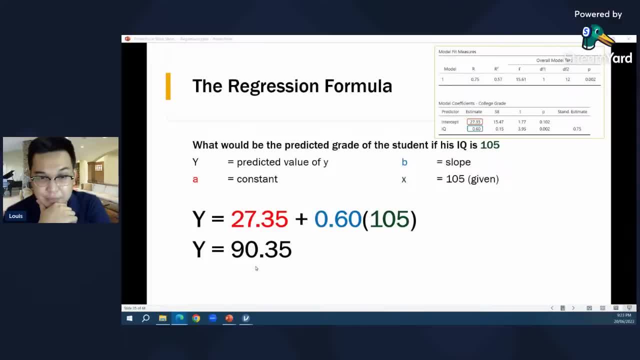 105, yung predicted grade mo magiging 90.35.. And that, my dear students, is how you use regression to make predictions. Ngayon gets yun na Nag-make sense na ba sa inyo. Ngayon gets yun na kung bakit, kapag 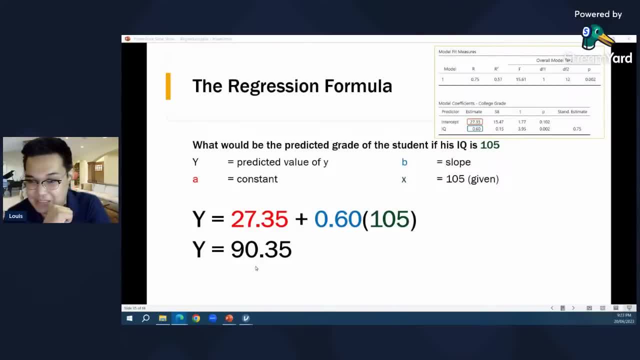 regression. it's the word that comes into mind is prediction, Kasi gumagami tayo ng formula to make predictions. Pero in psychology we rarely use this formula. Depende sa feature niyo. Pero ako we're not interested with this, We're interested with. 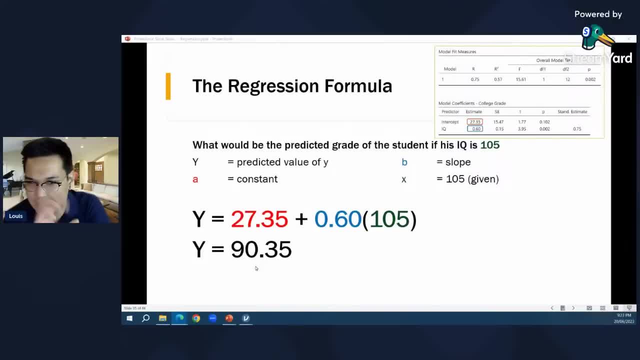 gaano kalaki or kaliit yung effect? Gaano kalaki or kaliit yung standardized estimate. That's what we care about. Okay Yan, Pero kung magbabasa kayo ng research from ABM Accountancy Business Management, 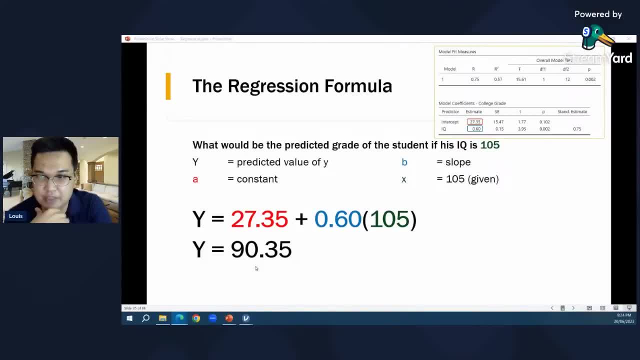 ECON Dati nagbabasa ako ng mga research from other fields, Talagang very specific, Dati may client ako Nagpagawa siya sa akin ng regression equation. What will be the GDP of the Philippines if this is the amount of money? the 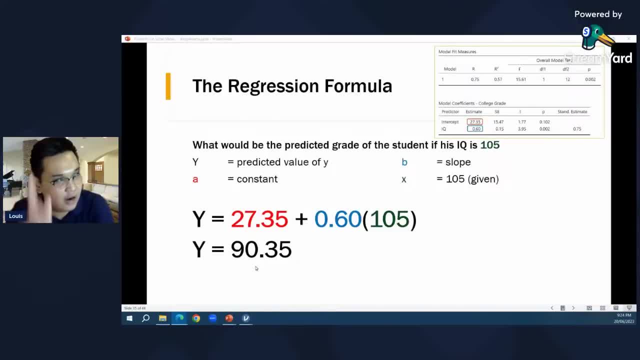 government will spend on the Navy, on the Army, on the Air Force. Yun, yung pinagawa niya sa akin? Okay, I don't think so. Kaya nga sabi ko hindi, Diniscuss ko lang siya para. 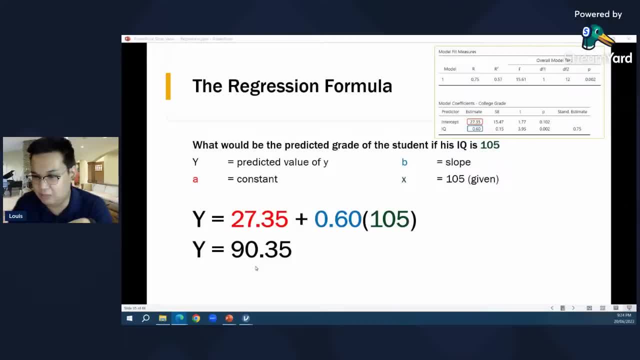 mag-gets ninyo Mali. ninyo meron, pero nung time ko wala naman, I don't think so. Yun yung sagot ko, dyan. Okay, The reason why I discuss it: maganda na gets niyo siya in terms of concept. 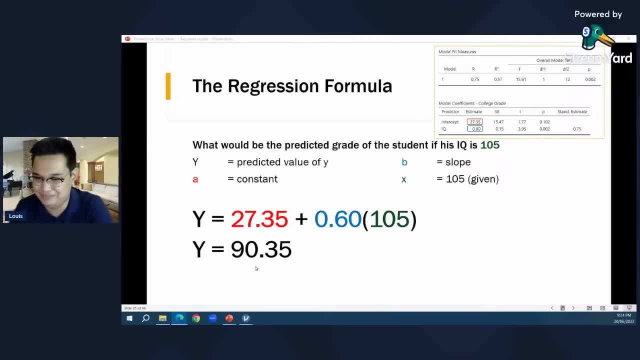 Kesa, yung mathematical side Yun. Okay, I think ang kutob ko dyan it's more of the concept of regression rather than the technical side of it. Hindi ko na siya malakihan. Sorry, kasi naka PowerPoint na siya. 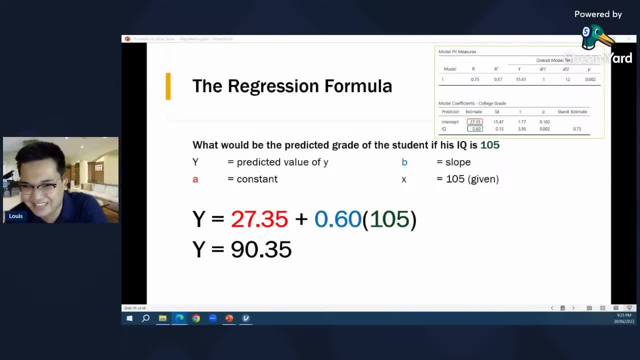 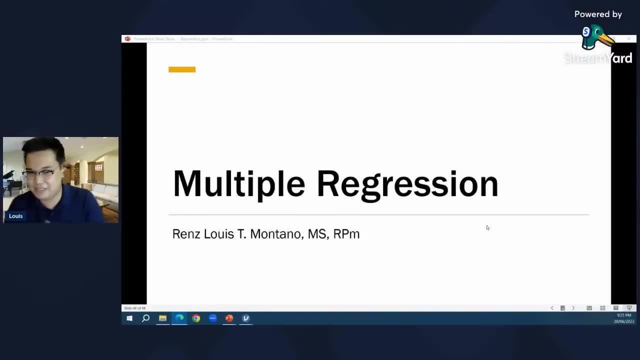 Yun lang. Sorry, Pero yung next commit yun yung malaki-laki Ayan Last part Sige Tapos dalawang demo. Okay, Ang kaibahan lang ng simple tsaka multiple sa simple. 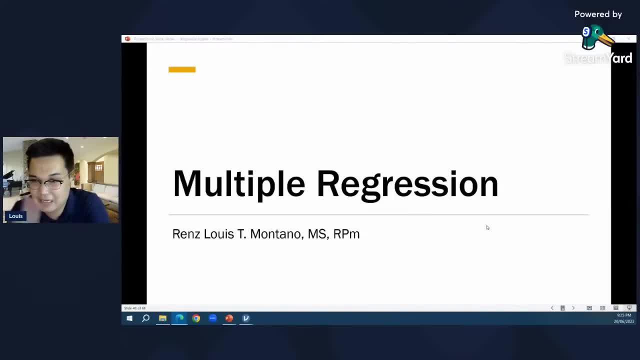 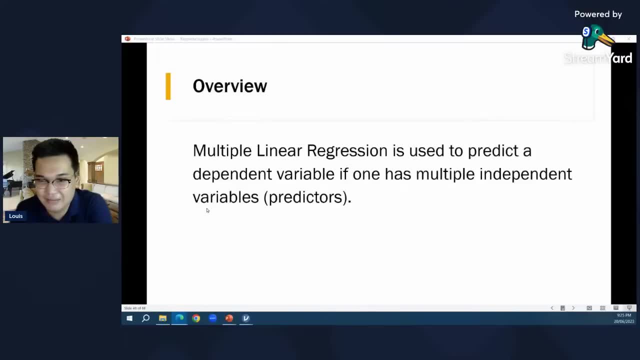 isa lang yung variable na predictor mo, Isa lang yung outcome mo, Pero sa multiple- kaya siya tinawag na multiple- marami ng variables yung tinitingnan mo. Multiple linear regression is used to predict a dependent. 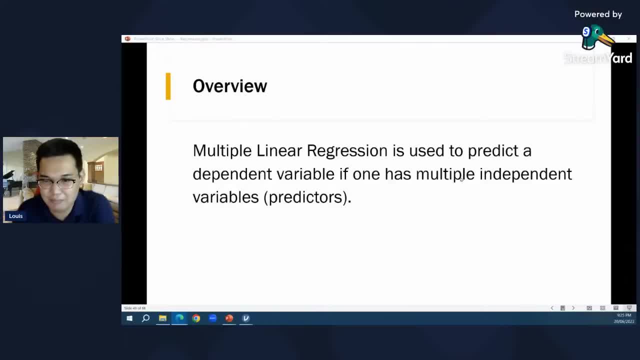 variable if one has multiple, marami, maraming independent variables or predictors. Tinitingnan mo ano yung effect ng dalawang variable na to sa isang outcome variable? Hindi na isa Kapag dalawa na siya. 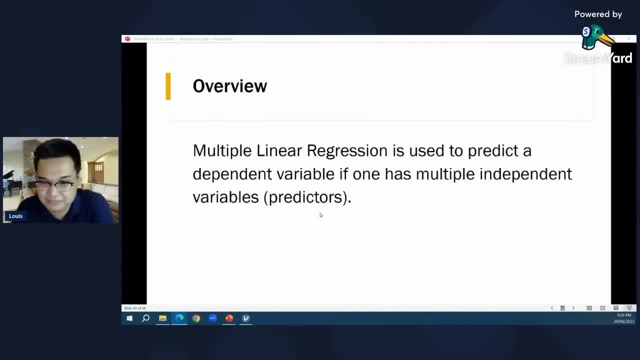 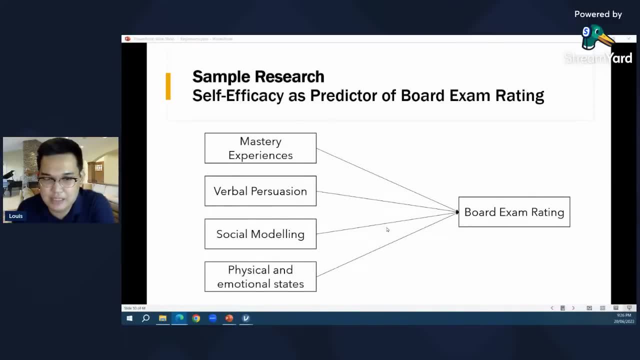 or more it becomes multiple. Okay, Sige, Here are some examples: Kunyari Ayan Usapang board exam: Self-efficacy as predictor of board exam Kung self-efficacy lang mismo in board exam. 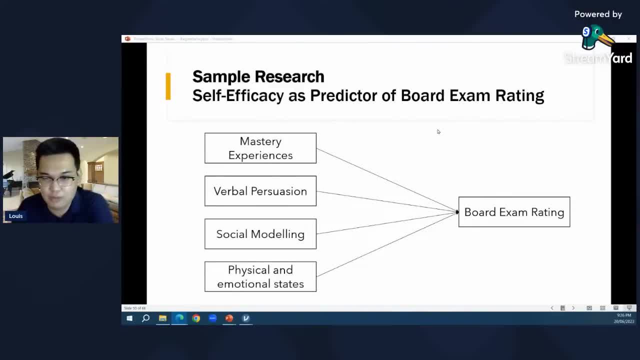 simple lang yun, Pero kung i-de-divide natin siya onto components. according to Bandura, may apat na component yan Mastery, verbal persuasion, social modeling, physical-emotional states. Makikita natin kung gaano. 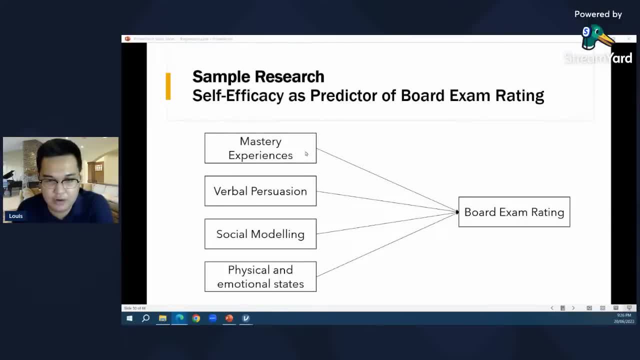 or among these four- sino sa kanila or ano sa kanila- yung may pinakamalaking efekto sa board exam? Sige Kunyari, Sa tingin nyo? I would like to ask you: ano sa apat na to, sa tingin nyo yung? 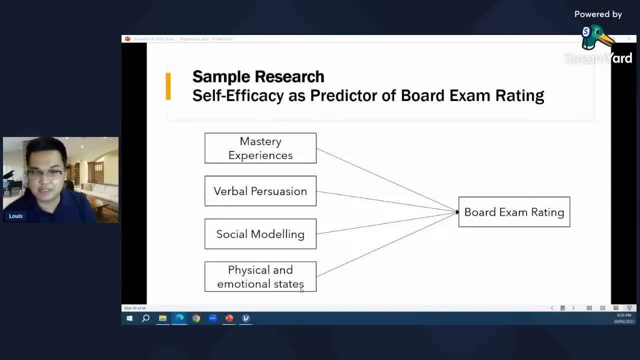 most likely will predict board exam success. Usapang Bandura tayo ngayon Si mastery ba Si verbal, Si social modeling Or si physical-emotional states. What do you think among these four predicts board exam success? Very good See. 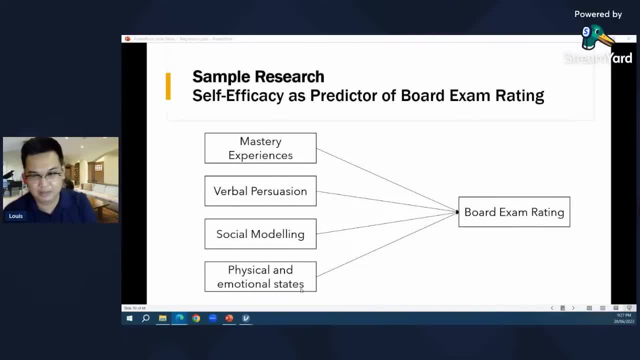 Sabi nga ni Bandura mastery, The more that you know the topic, the more na confident ka about sa inaaran mo. the more na alam mo yung inaaran mo, the more that you succeed. Ayan Ang medyo mahina. 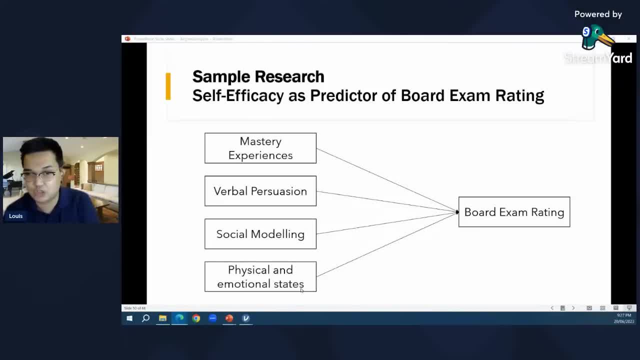 si si verbal persuasion. eh Kasi, what if sinasabi: oh, kaya mo yan. Tapos what if hindi? ka naman nag-aaral Diba Ayan, Okay Si physical-emotional yung efekt niya negative, So may. 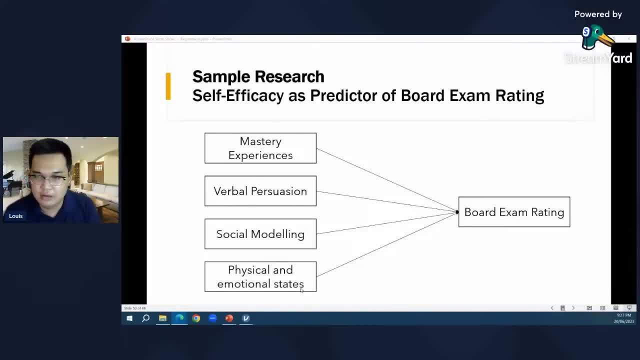 nagtanong nung kanina diba Si ikaw ba yun your next RPM. No, Eto negative to Kunyari nilalagnat ka Physical state yun Malamang bababa board exam rating mo yan kasi. 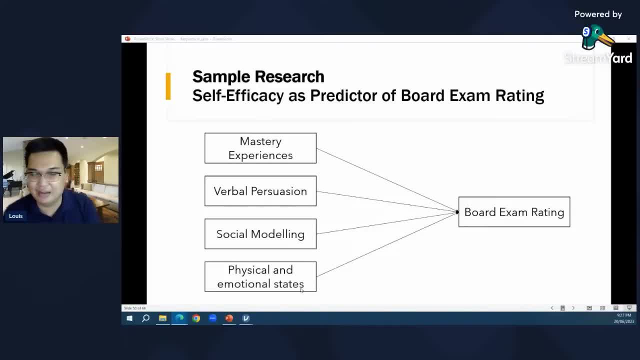 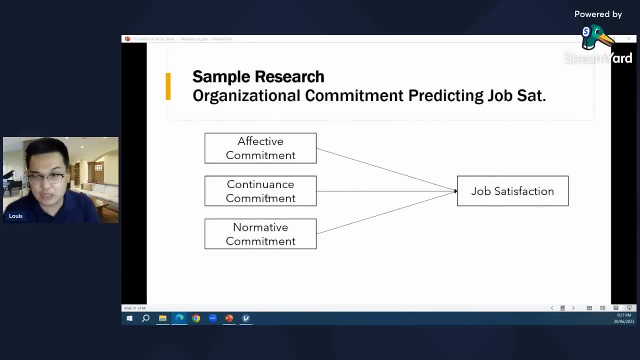 nilalagnat ka. So ganito, ang ganito ang ano, no multiple regression. Another example ako, kahit hindi ako IO major, natutuwa ako sa mga topic sa IO: The effect of the three types of commitment on. 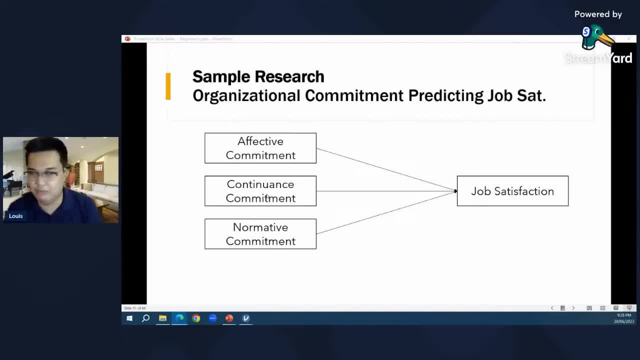 job satisfaction. Diba tatlo yan Affective continuance normative. Ano dyan sa tatlo yung pe-predict ng job satisfaction. Ako sa tingin ko effective, Mas masaya ka sa trabaho mo. 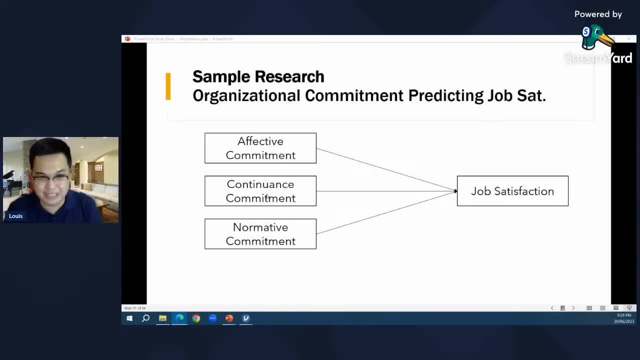 Ay sorry, Mas mas masaya ka sa company, Mas mahal mo yung company, Mas masaya ka sa trabaho mo, Ganun siya, While the other two I think yung continuance negative yung effect niya. I think lang nga, I think lang. 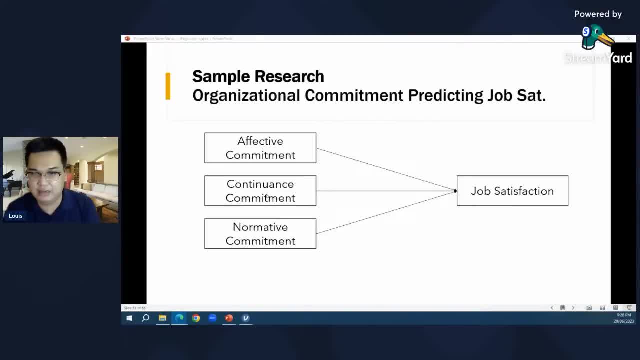 Tapos I think yung normative medyo mahina yung effect niya. Okay, Eto, binibase ko ito sa real research. Maraming nag-i-study na ito ng commitment na ginagamitan ng regression. 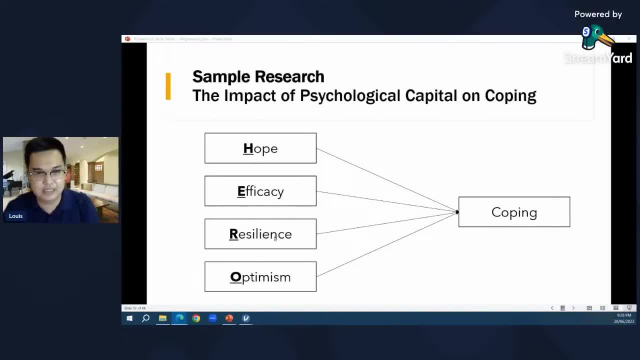 What else The effect of hope, self-efficacy, resilience and optimism, or what we call heroes Baka itanong ito sa IO. I don't know When we say psychological capital sa IO, hero yan Hope, efficacy. 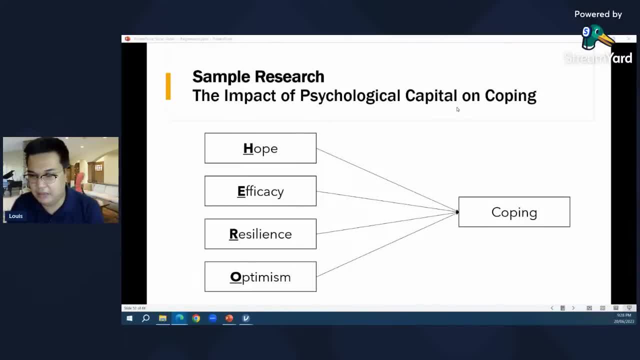 and resilience optimism. Okay, I have a colleague right now sa university: IO, No, IO, Nag-conduct sila ng intervention sa isang company. Ewan ko kung tapos na or magkakandak pa lang. 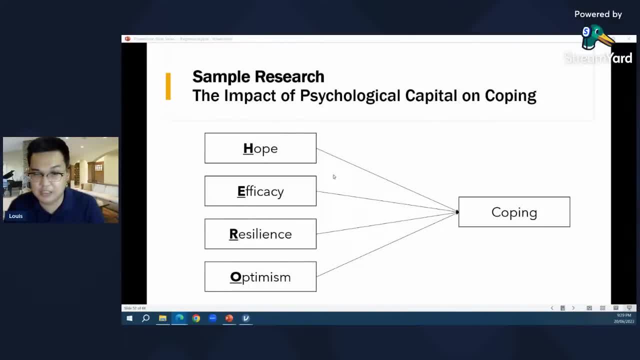 In-increase nila yung hope, efficacy, resilience, optimism, Tapos nanitingnan nila anong effect. nun, Okay, Ang tawag dyan, just in case lumabas siya. we call that psychological capital. 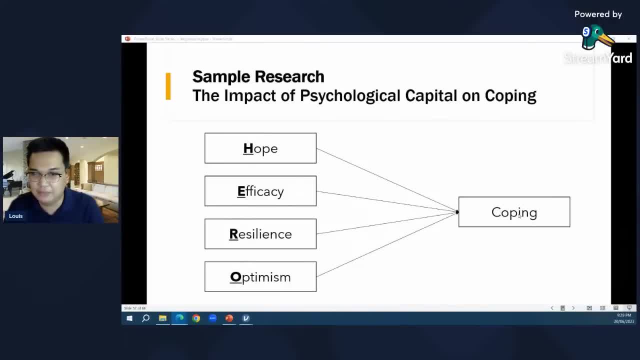 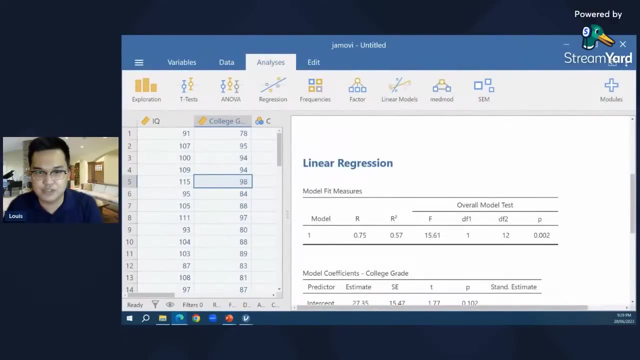 In short, that's the hero ng isang empleyado. Does it affect coping Yan Sige? Okay, I think that's the last part sa PowerPoint ko, And now we do some demonstration. Okay, Sa demo natin. 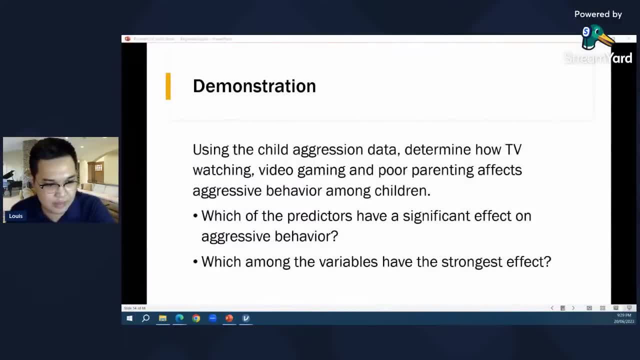 eto yung gagawin natin. I'll prepare the data, Basahin niyo yung instructions. Tingnan natin no, yung child aggression: Using the child aggression data, determine how TV watching, video gaming and poor parenting. 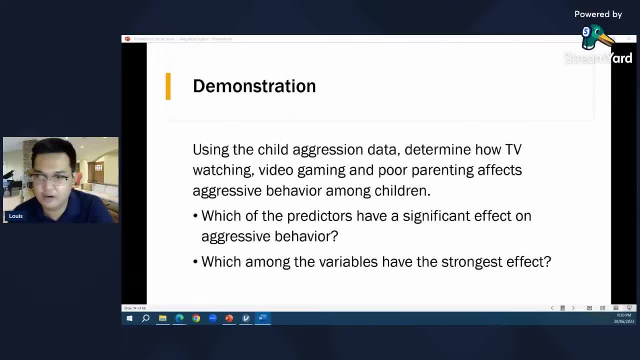 affects aggressive behavior among children. Particularly, which of the predictors have a significant effect on aggressive behavior? Pangalawa, which among the variables have the strongest effect? Ano sa tingin niyo, Hulaan lang natin Ba't ba nagiging masama? 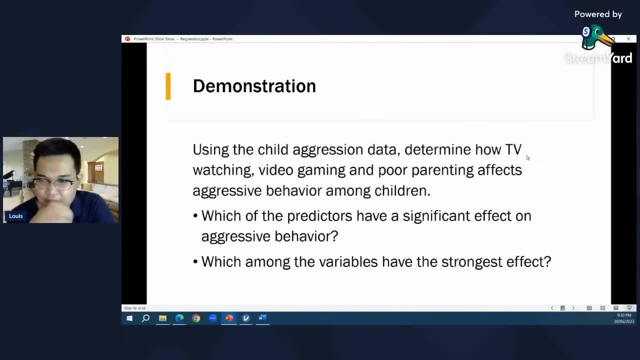 yung mga bata, Ba't sila nanununtok, nangangagat, nananabunot, Kakanood ba ng TV, Kaka-computer, Kaka-cellphone, Video gaming? Or do you think it's parenting? 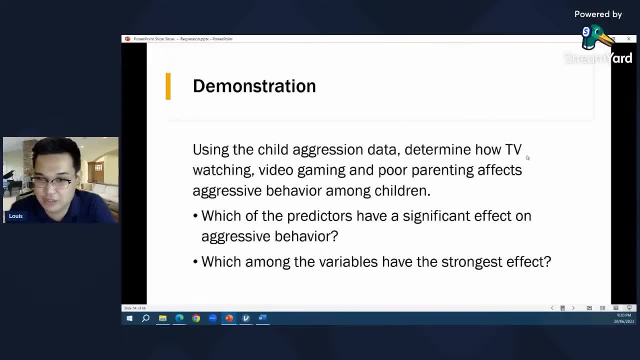 Eto, pwede itong dev psych. Kung dev psych major ka, pwede ito yung study mo Dev psych? o yan sabi ni ano. sabi nila poor parenting daw. Yan yung tingin nila. 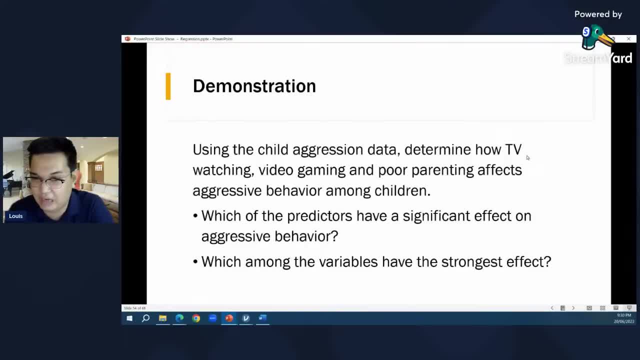 Or pwede naman kasi hindi lang isa, Pwedeng silang lahat, Pwedeng dalawa. Okay, So ano yung effect nila? Yun yung titignan natin. I prepared the data set ahead of time. 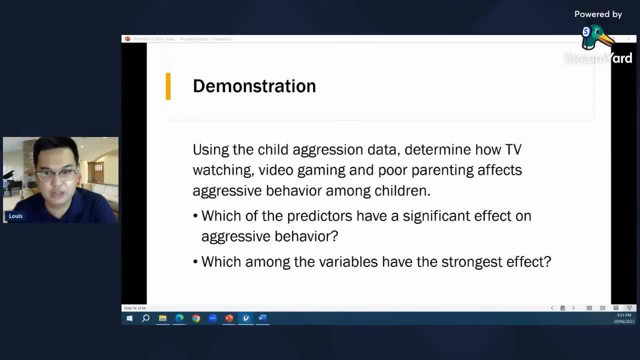 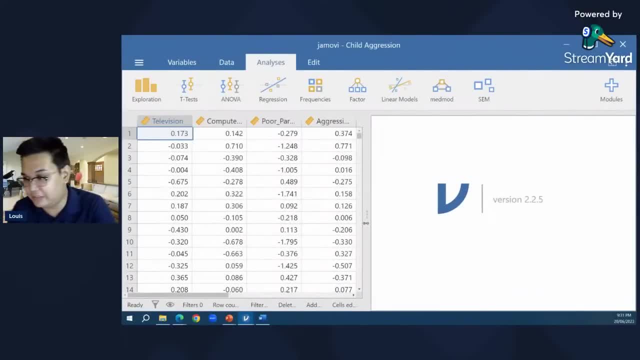 This is based on a real study. I forgot who the real authors were. Credits to the real authors. I got the data from the textbook of Andy Field. Okay, So here's the data set. So, basically, I don't know how they did this pero. 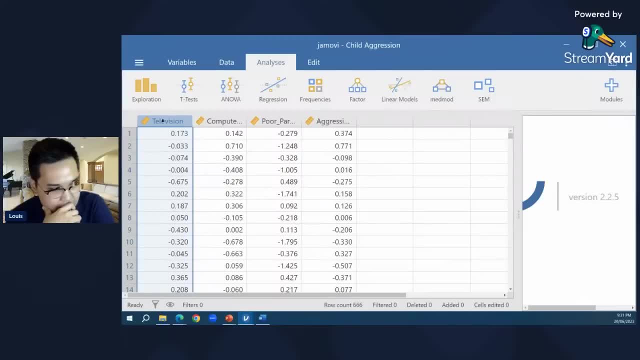 I think nag-survey sila sa mga bata. Medyo malabo na nag-survey sila sa mga bata. I think this is observation. I think instead na yung bata yung nagsagot, baka yung nanay. 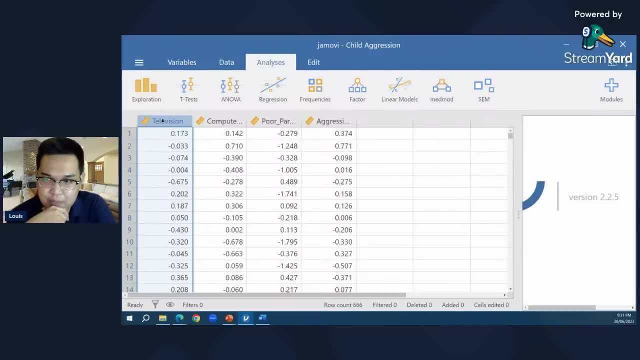 yung pinagsagot neto. Hindi ko lang alam paano may nesure yung poor parenting. Kasi kunyari, kung nanay yung nagsagot, magiging honest ba siya doon. 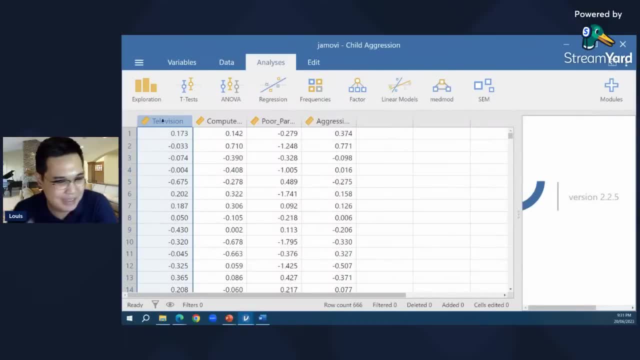 Anyway, hindi yun yung problema natin, Huwag na natin problemahin yun. Basta nagawa nalang yung study. yun yung mahalaga, Tapos ito yung mga variables natin. 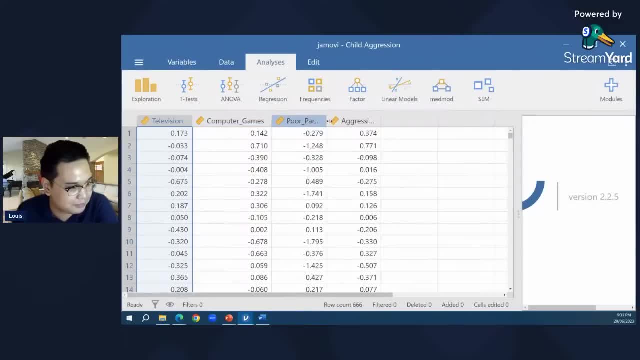 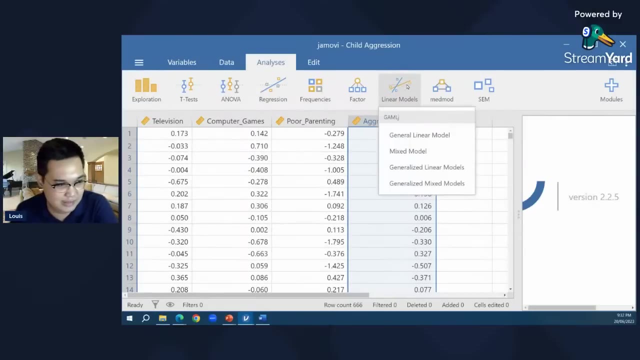 Television watching, computer gaming, poor parenting. Our outcome is aggression. Bakit nagiging agresibo ang mga bata? Okay, Let's run the analysis Review. i-correlate muna natin, Correlation muna, Regression. 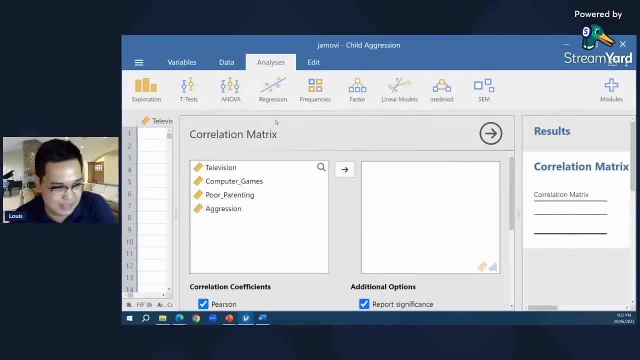 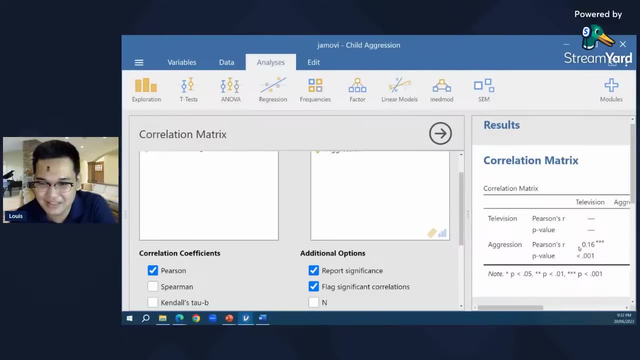 correlation. Isa-isahin natin Television and aggression Significant. The more na nanonood ka ng TV with tatlong asterisk pa yan, the more na nagiging aggressive ka. Pero yung relationship is weak, Mahina 0.16.. 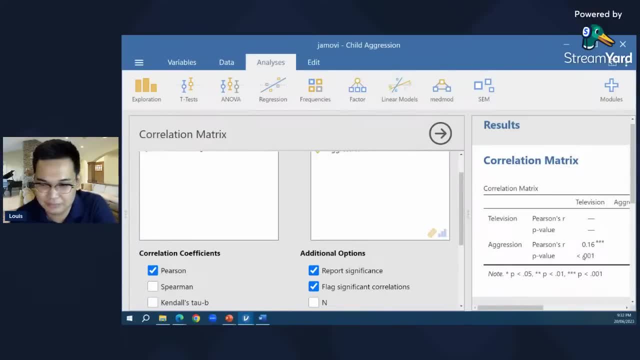 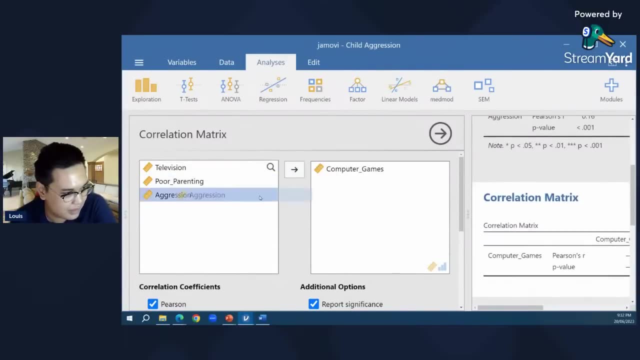 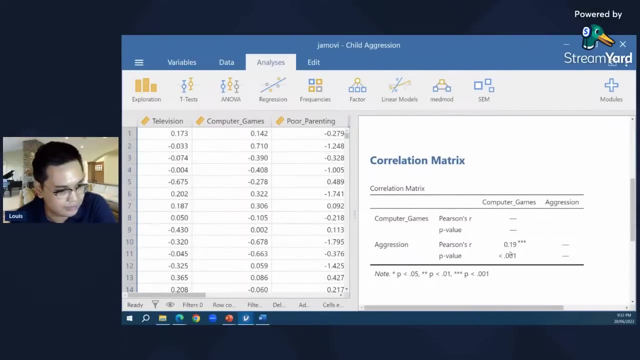 Compared kanina: 0.75.. Yung una, tingnan natin yung iba. Next, Computer games: aggression: Mas matinti to 0.19.. Significant ba? Yes, it is Last one. 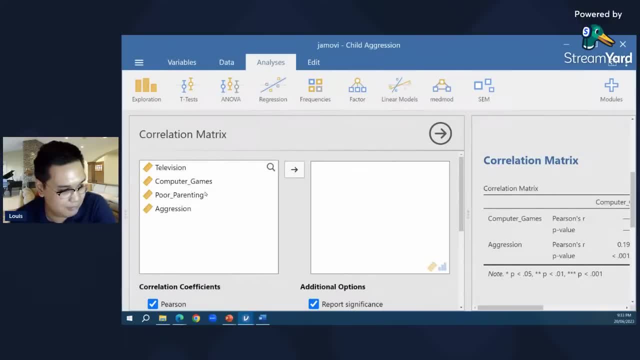 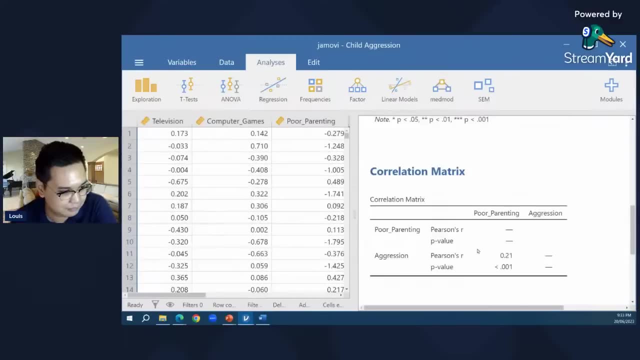 Tapos mag-regression na tayo after Poor parenting aggression. Maniara hindi marunong yung nanay magpalaki ng bata. Hindi ko na checkan yung star Mas matindi Effect 0.21.. 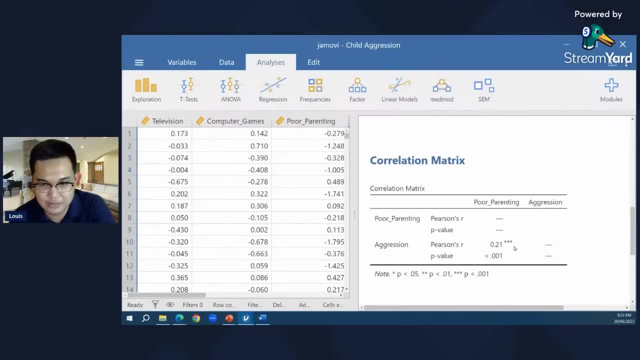 Dito palang may clues na tayo, Pero kasi hindi ito accurate, dahil when you do correlation you ignore the other variables Sa regression, kasi you take into account yung mga variables para malaman mo sa tatlong yan. 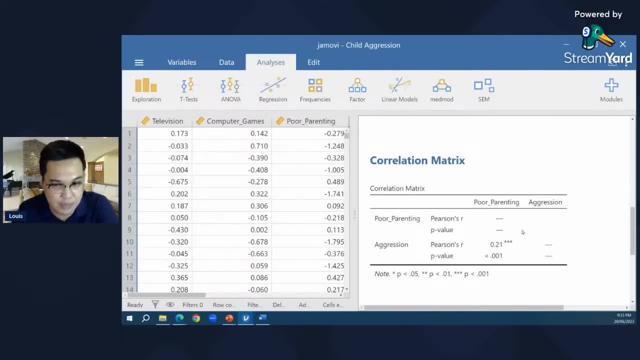 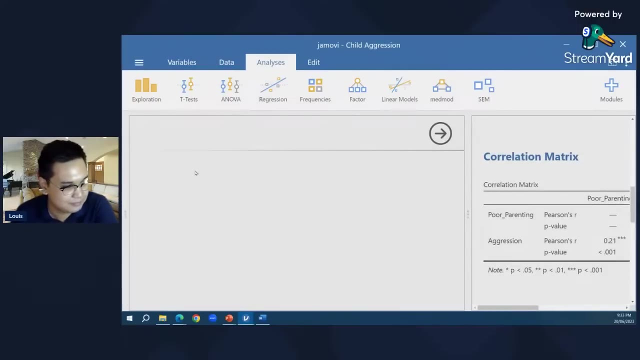 ano talaga yung may effect, ano yung wala. Okay Kaya mas accurate yung regression Because in regression you do not ignore the other variables, You consider their effect. So let's run a regression: Our outcome variable. 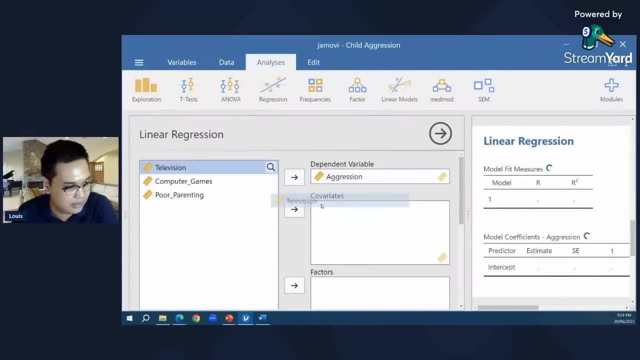 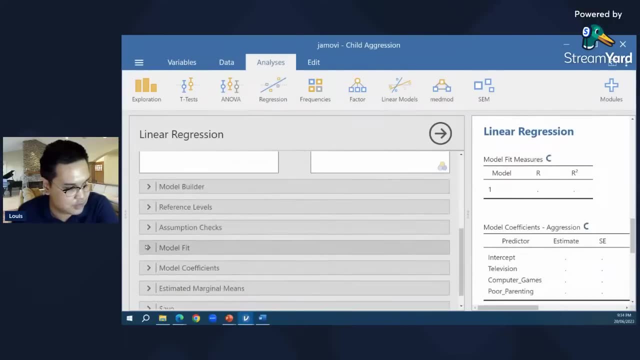 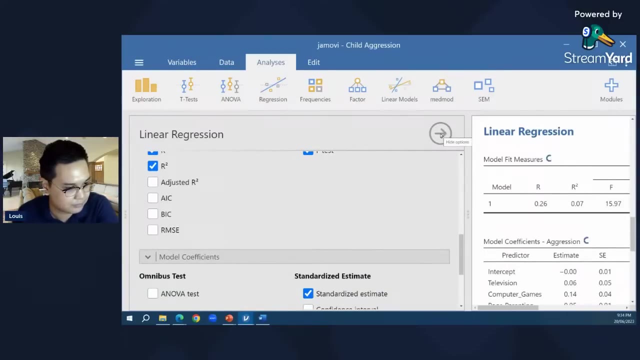 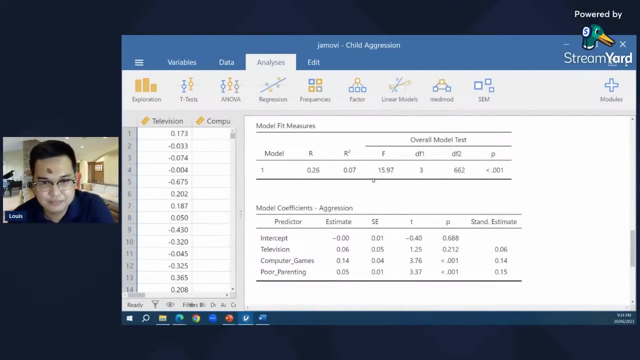 is aggression. Our predictors are television, computer gaming. scroll down sa left. Gusto kong makita yung model fit At. gusto kong makita yung standardized coefficients. And here are the results: R squared medyo mababa. 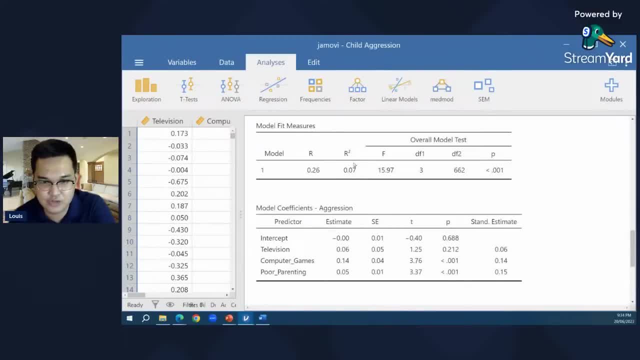 0.07.. 7% lang ng aggression yung iniexplain yung tatlong variables na to Meaning. may iba pang variables that can explain aggression aside from these three. Ano kaya yun Tulungan niya ako mag-isip. 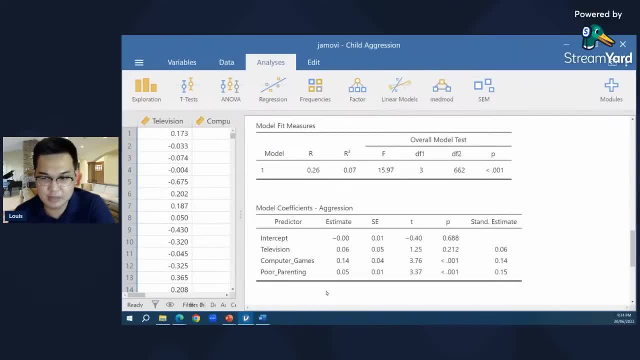 Maybe temperament, What else? Ano pa sa tingin niyo, Maybe modeling Kunyari, kung may kuya sila na aggressive Medyo mababa, no 7% lang, Times 100, kasi yan eh. 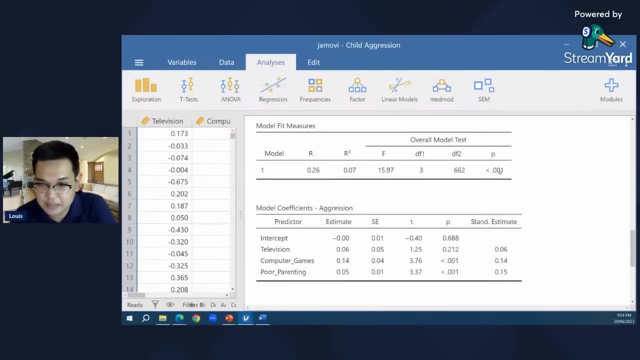 0.07.. 7%, Pero still significant. Kapag nag-significant yan at tumingin ka sa baba dyan mo makikita kung ano sa mga variables mo yung significant or not. Kapag dito pa lang sa taas. 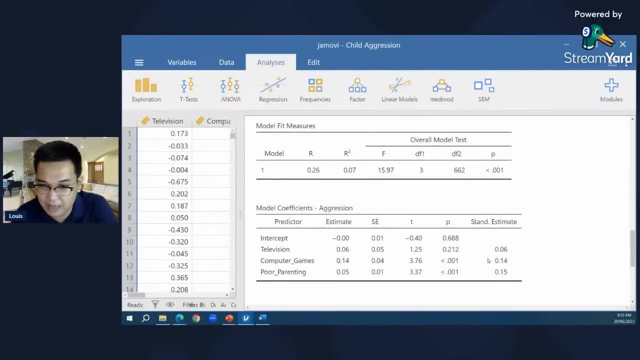 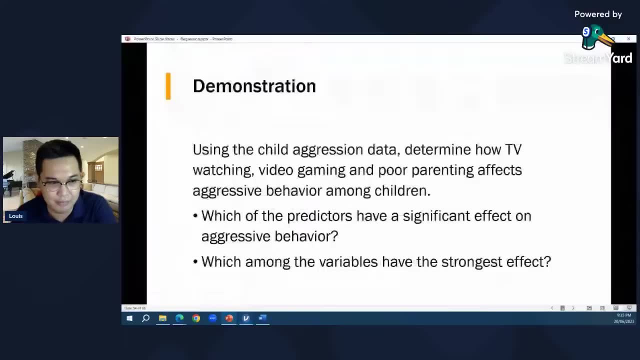 hindi na significant. huwag ka na mag-expect na significant sa baba Ganun siya Kaya mahalagang tinitingnan yung model fit, Pero meron ako mas malaking version yan sa PowerPoint. Same lang pala. 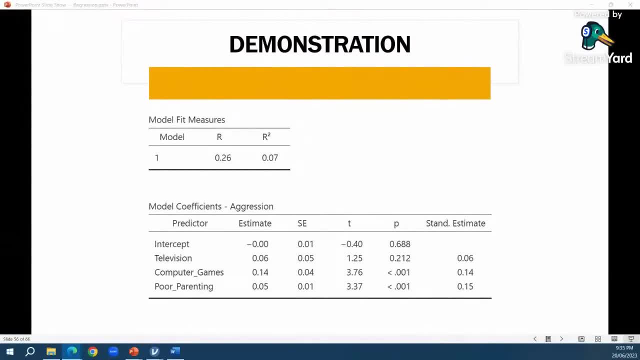 But anyways, Isa-isa yun Himay-himayin natin Television, Significant or not? What do you think? Significant type SIG or not? significant type NS? How do you understand the results based on our discussion? Ang panonood ba ng TV. 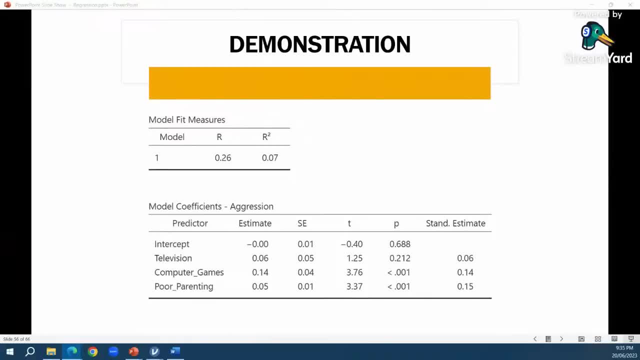 ay may efekto sa pagiging agresibo. Look at the p-value. What do you think? Significant or NS? Okay, May mga nagsasabing significant, May mga NS Okay, But the correct answer is NS, Kasi yung. 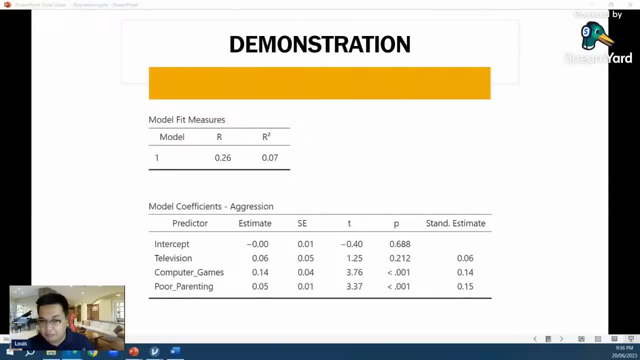 p-value mo higher than .05.. Meaning, walang kinalaman ang panonood ng TV sa aggression. E di ano yung may kinalaman, sir? Next, computer gaming: Significant or NS. Significant or NS Computer gaming. 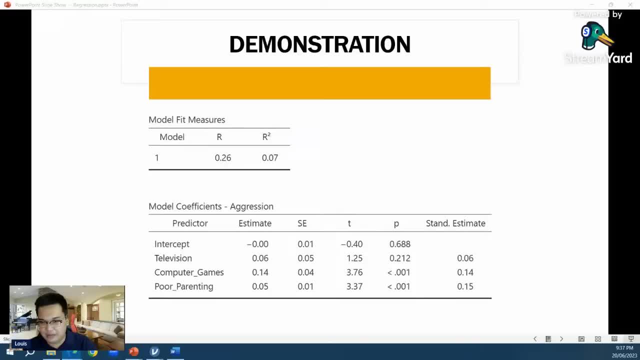 Ito si computer games. Isa to yung p-value niya. Ayan tama Significant, Kasi sobrang liit ng p-value Meaning may efekt talaga siya. Aning efekt niya. You look at the standardized estimate. 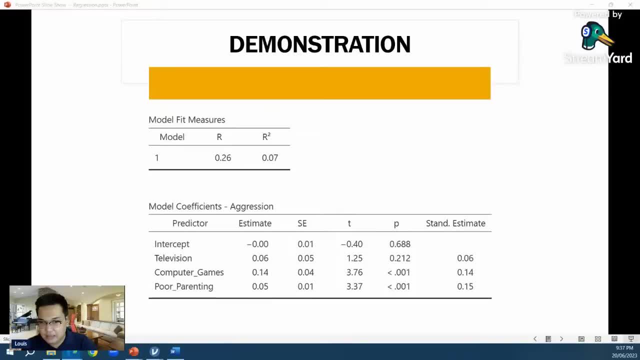 .14.. Meaning, the more you play computer games, according to this study, the more you become aggressive, And the same can be said for poor parenting. Significant din siya, Pero among the three, siya yung may pinakamalaking. 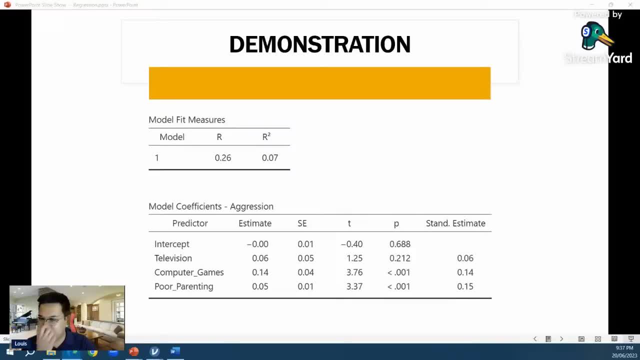 standardize estimate. May tanong kanina, Sir, ba't mas paganda yung standardized estimate? kesa estimate? Kung babalikan natin yung basics ng psych assessment, Hindi kasi lahat ng test on a scale of 1 to 5. Merong 1 to 7,. 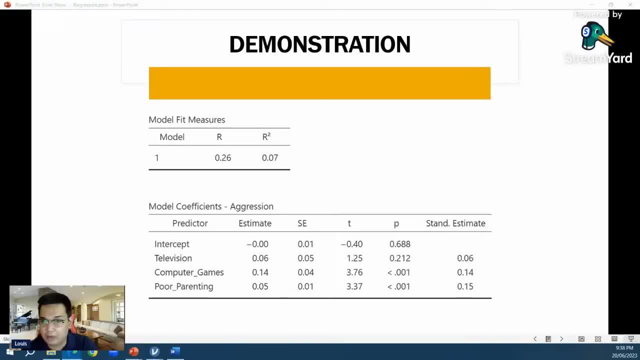 merong 1 to 10, merong 1 to 3, 4, merong 1 to 5.. Kaya natin mas sinusunod yung standardized Kasi, ginagawa niyang same yung scoring system. 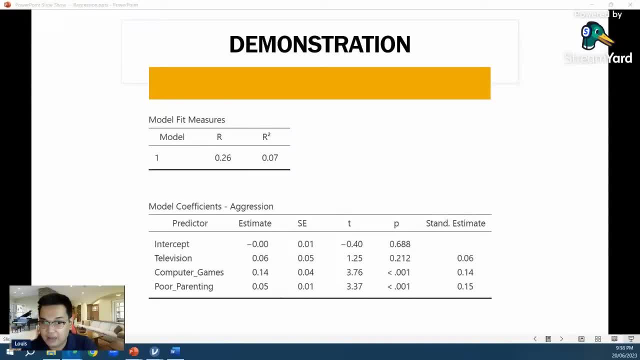 ng lahat, Ini-standardize niya. Kung titingnan natin, tingnan yung estimate, yung estimate lang, Kung ito yung basihan natin, mas malaking effect ng computer games than poor parenting ang liit. 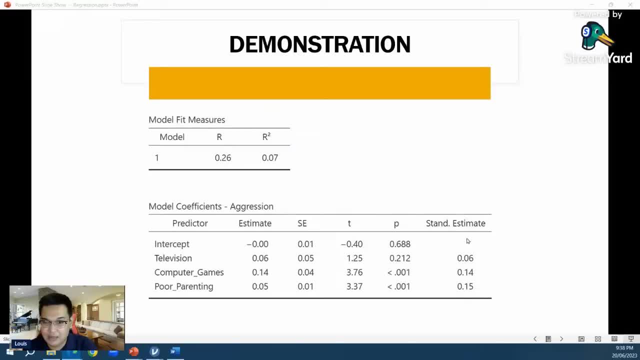 Pero sa standardized estimate, which is C-score, dito lumabas na mas malaking effect ng poor parenting kesa computer gaming. This is a more accurate result than the unstandardized one. Kaya ito yung itinitingnan. 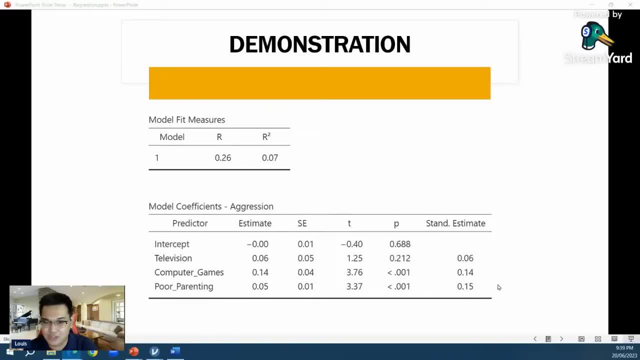 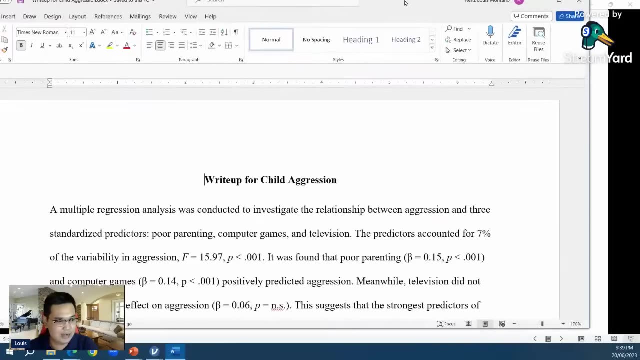 And between the two, poor parenting has a larger effect on aggression than computer gaming. So to end this part after netto, gusto niyo pa na isa pang sample, But to end this part, this is how you report, this is how you make. 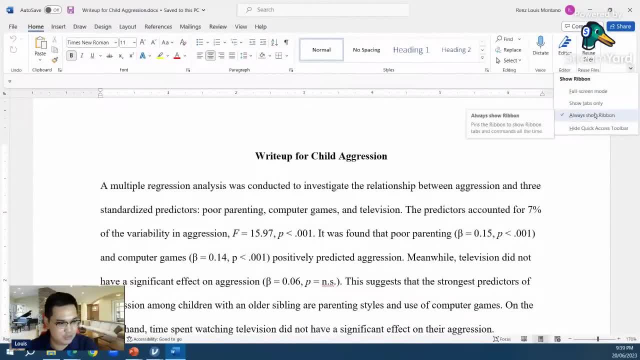 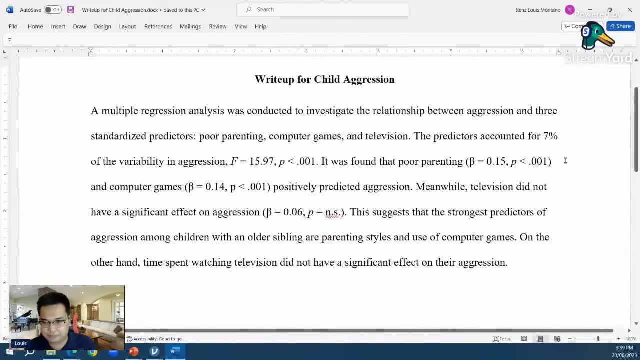 sense of the results. This is for my students. I borrowed their write-up for tonight's, for tonight's live stream: Sabi nila mga stat students. A multiple regression analysis was conducted to investigate the relationship between aggression and three standardized predictors. Bakit may? 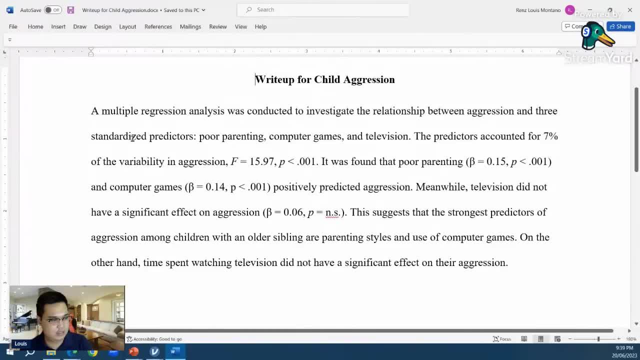 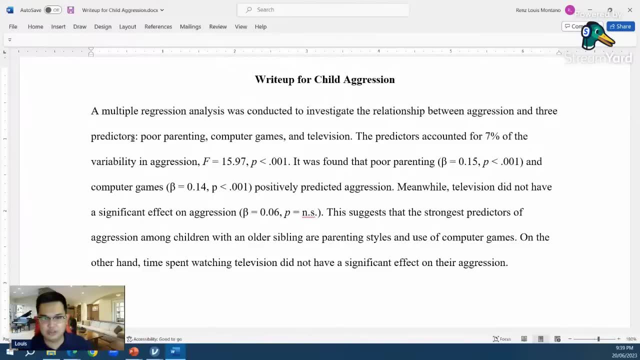 standardized Sige. i-correct natin yung result nila Hindi siya. I don't think it should be Predicters. that would be enough. Poor parenting, computer games and television. The predictors accounted for 7% of the variability. 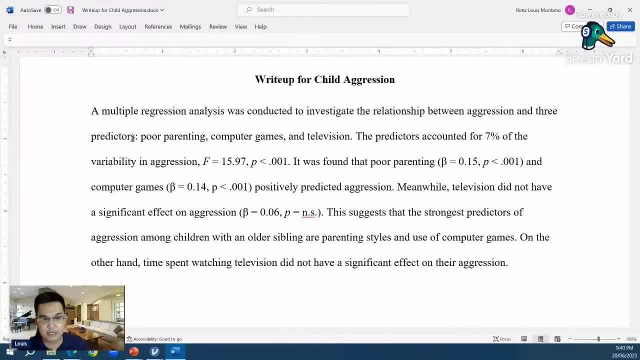 in aggression. Tama yan. Based dun sa result kanina Nilagay nila yung model. fit Significant yung model. It was found that poor parenting and computer games positively predicted aggression. Meanwhile television watching, hindi naman television. 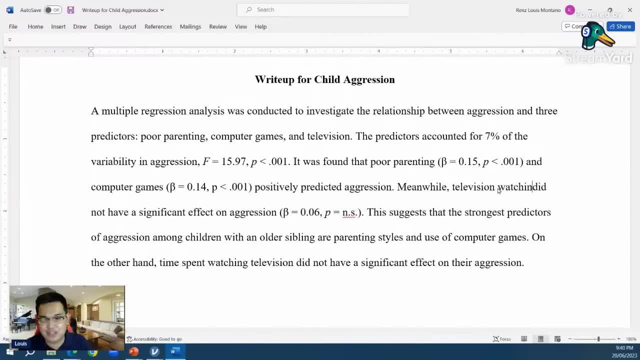 Ano yung TV mismo, Television watching naman. Television watching did not have a significant effect on aggression, Kasi maliit yung beta niya, Pangalawa yung p-value niya 0.212.. Tama ba pagkaalala ko: 0.212. 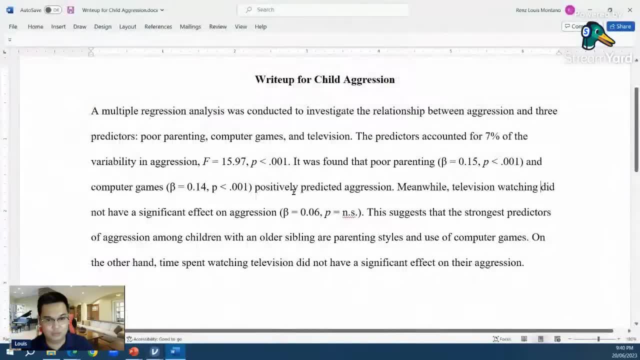 ba yun? Yes, 0.212.. Napaka-liit, Ito yung interpretation nila. This suggests that the strongest predictors of aggression among children- kasi yung study nato may- with an older sibling, mga bunso. 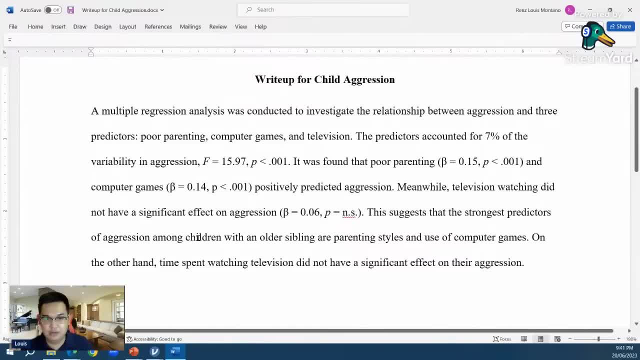 or mga younger siblings. The strongest predictors of aggression among children with an older sibling are parenting styles and the use of computer games. So yung may effect daw sa aggression ng bata yung parenting tsaka yung gaming On the other. 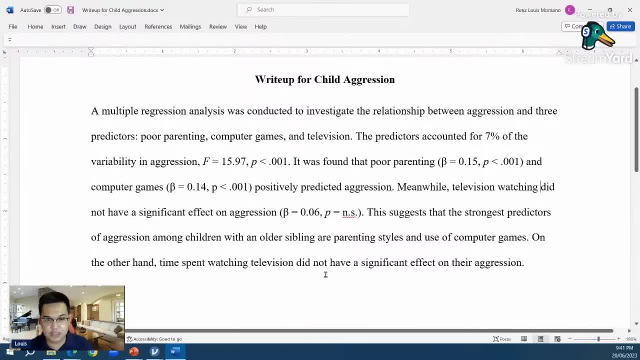 hand, time spent watching television did not have a significant effect on aggression. So that was their conclusion, And I do agree with that. Based on the data, yun yung naging outcome. Okay, Yes, po, isa pa daw. 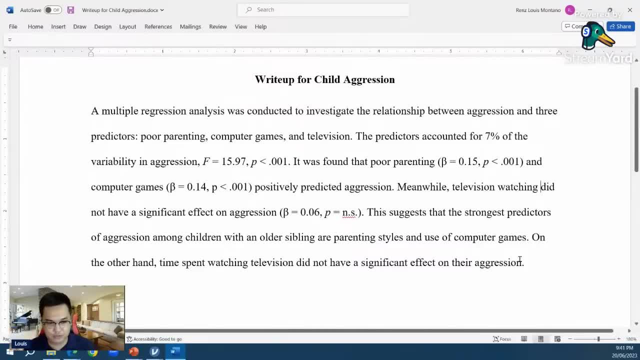 After neto mag-words of wisdom na tayo para sa board, as you requested. Tanong, ano yung mga gusto niyo i-cover ko Before the last example. what do you want me to cover in the next livestream? Hanap ulit ako ng another. 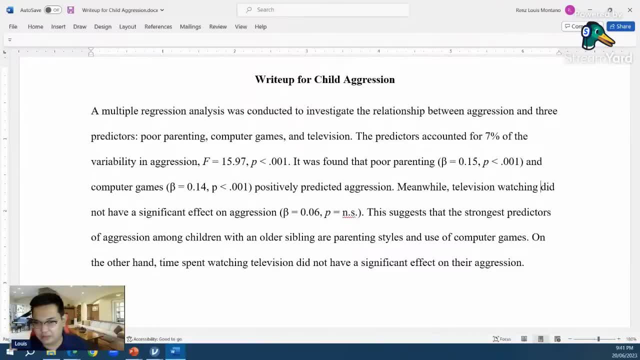 opportunity. Ano yung mga gusto niyong ano natin. no, I-cover natin. I-comment niyo lang. Titignan ko kung kaya ng powers ko. As long as kaya ng powers ko, i-cover ko. 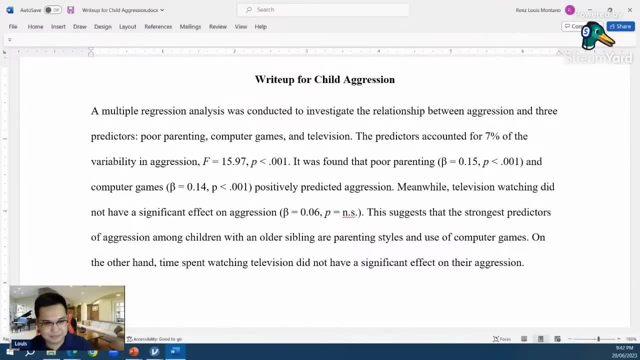 yan, Pero itutuloy natin yun na yung statistics and test development. Ipe-prepare ko lang yung, ano, yung material ko doon. Okay, Sige another example: no, While waiting for your responses. 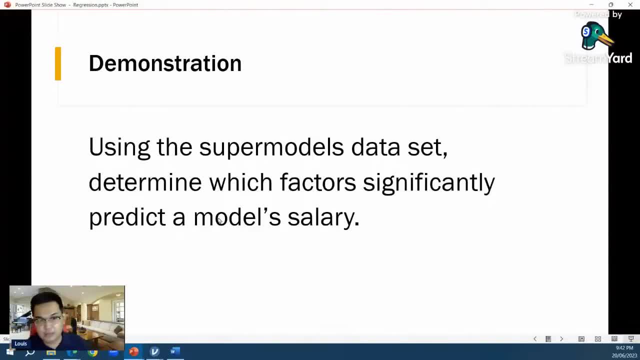 Using the supermodels dataset, determine which factor significantly predicts a model's salary. Okay Yan Sige, Tingnan natin to No Okay. So this is another study from the textbook of Andy Field about supermodels. Yung mga catwalk. 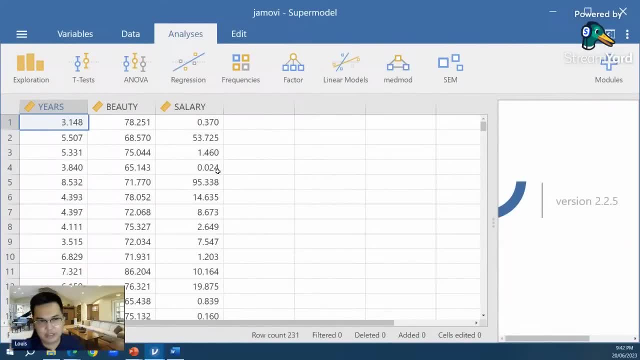 models And ano yung predictor ng salary nila, Whether malaki yung bayad sa kanila or maliit lang. And the two variables they have taken into account are years of modeling. Kompletuhin natin na Years. 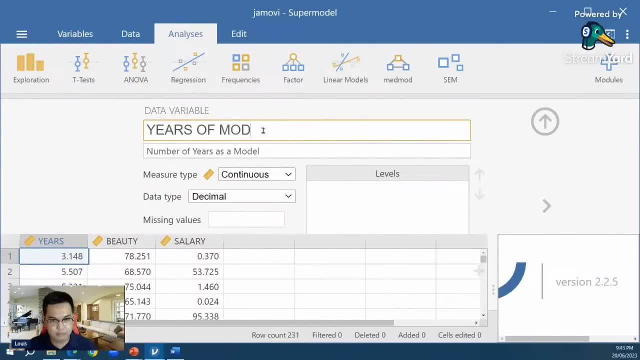 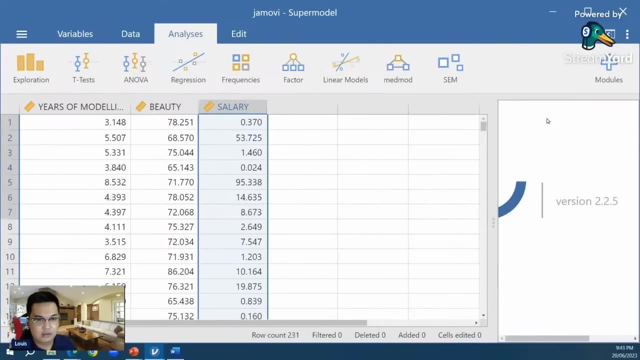 of modeling and beauty. No, How you define it traditionally, yun yun The beauty of the model And the outcome variable is their salary. What do you think between the two will be? Ano kaya yung may effect sa salary? 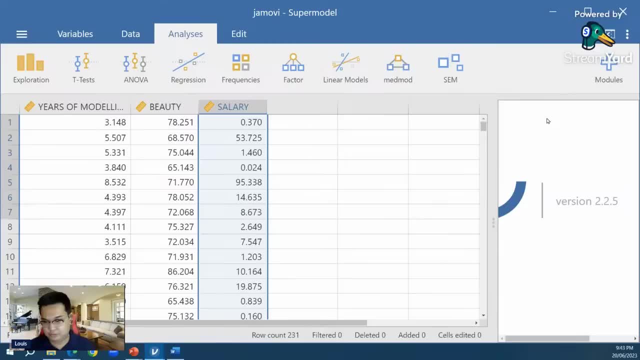 Years of modeling beauty or both. Ayan Parametric, non-parametric, Sige, May material ako dyan Ready na, actually Ready na nga. ba Hindi yun ganun ka-technical, Pero wala akong demo doon. 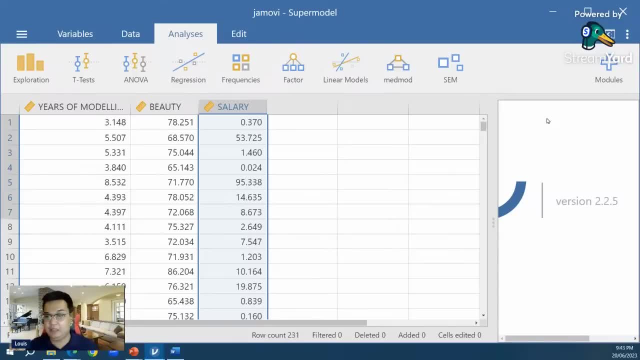 Wala akong demo doon, Pero dadaanan lang natin yung iba't iba't mga treatment. Pero hindi ako magde-demo, Kasi baka abutin tayo ng limang oras. Pero will that help na ba? Okay na ba yun? 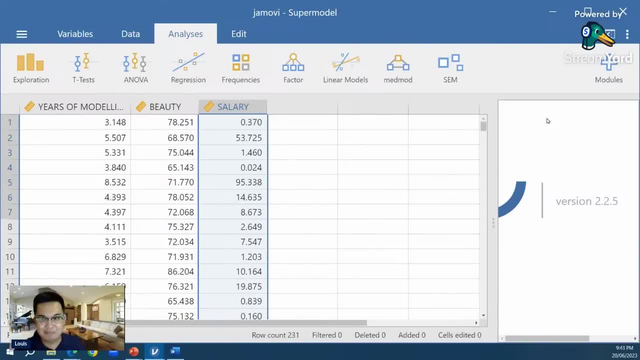 Sabihin ko lang kailan yung gagamitin. Pero wala mo ng demo, We can do that on a separate occasion. Okay, Ako pinlano ko na t-test, Tapos another occasion. ano ba naman? 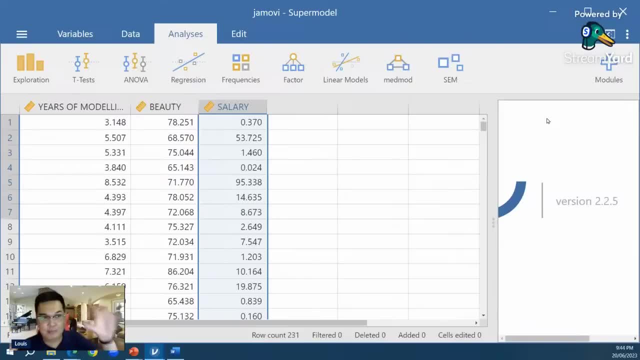 Pero ang gagawin ko this time? ano lang muna, ano yung pipiliin mo. if this is the situation, Okay Ayan. Pero going back, sabi na yung beauty daw na yung may effect. Okay, Sige, i-run na natin. 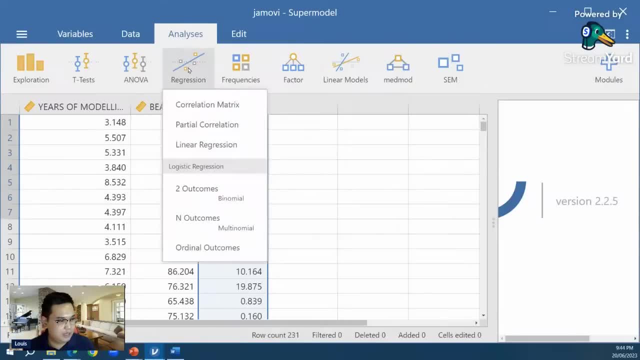 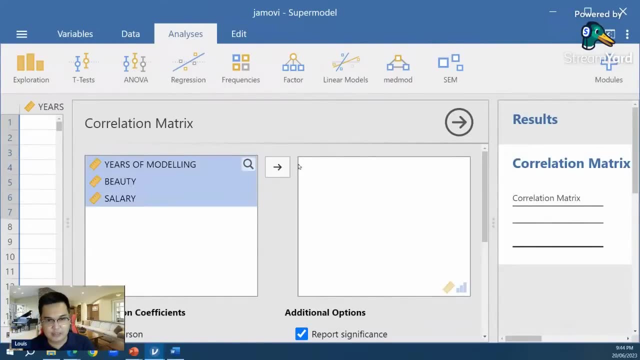 No. So tingnan natin ano ba talaga I-correlate muna natin. And para masanay kayo lahat ng variables natin, isalpak na natin sa correlation, Para matuto kayo mag-interpret ng matrix. 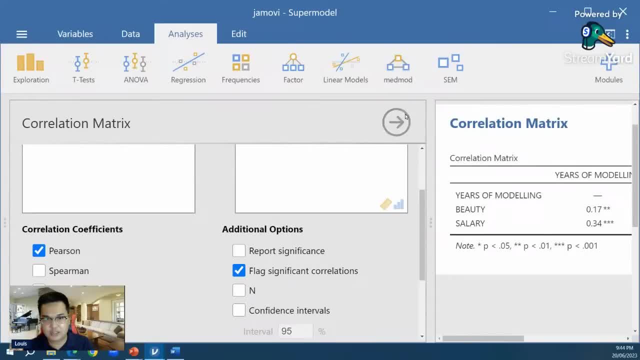 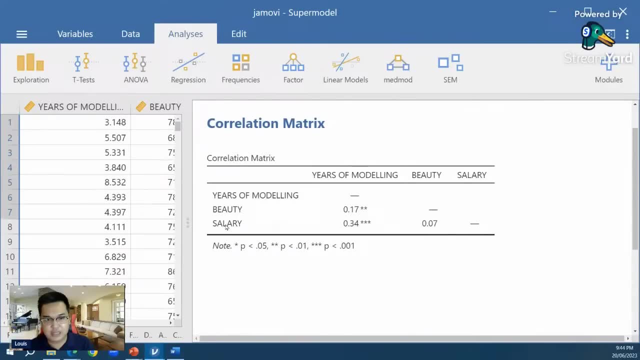 Okay, Tingnan natin yung correlation matrix Yung correlation ng beauty ay salary, no Salary yung variable natin. So yung nasa pinaka last column, Beauty and years of modeling are significantly related. kasi may asterisk, 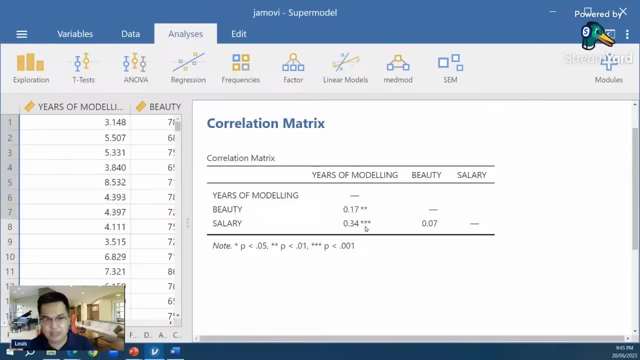 .34, Meaning the more that the longer you are in your modeling career experience, the higher your salary. Pero si beauty walang effect sa correlation And somehow that tells us na sa regression parang ganyan din yung ending. 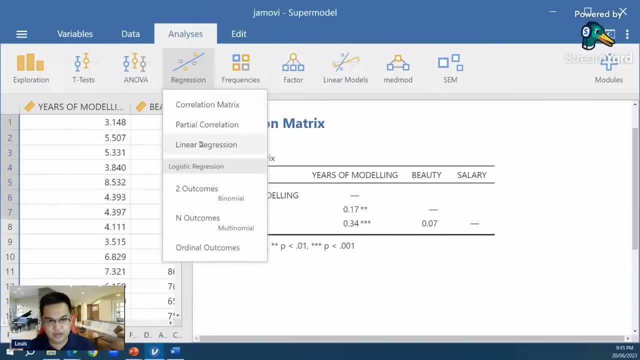 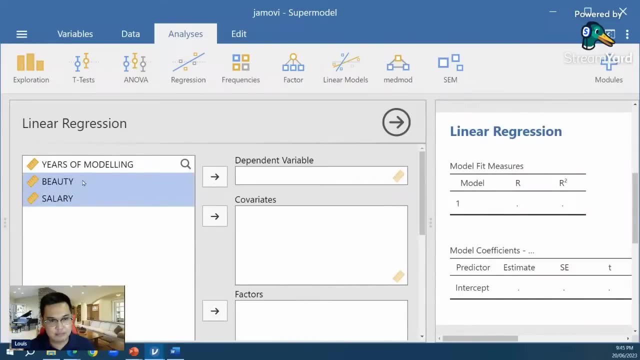 So i-check natin, Let's do regression, Okay. Beauties and modeling- sorry Beauty and years of modeling and beauty are the corporeal And salary is the DV. Gusto kong makita yung model test. 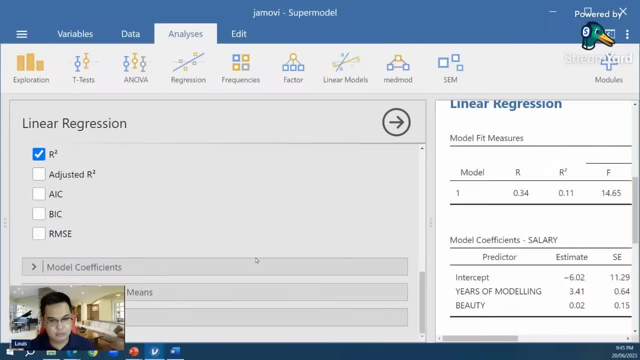 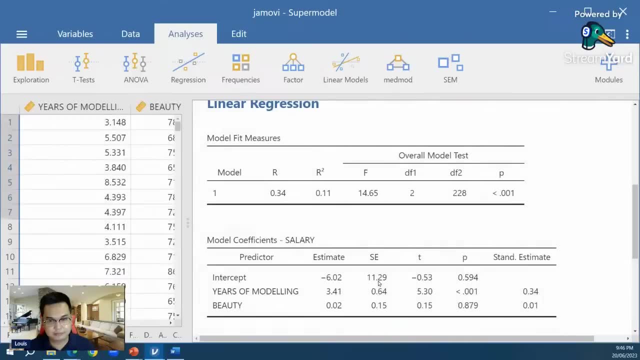 And gusto kong makita yung model coefficients na standardized. And there you go. Isa lang na natin yan. Ito siya R squared .11.. Okay na yan. P value less than .001.. Significant, So meaning kapag tumingin ka sa baba. 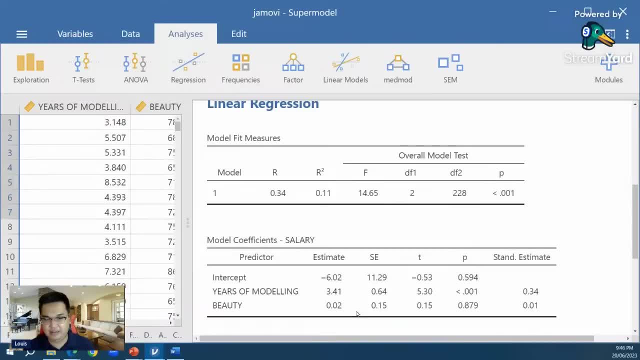 isa sa mga yan may effect. Okay, Just like in correlation, if you look at years of modeling, if you look at its P value- less than .001, standardized estimate is positive .34.. Meaning, the more that you spend years in modeling, the higher. 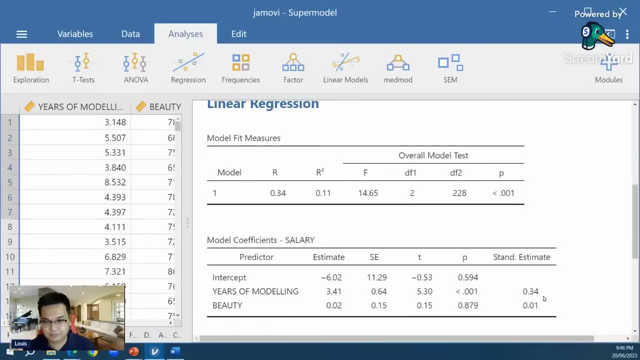 your salary is going to be. Pero sa beauty, look at the P value .879.. Mas mataas siya than .05.. Meaning, wala siya talagang effect. Is it surprising Ako? na-surprise ako. 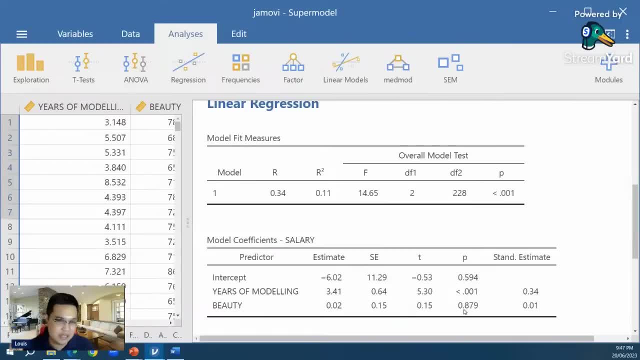 Okay, Maybe sa research lang na to. I don't know kung ba't ganun yung finding nila, pero basically this tells us that what matters more in their participants in their research is the experience of the model rather than their beauty. 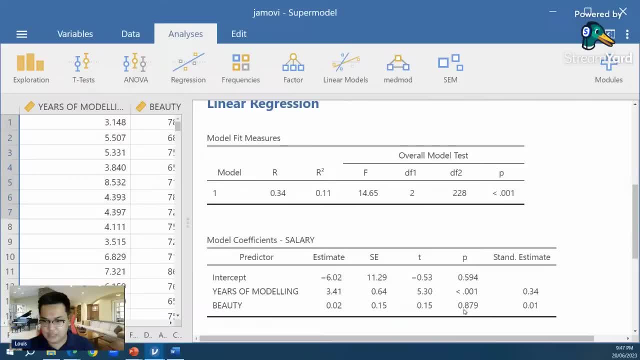 Nakakagulat. Okay, I don't know, this is absolute. I don't say that this is absolutely correct at all times. Maybe sa sample lang nila. I don't know if other studies would have the same finding, But let's. 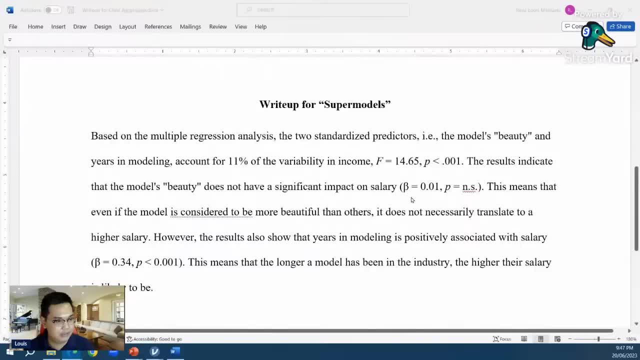 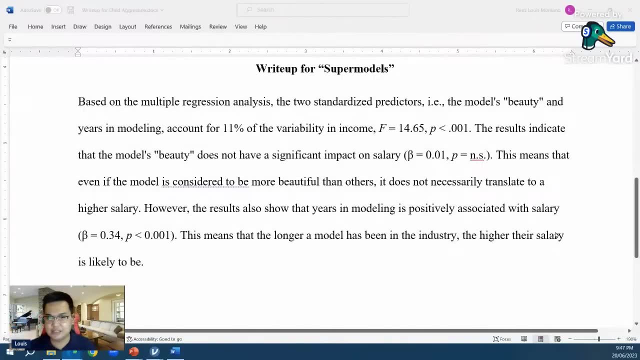 report the results as we end the session. Ito sabi ng students ko. Based on the multiple regression analysis, the two predictors are: the model's beauty and years of modeling accounts for 11% of the variability in income or salary. The results indicate: 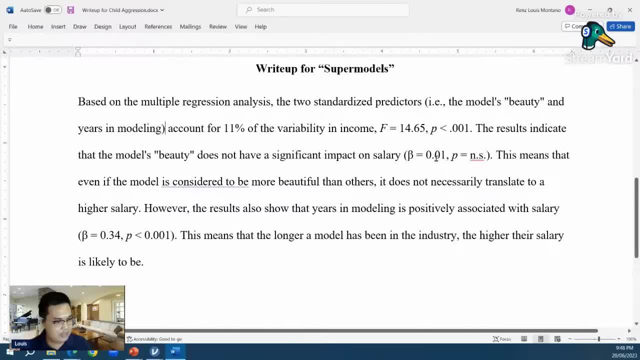 that the model's beauty does not have a significant impact on salary. This is the beta. .01 nga ba Tama .01.. P is not significant. This means that even if the model is considered to be more beautiful than others, 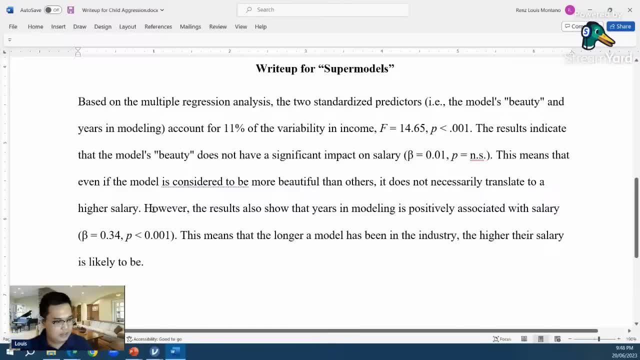 it does not necessarily translate to a higher salary. However, the results also shows that years in modeling is positively associated with salary. This means that the longer a model has been in the industry, the higher their salary is likely to be Okay Yan. 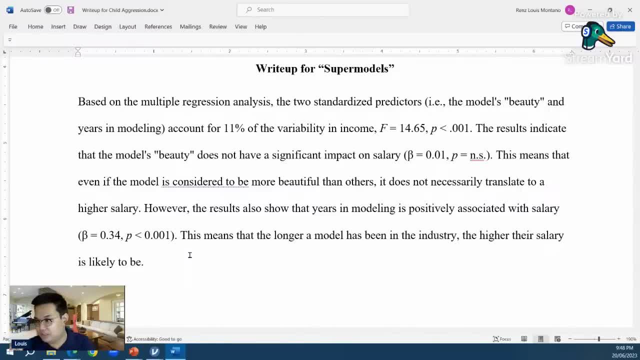 Kasi madalas akala natin yung subjective beauty ng tao is totally the end. Alam natin iba kung manunood ka ng Miss Universe, iba may mga races din. What is beautiful for an Asian may not be beautiful for an American. 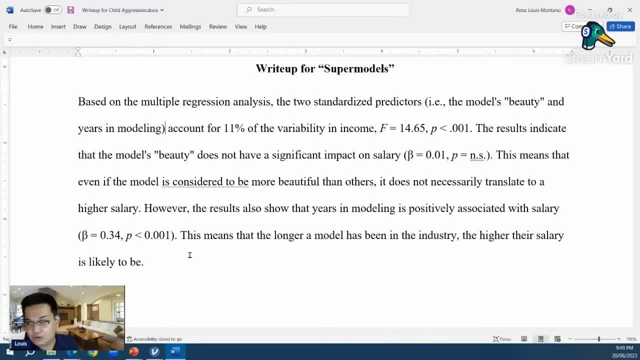 for a European, for an African, Yun Yun, yung isang magandang explanation doon. So it's not the subjective rating of the beauty of the person. Maybe that's a big factor. Do you agree with that? I don't know if you agree, no, Pero that's one way. 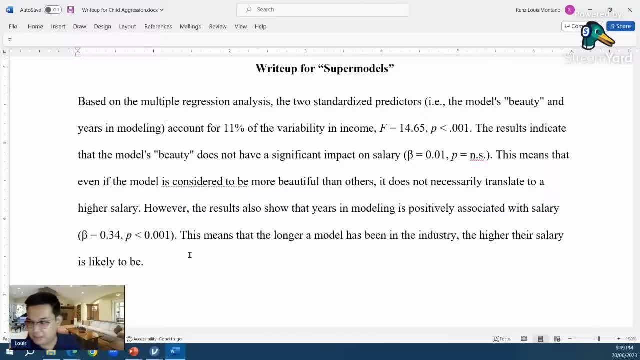 to look at it Yan. Pati sa ano diba Kunyari may racist comment ka. Ano ba yan. Ano naman, Ba't ganito yung skin color niya, Ba't ganyan yung mata, Ba't ganyan yung itsura. 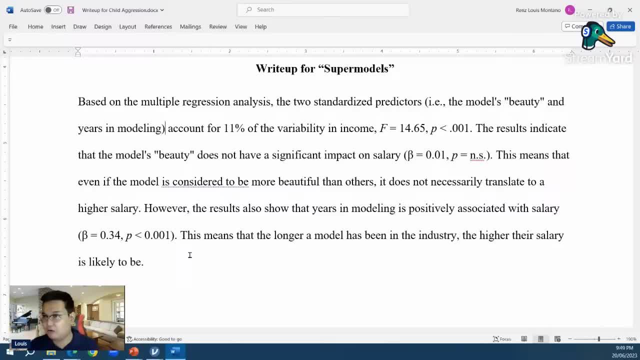 Ba't ganito, ganyan yung shape ng katawan. Pero maugulat ka, Yan yung champion Or yung Miss Universe Yan Alright, Sige. Questions about the regression analysis. Okay, Tama yan no. 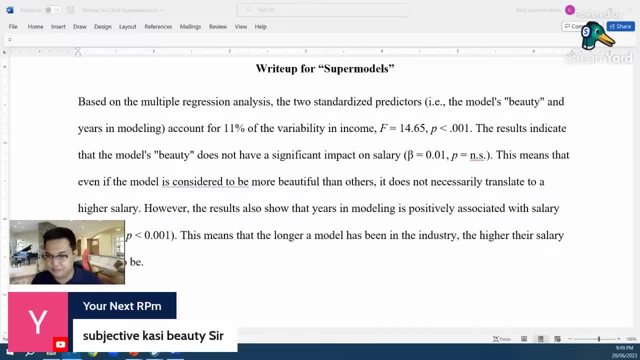 Subjective, kasi ang ratings ng beauty Yan Questions or clarifications. Anong mas gusto niyo unayin natin next time? Is it the statistical treatment or statistics and test development? Stat treatments: Okay Sa hierarchical, mas advance na yun Sa hierarchical. 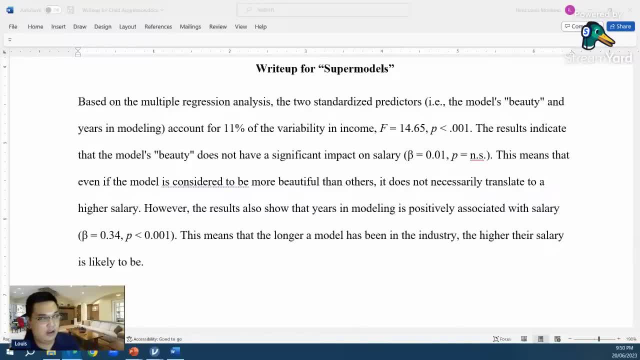 iniisa-isa mo siya May study kaming lalabas soon Hierarchical regression Sa multiple. kasi sinalpak mo lahat Sa hierarchical, isa-isa mo siyang iinsert Masyado na yung advance. 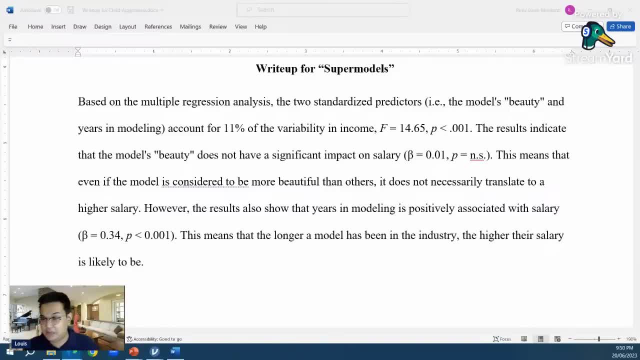 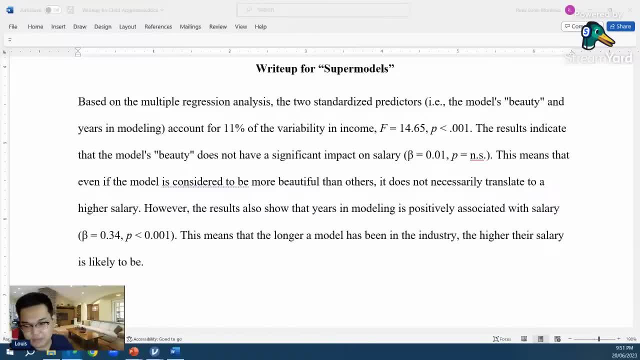 ginawa siyang z-score. Okay, Parang ginawa siyang z-score instead na raw score, Kaya mas makakapag- make ka ng comparisons between the variables. Saan po dapat mas mag-focus, Oh, cohen gamit ko. 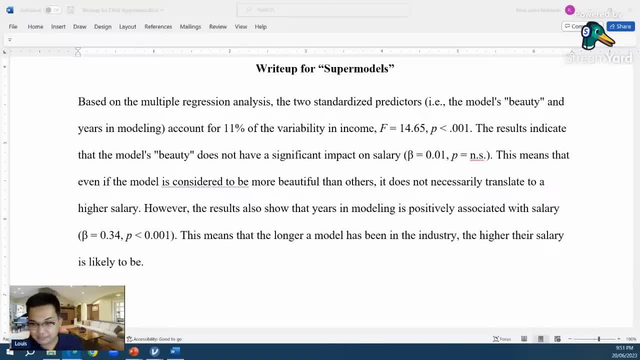 Okay, Cohen, yung ginamit ko nung nag-aaral ako. Okay, Sige, may lecture ako about test development. Hanap tayo ng day no Medyo busy ako this week. Bukas may presentation, kasi kami sa ano eh. 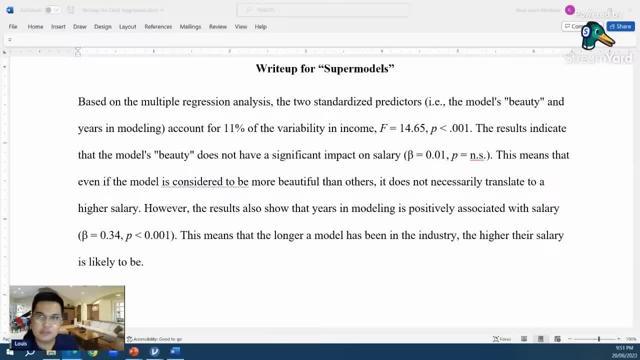 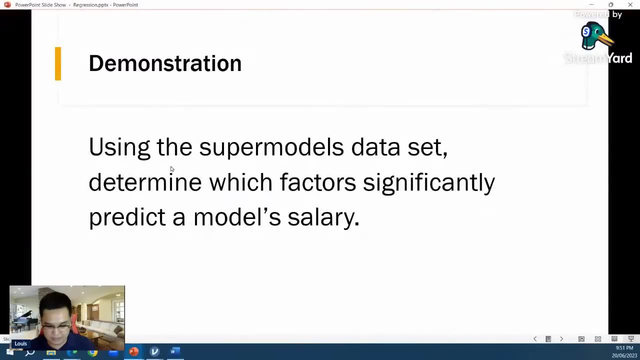 ng research namin. Tapos saan Ang dami namin mga presentation? no Yan Okay Sige. no Ayan Okay Sige. Before we end, let me just invite everybody that, if you're considering no. 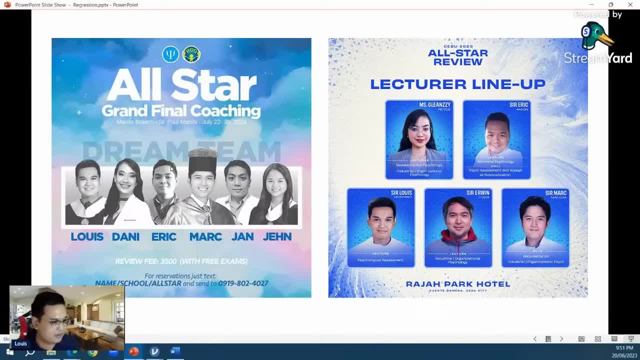 mag-All-Star, I'll be in the All-Star review. if you're considering joining the All-Star review, I think magkikita kita tayo sa Manila branch Okay, And also sa Cebu branch, no, So you can. 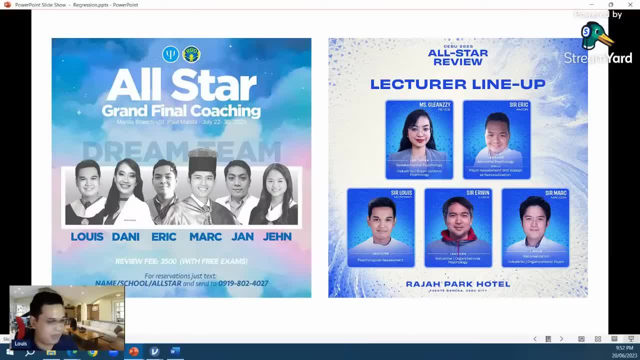 contact the respective branches if you would like to join Meron pang All-Star sa ibang mga lugar. no, And you can contact the branches offering All-Star review. Okay, Pero yeah, I think makikita ko ang mga future RPMs. 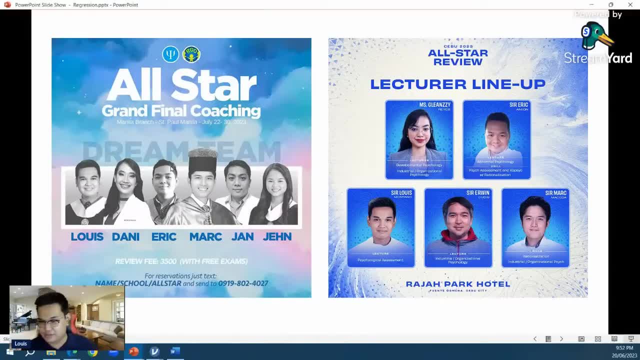 ng Manila branch, for the All-Star, and also for also for the Cebu branch. So ayan in-advertise ko lang. So okay, Makikita kita tayo soon again face-to-face. Wala po ba sa standard. 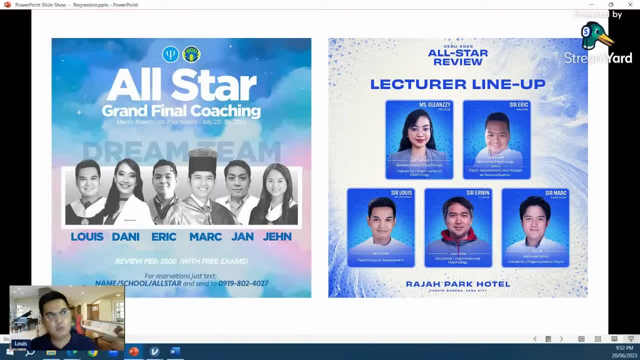 estimate na strength kung sino, Unlike correlation, wala siyang strict interpretation na ito. yung small, medium, large, weak, moderate, strong, Wala siyang ganun Okay. Words of motivation daw for the board exam. 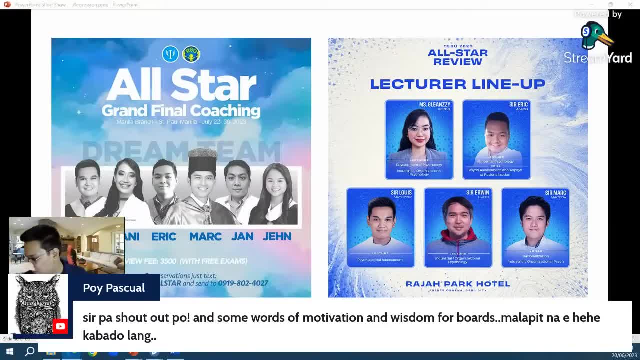 This is not my line. no, Nakuha ko to kay Sir Jojo. Okay, And I remember Sir Jojo once told us no one is 100% ready for the board exam. You just have to be ready to take it. 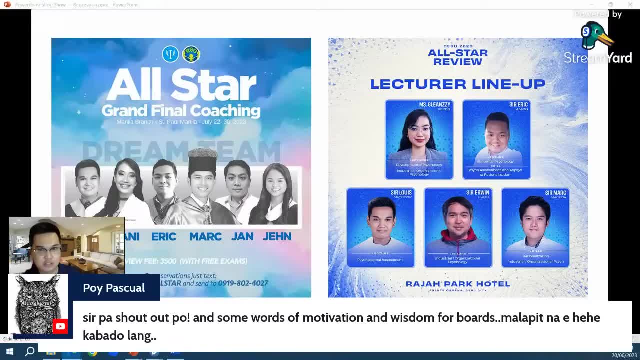 Okay Ako nung na-board exam, ako ang daming reason for me to think na hindi ako papasa, Like, alam ko, most of ang daming mga graduate this time, this batch with Latin honors. no, Ang daming natin mga. 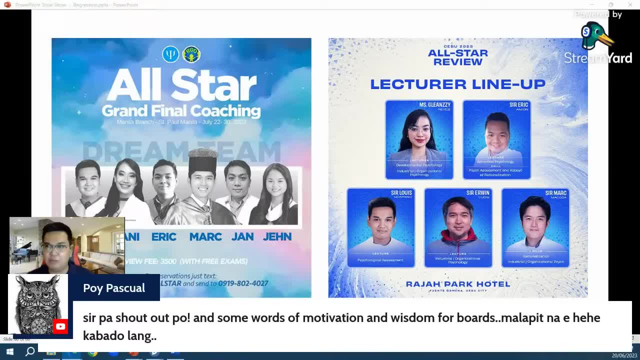 scholars. no Mga cum laude, manyong cum laude, suma cum laude. When I graduated, I was just a regular student. I did not graduate with honors. I'm like most of you na hindi graduate with honors, Pero kasi what kept. 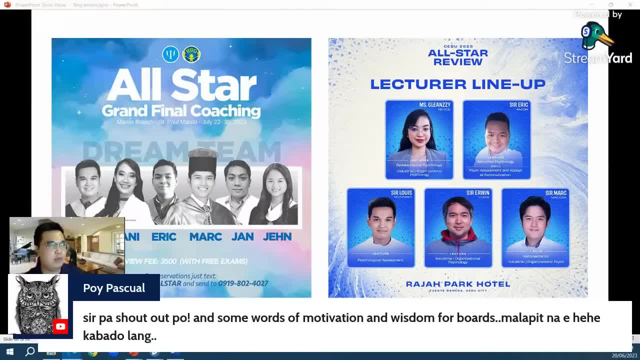 me going is that I really wanted to pass And I'm willing to do everything I can do okay During that time for me to pass. So I was not 100% ready, Kahit malapit na yung board exam. 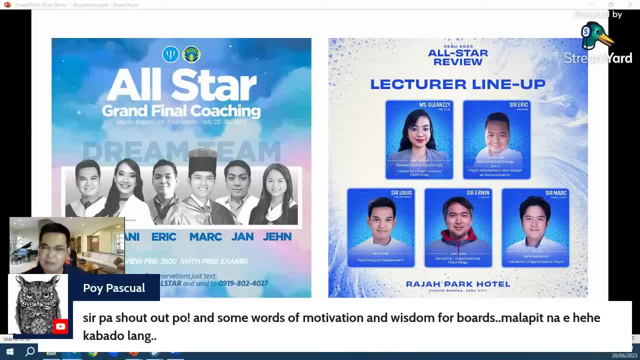 I still make silly mistakes in my drills. Ang daming kong mga mali. When I had my diagnostic exam 46 over 100 lang ako. Pero for me, the more mistakes I make, ibig sabihin more room for improvement for me. 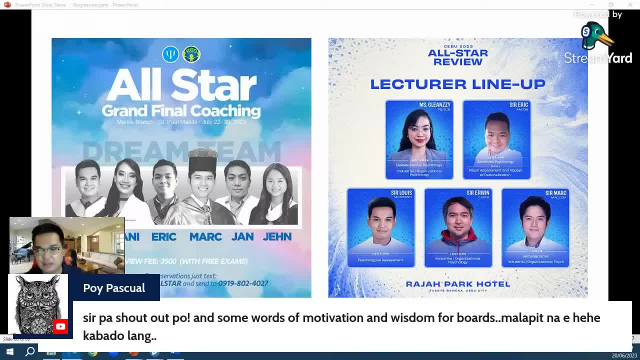 So I think if I was able to do it, definitely you can do it as well. Ayan Sige. So there you go, Sa Mindanao. I don't know kung meron na e-check mo lang yung mga branches. 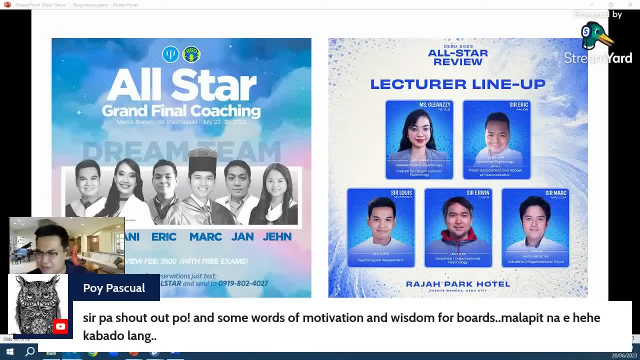 O saan ka ba ngayon? no, I don't know kung saan. no, Hindi kong memoryado kung saan yung mga may all-star na branches Ayan, Okay, And remember what predicts success in life. 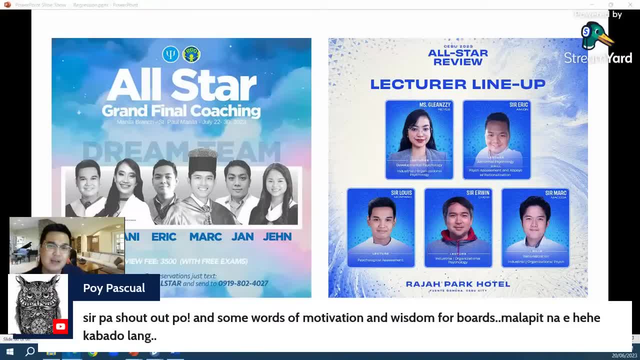 okay is not the person's IQ, but rather it's the grit, it's the academic resilience of the individual. I failed so many times as a student. I had lines of. I have mga line of sevens when I was studying I did not graduate. 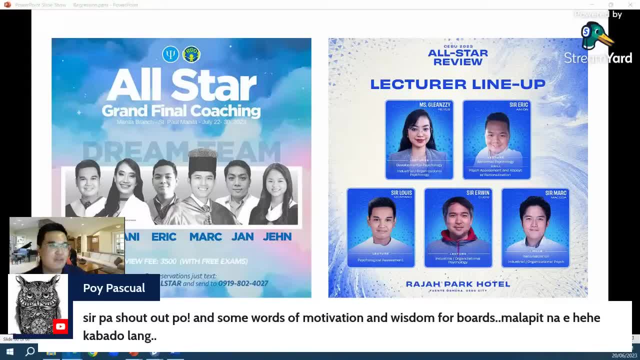 with honors. Pero pagdating sa review, kung yung review nag-e-start siya ng 8 o'clock, 7 o'clock pa lang, nandun ako, Nag-aaral, ako nagbabasa, ako, before the day starts. 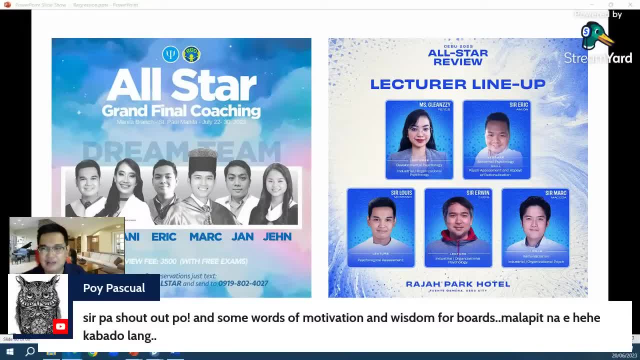 and when the day ends, nag-aaral pa rin ako. It's my consistency, it's my consensuousness that brought me here. So ayun, no, If I was able to do it, paano pa kaya kayo who graduated diba? 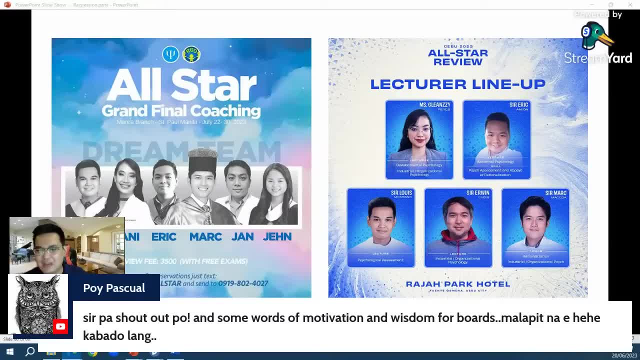 with cum laude, magna cum laude, summa cum laude. no, Mas matatalino pa kayo sakin, mas magagaling pa kayo sakin, because ako nga hindi ko narating yan Diba. So if I was able, 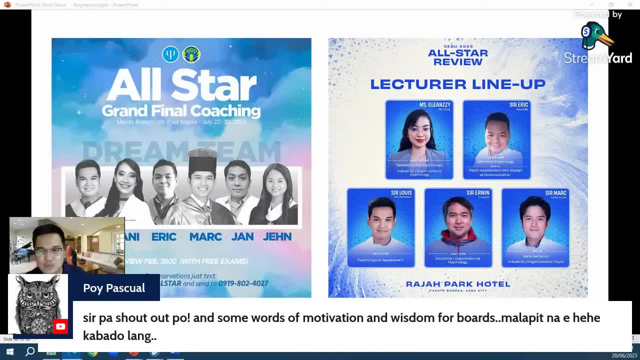 to do it, lalo na pati yung mga usual students, mga typical students. ako nga kinaya ko Kayo pa kaya Diba. Hindi ako magaling sa lahat ng hindi ako magaling sa isang, wala akong isang. 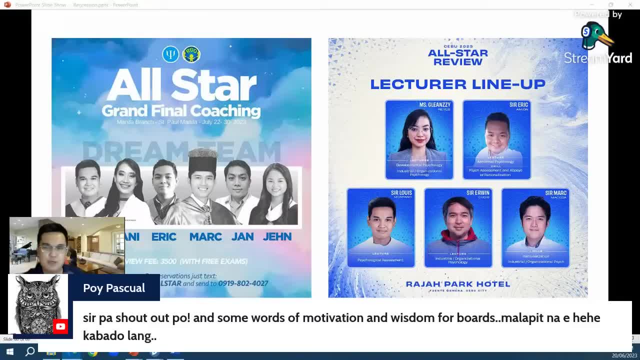 subject. Usually laging yung class may kumanta-taas ng score. may mga nakaka-96, kunyari Sa Abcite nakaka-95.. Sa IRO ganun Ako wala akong. 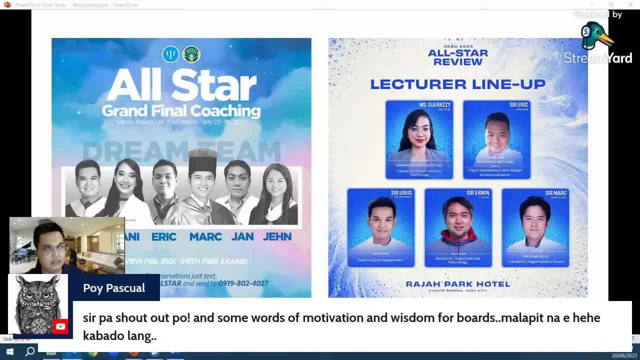 isang subject na magaling ako, Or ako yung laging top? Wala akong ganun, Pero yung secret ko is that sa lahat ng subject consistent ako. Okay, Yun yung secret ko. I may not be. 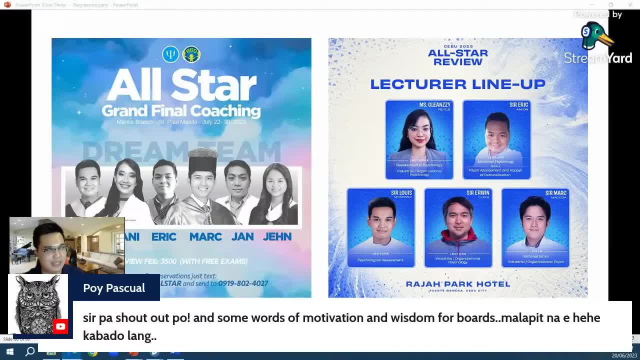 the best. I may not be the top the ace in a single subject, pero kung ano yung score ko sa isang subject dikit, dikit siya with my score in other subjects. Kumbaga, pinahalagaan ko lahat ng. 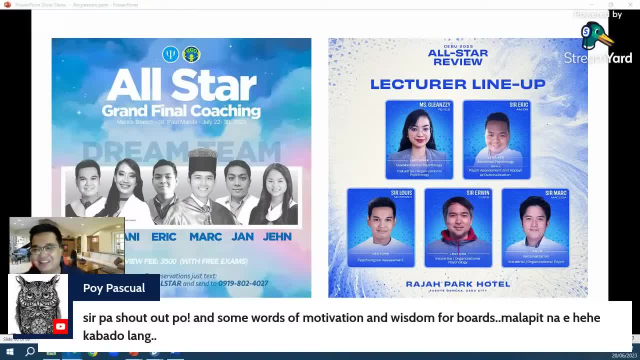 subject sa board exam. That's how I was able to do it. Yan, Just trust in yourself. Remember nando na. okay, nando na sa board exam paper, yung sagot Ahanapin mo lang siya. 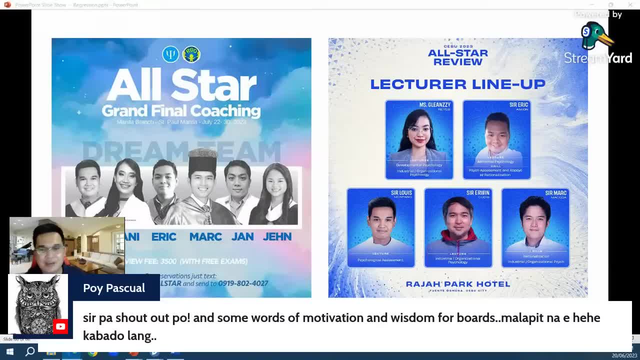 Yun yung tatandaan. niyo Nakasulat dun yung sagot. Kailangan niyo lang daw yung hanapin. It's not an essay test, It's a multiple choice test. Of course I'm not giving you false reassurances. 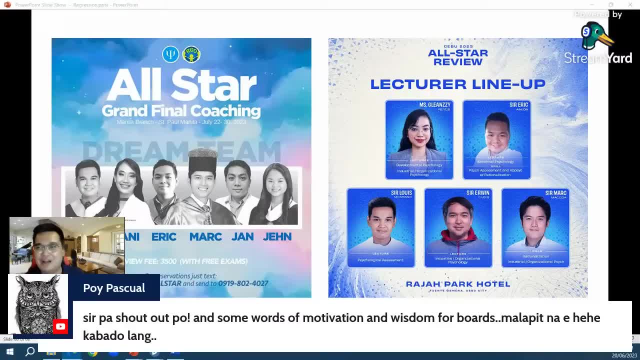 Pero if that will help you, di ba yun yung tandaan niyo. Okay. So there you go. Questions or clarifications. Anybody Alam ko magkikita-kita pa tayo ulit. no, Let's plan kung. 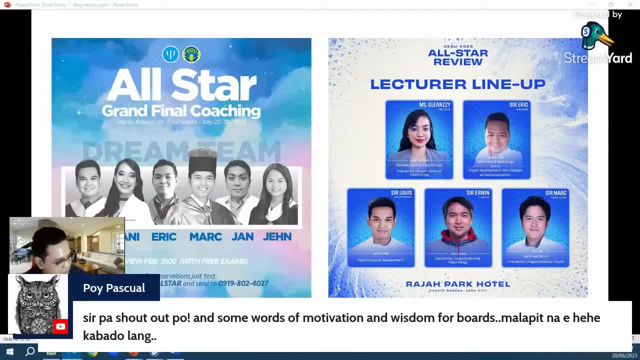 kailan tayo mag magkakaroon ng another session for the stack treatment- Ewan ko kung this week or baka next week na- And for the, Gusto ko kasi ituro yung test development. Okay, Gusto ko kasi maturo yung test.